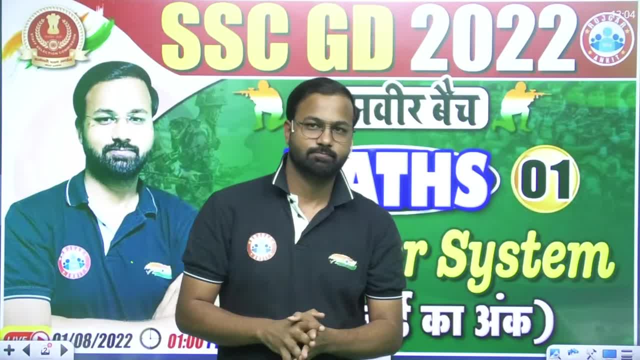 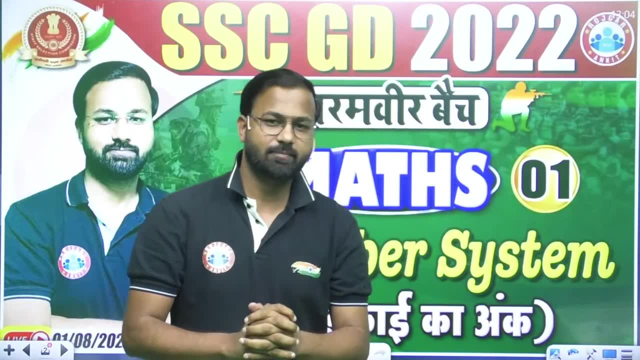 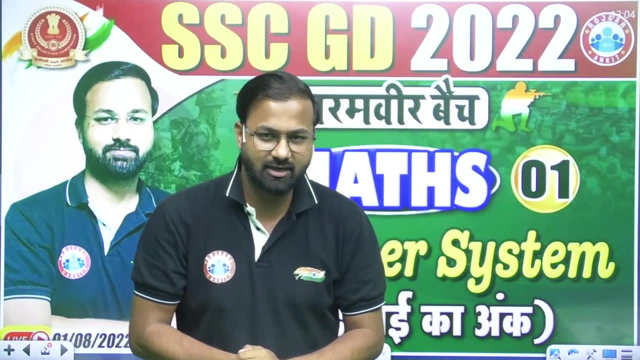 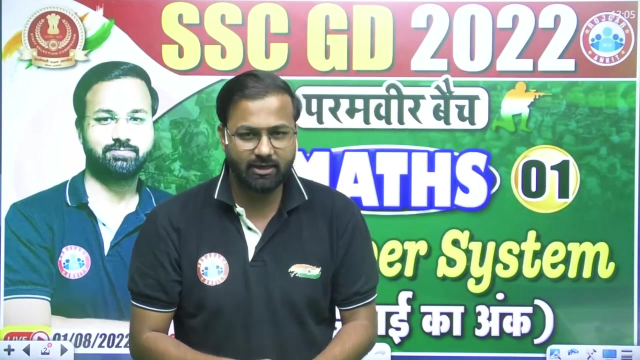 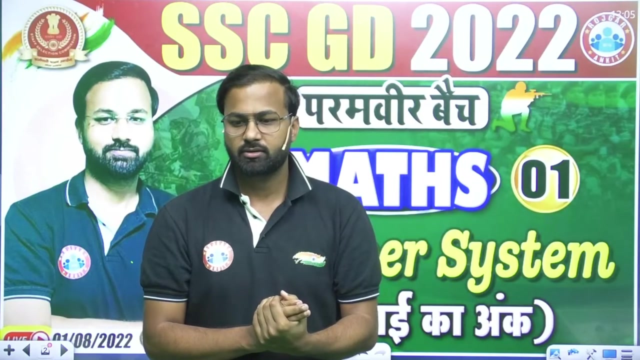 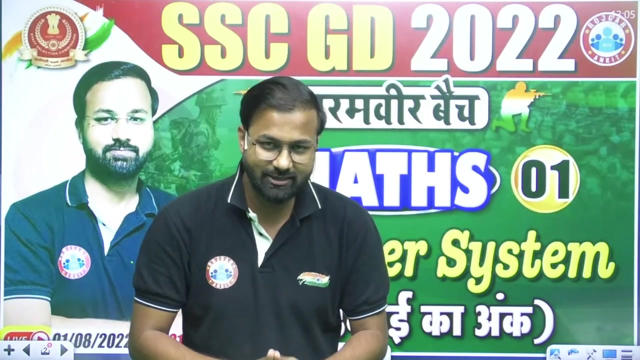 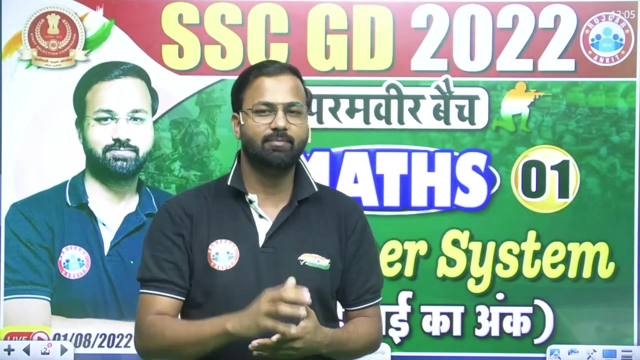 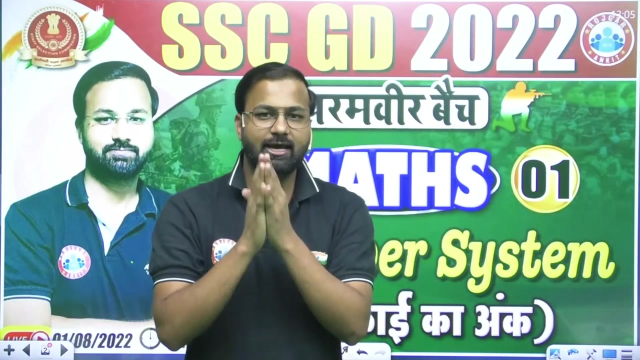 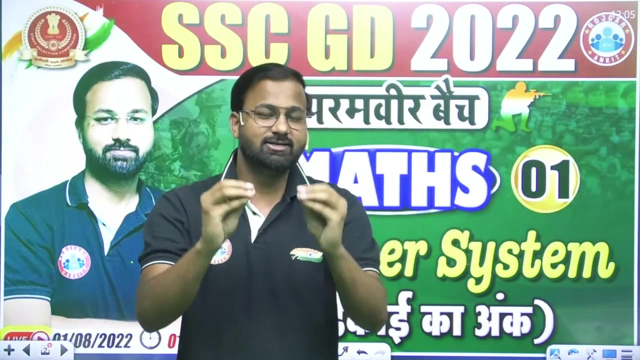 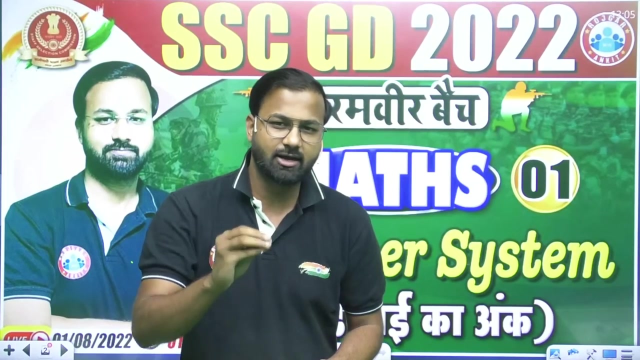 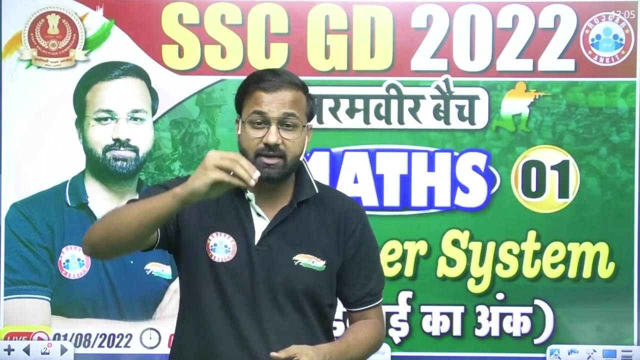 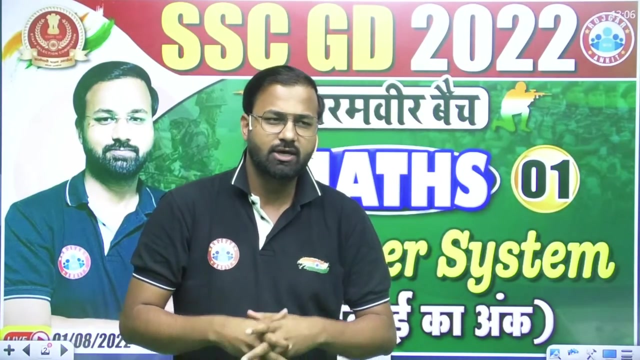 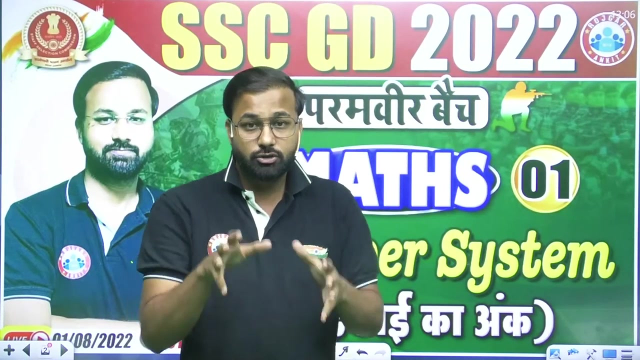 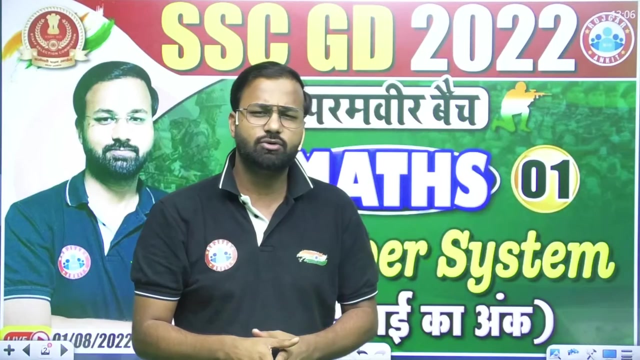 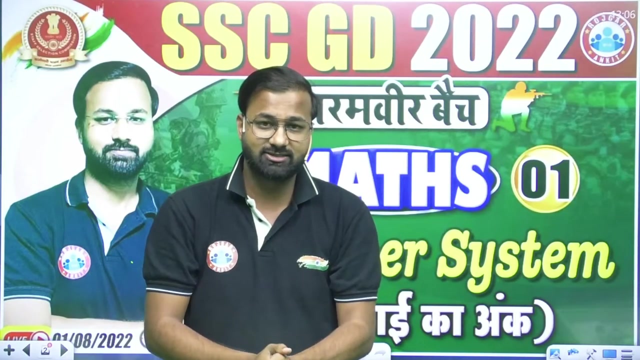 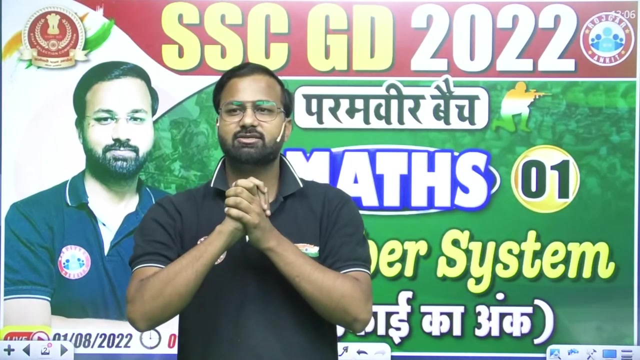 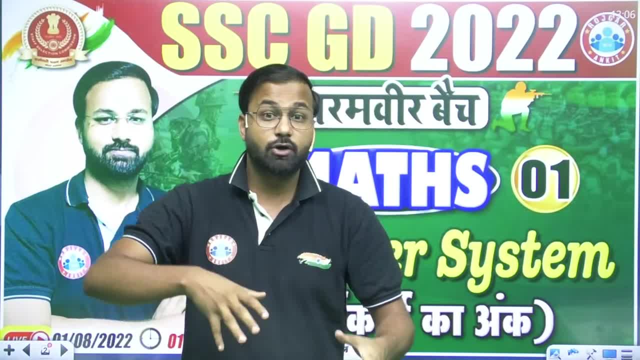 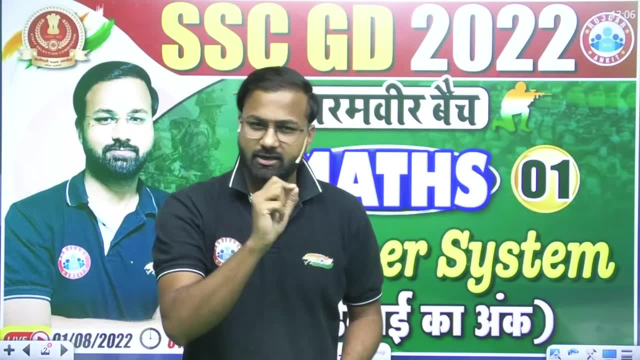 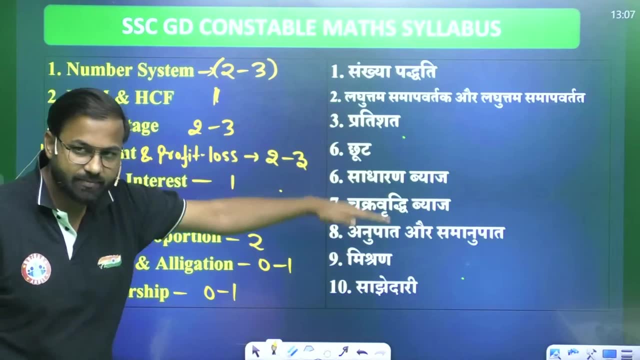 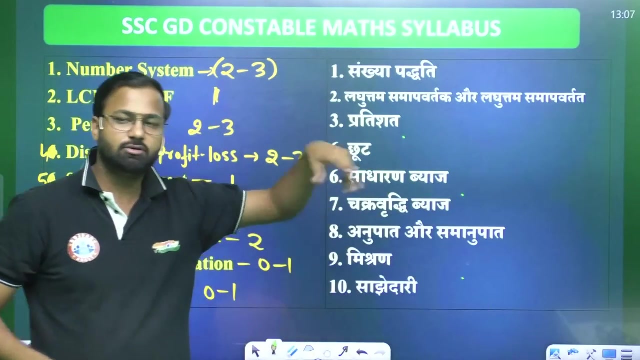 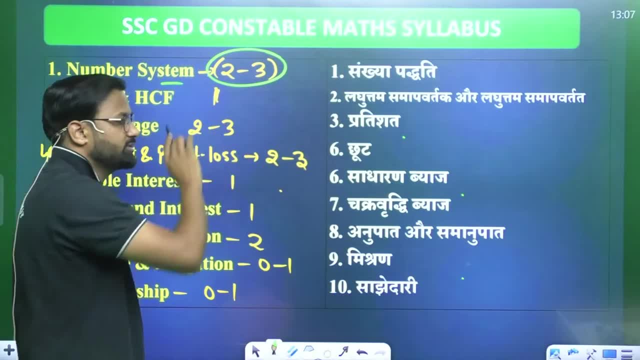 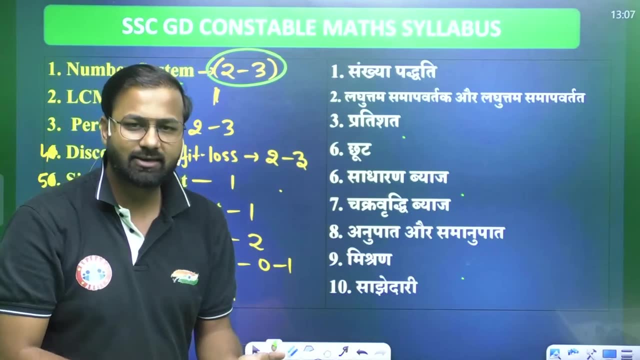 What I have made is that 2-3 questions have to be made in the number system And they will be made. 100% will be made. There are many chapters in the number system, Like as we started: Ikaikank. 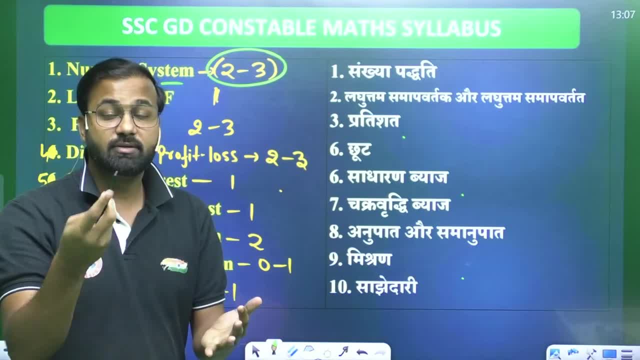 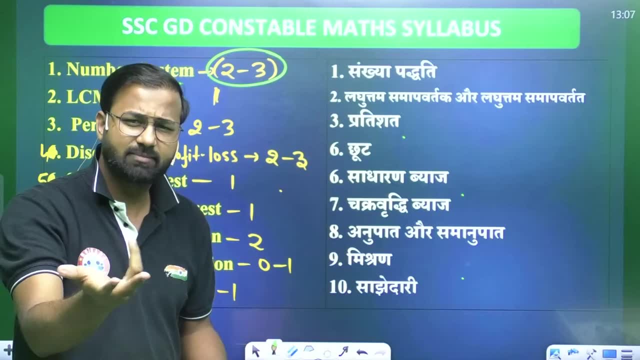 there is a chapter in Remainder Theorem Sesphalpari. the number of zeros is zero. there is a board mass in your number system itself. I will do your simplification and surds indices For Ghatankarni etc. 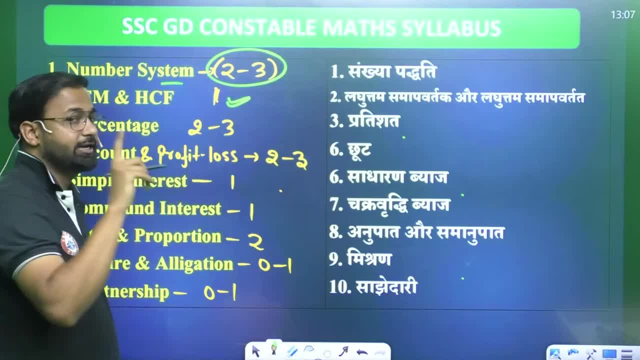 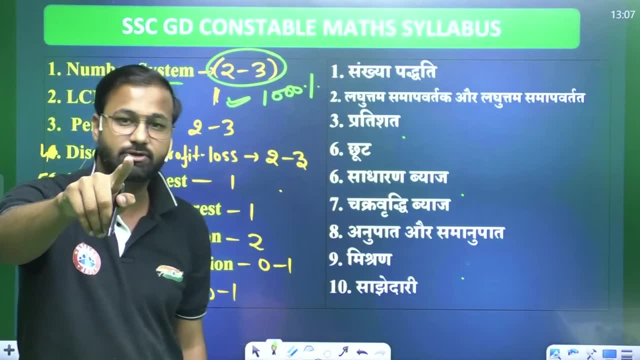 let's assume 2-3 questions In HCF-LCM. one question is 100%. I guarantee you not 100, I will put one more zero, 1000% will be made in HCF-LCM. So we have to divide each question in such a way that 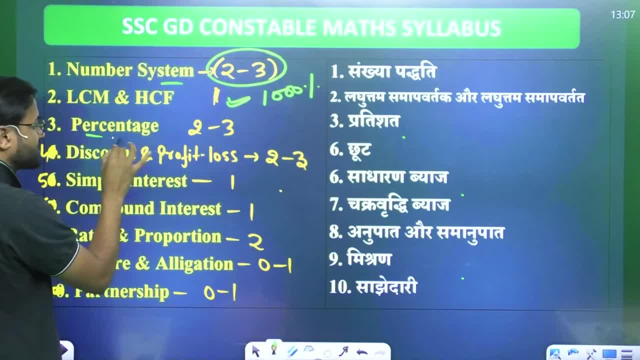 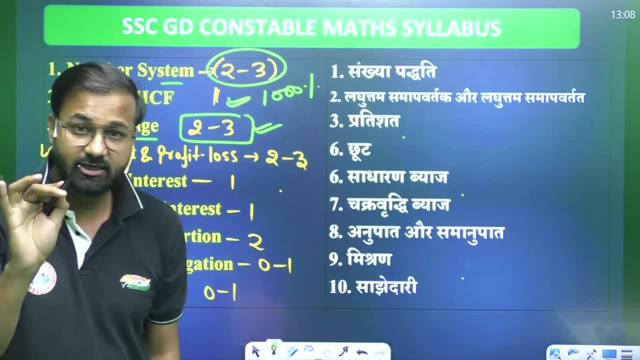 we will not let this question go at all. Secondly, if I talk about percentage chapter, then 2-3 questions will come in percentage chapter. Okay, If 2-3 questions will come in percentage chapter, then you have to be ready for percentage chapter. 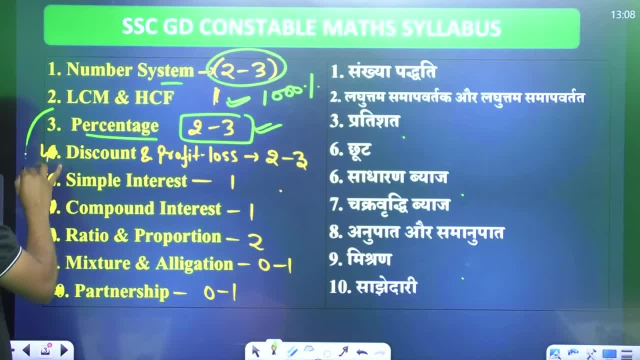 Because percentage chapter is the only one which will make these 4 chapters strong. 4 chapters till 6th chapter: Percentage, discount, profit loss, simple interest and compound interest. Yes, These 4 chapters will be clear from percentage. 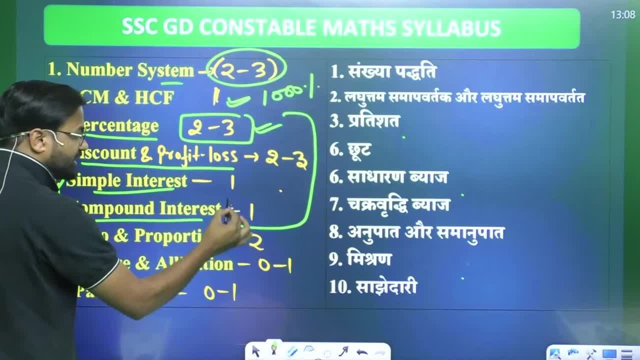 And now you see how much weightage you have taken in these 4 chapters: 2-3 questions in percentage, 2-3 questions in profit and loss, 1 question in account, 1 question 1000% from simple interest. 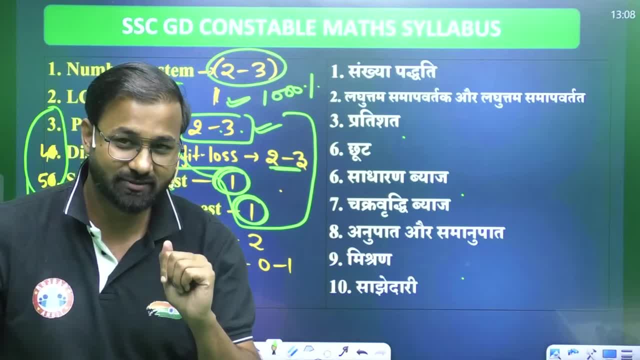 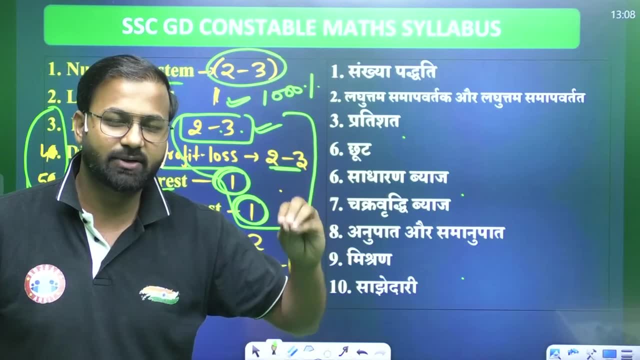 and 1 question: 1000% from compound interest, ie from HCF-LCM. And these 4 chapters are such that I will teach you percentage and the day I will teach you percentage, that day you will ask about HCF-LCM. 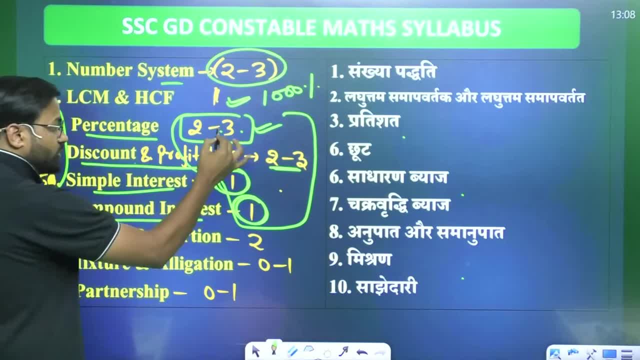 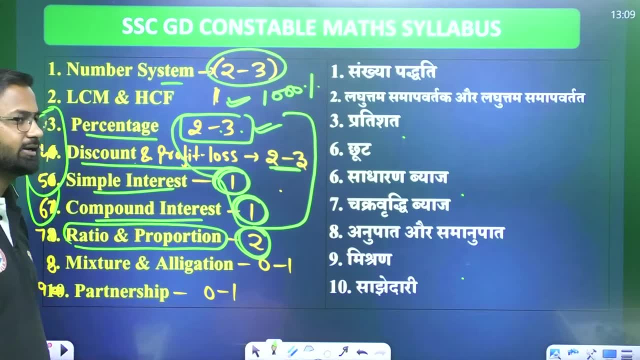 That day I will clear these 4 chapters from 1 concept. So this much question weightage is done. Then comes the question on ratio proportion. From ratio proportion: 2 questions have to come 100%. From ratio proportion: 2 questions have to come 100%. 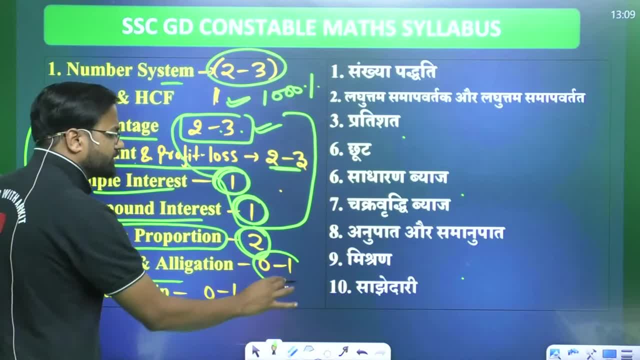 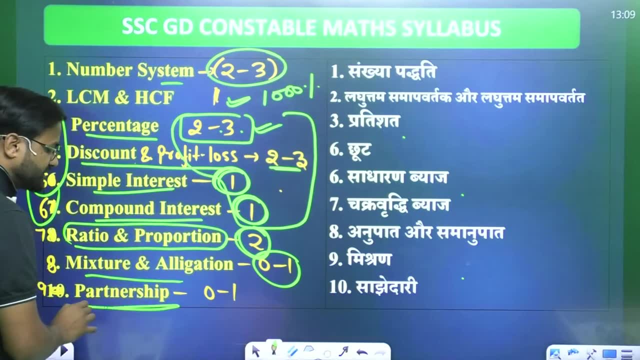 Let's move ahead From a little mixture allegation from 0 to 1 question. It can come, it can not come. That is how much weightage it has, a little less weightage of mixture allegation. Same thing with partnership. 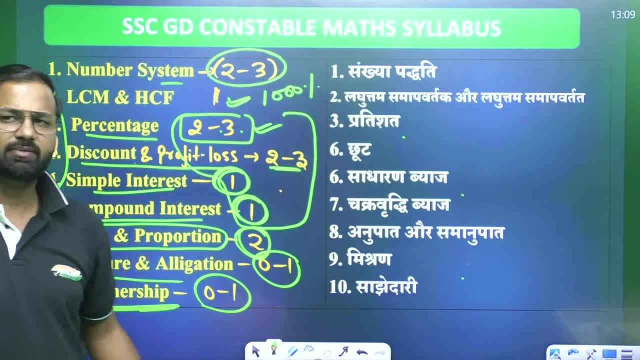 Most of the time I tell you this: mixture allegation and partnership. why did I write from 0 to 1?? Why did I write? Because the SSC is the enemy. The SSC is the enemy of mixture, allegation and partnership. I don't know why. 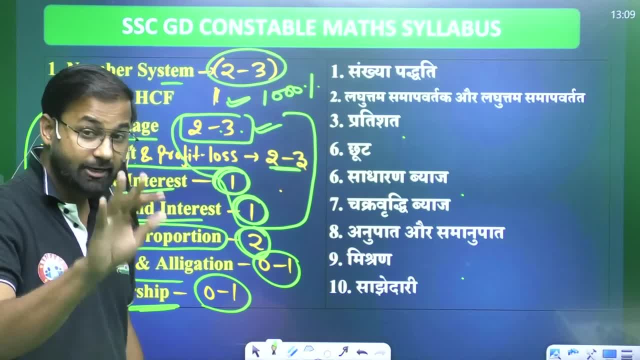 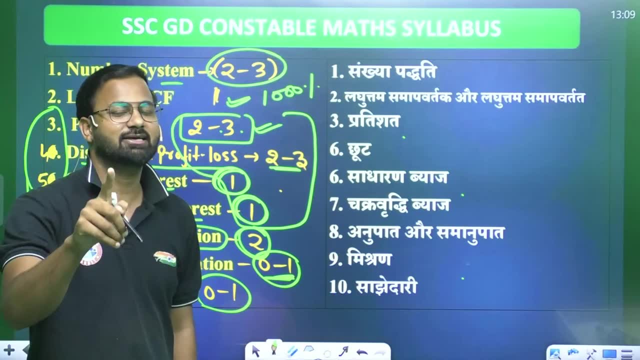 Sit in any exam. The SSC gives very few questions from mixture allegation, But still we will read them very well Because I have put 0 to 1.. It can happen. Examiner is also watching our class. Okay, From 0 to 1.. 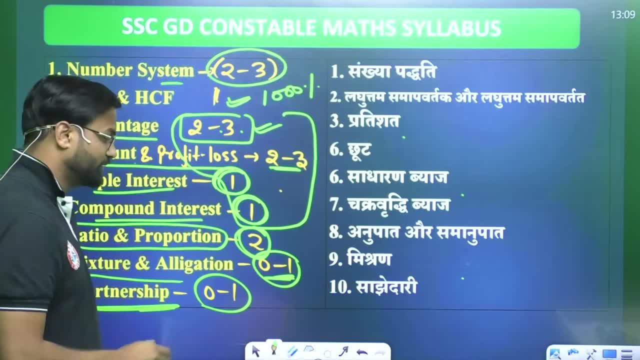 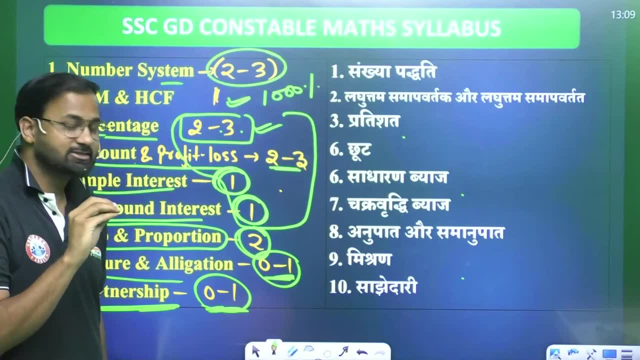 Less weightage. I will keep the question like this, Isn't it? So we have to keep that thing in mind. That examiner can be one of you, So here too, We don't have to go back step at all. 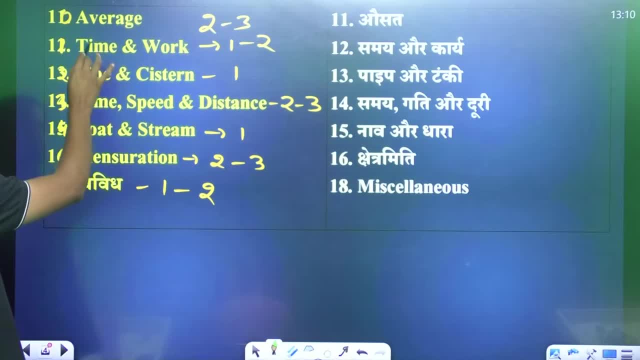 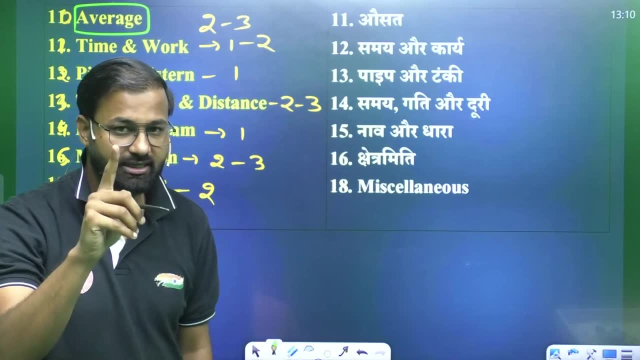 So we have to prepare this thing very well. If I talk about next, Let's go to the next chapter. Next chapter is average chapter, The most favorite chapter. If I talk about the most favorite chapter of SSC, Then you can put that average star above it. 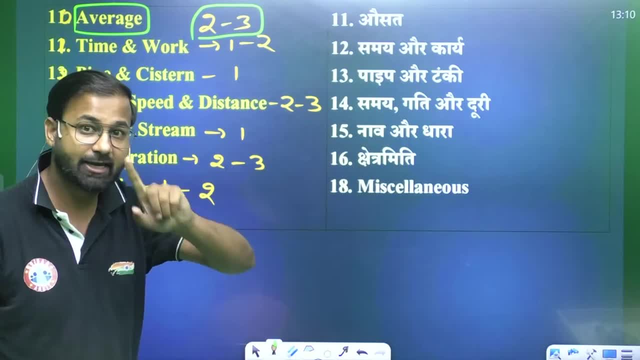 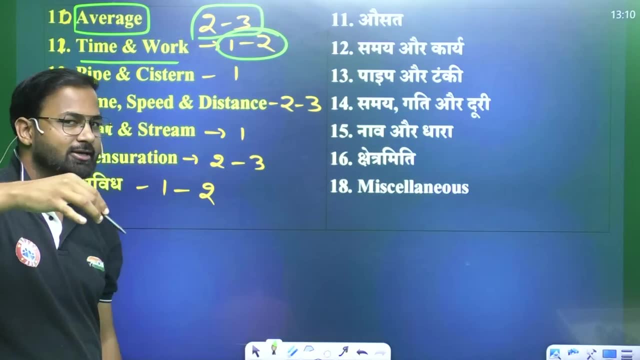 The most favorite chapter and 2 to 3 questions are made from average chapter. Okay, Let's go a little further Time and work 1 to 2 questions. And if I talk about SSC, In which chapter can you make the best question? 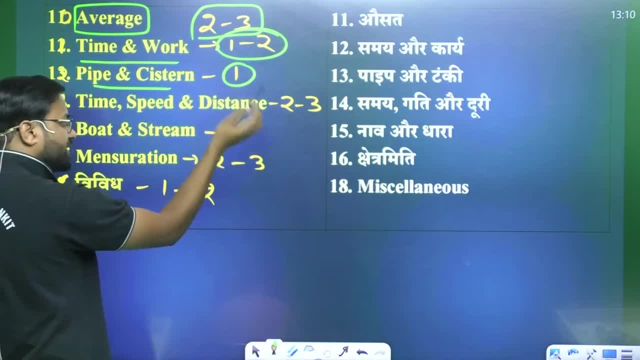 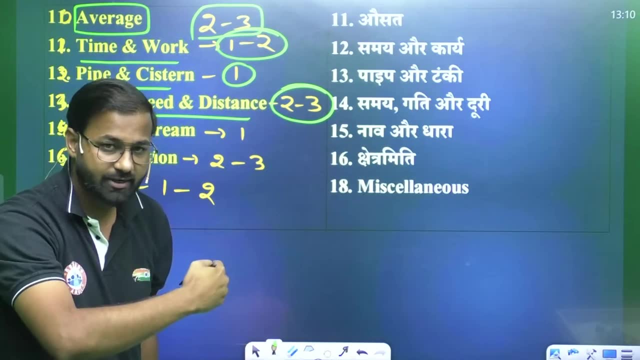 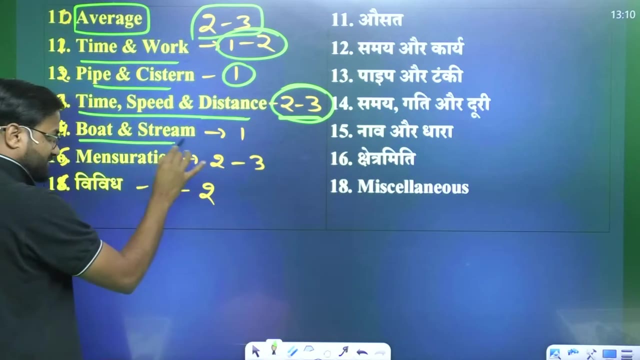 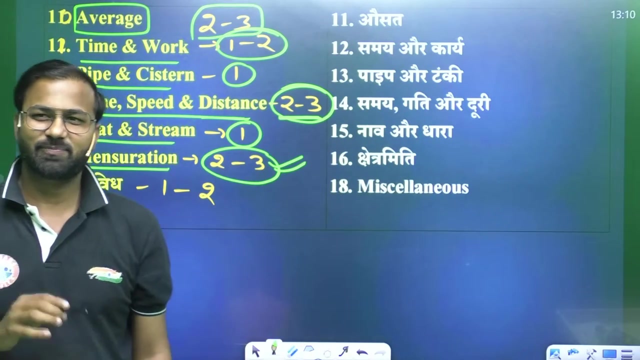 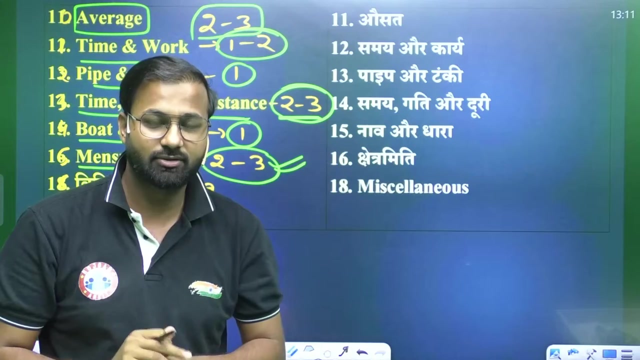 I will tell you that too. In which chapter will it be made? I hope to get a question from the pipe system. 2-3 questions from time speed distance. I have done previous year analysis. I have not written in the air like this. I have done previous year analysis. 2-3 questions from time speed distance. 1 question from boat stream. 2-3 questions from mensuration, and this mensuration is such a topic that is looking at mensuration the light of your mind. if there is a yellow light, it will turn red. if there is a red light, it will turn more red. 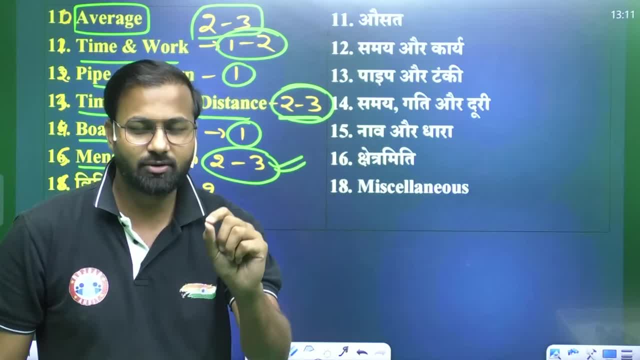 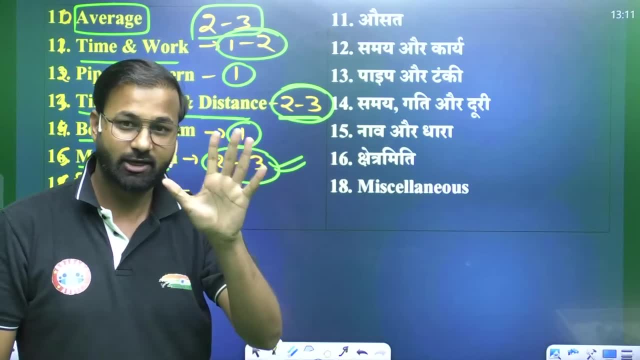 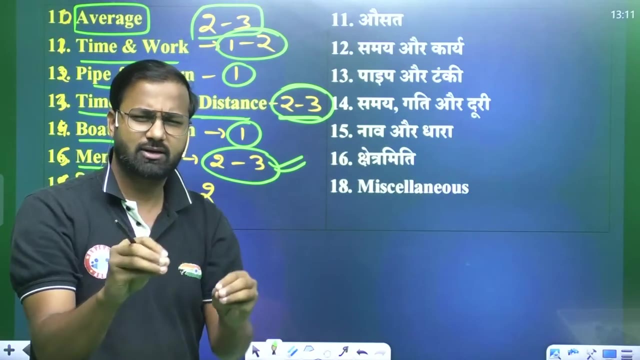 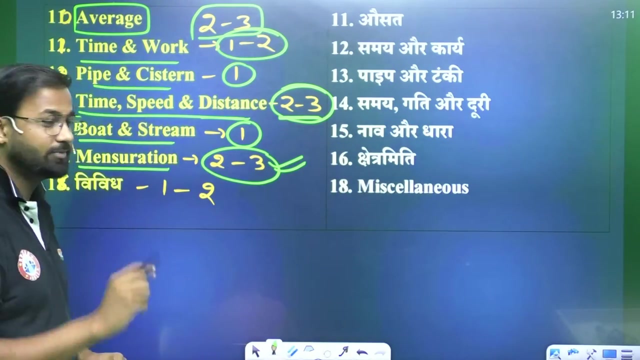 Sir, mensuration will not come, and the day you read mensuration from me, you will say: sir mensuration comes. the rest of us are already perfect. bring the question of mensuration first, because we can do limited things very well and do a lot of things lightly. there is a difference in both things: in exam oriented reading and in reading. there is a difference in both. we will read exam oriented things, okay. 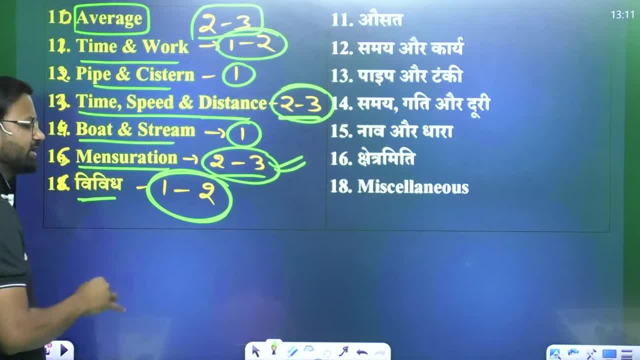 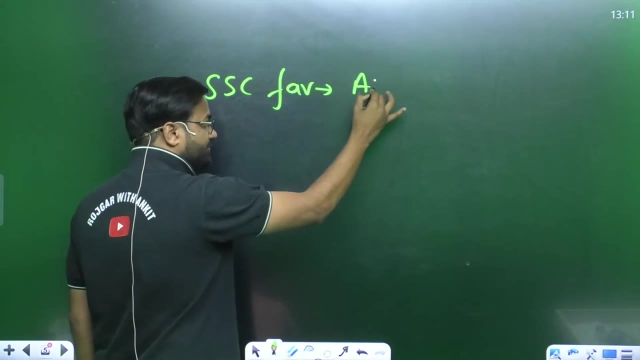 The thing is, if something is left- DI, etc. Whatever is left of, regardless of the life of sadness, we will keep it in the middle of the various wisdom. I will tell you that the most favorite topic of SSC. I told you which is the favorite topic of SSC, I told you. I told you average. 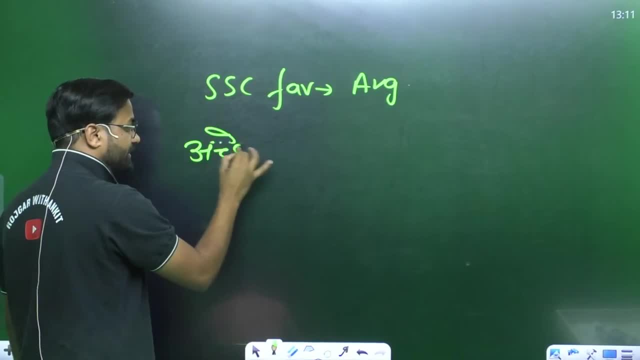 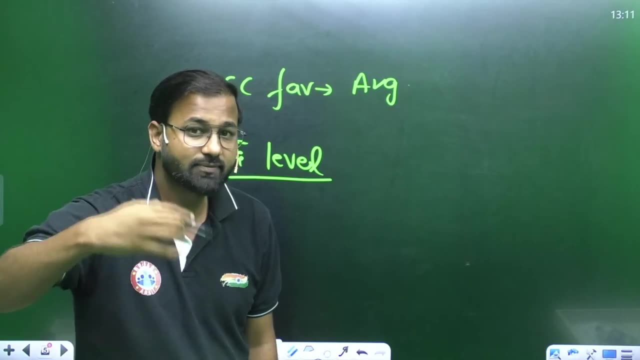 The second thing I will tell you. the question of good level will be made. from which chapter of good level, which you call hard questions in your language. hard questions, hard, nothing happens. level becomes a little good. Good level question children. Either made from a chapter or made in a short time- Good level- which will be made in six days- or if you have done it. if you do not feel like it, you can do it. So it is a little difficult, you can do it. 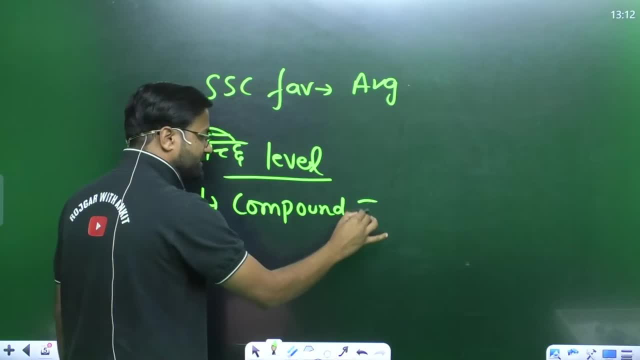 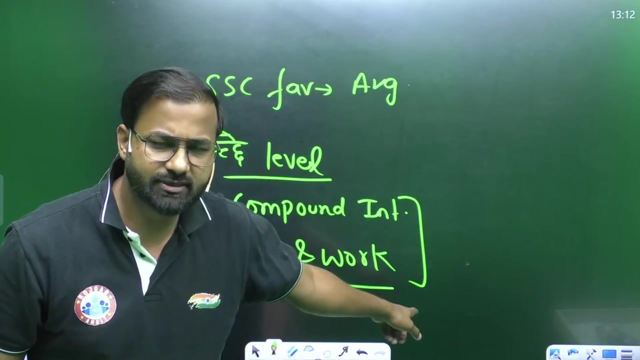 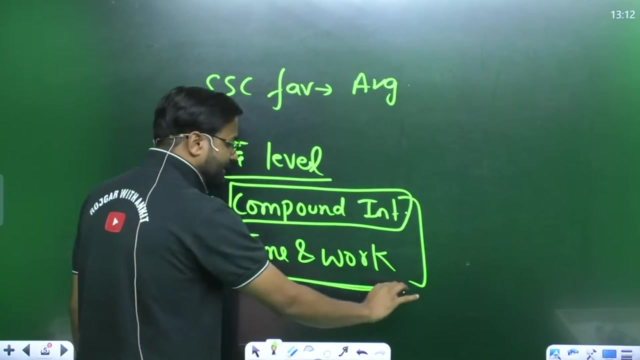 in compound interest or in time and work. These are the two chapters in which good level questions have been made in SSCGD. If you look at the previous year, if a good level question is made in SSCGD, then it is either made in time and work or in time and work. 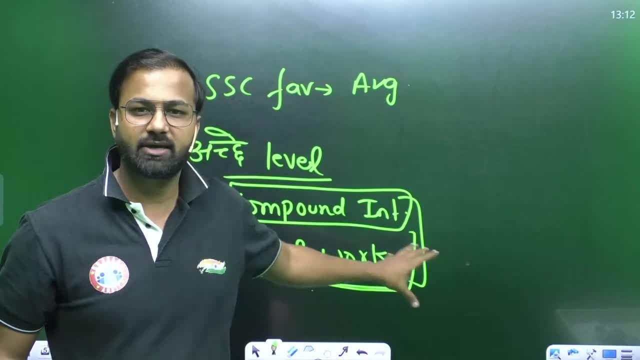 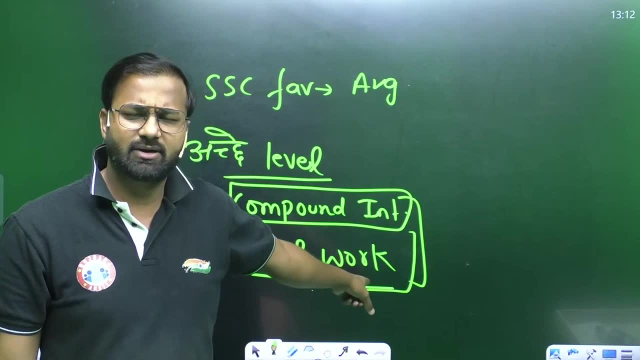 And what does it mean to do analysis on these? Why am I saying this? I will make these two chapters your backbone. I guarantee You will feel that how good a question will be made. We will not go back in these two chapters. 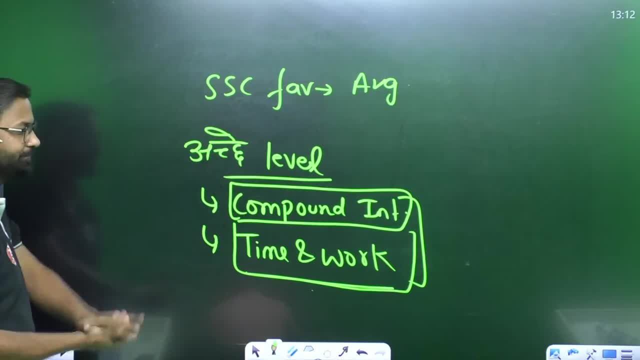 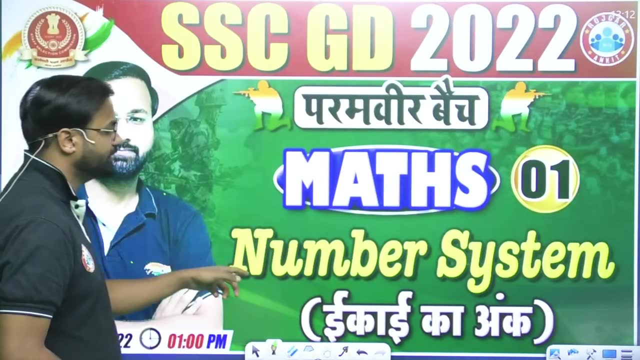 Okay, so you will go through all the syllabus, Okay, so let's start. Okay, what is our chapter? Those who have just come, let me tell them: In the number system, unit digit will be our chapter today. Sir, what is unit digit? 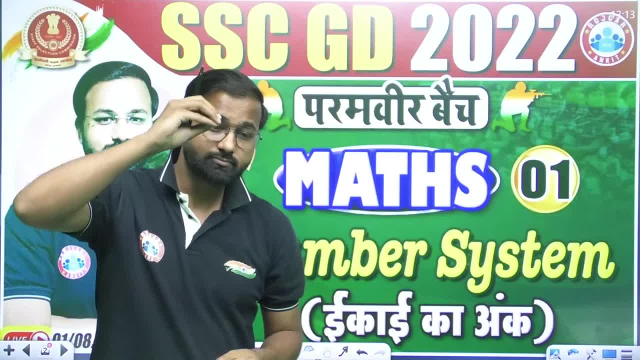 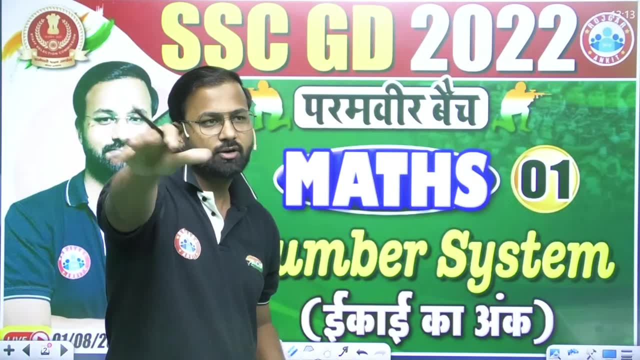 I will start with the basics. I will say it from the basics. The kid who has opened the video for the first time. I have to prepare for GED. I want to get young And I have opened the video. I don't know what will come- math or what will come. 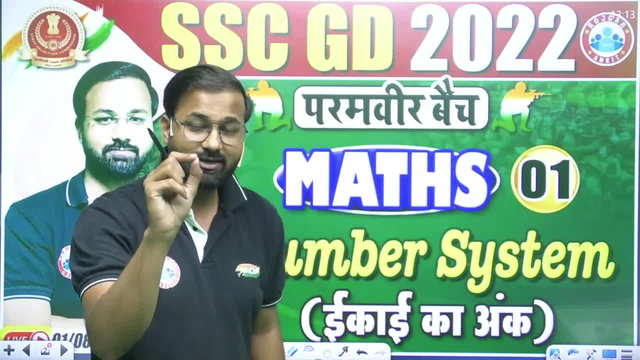 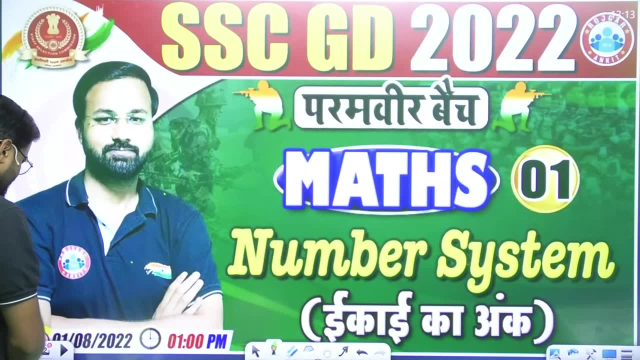 I just opened the video and sit down, Take the number in GED. this time He will also be cleared in this way today, If he also finds a question, then he will only find the number of 1.. Okay, so let's start the number of 1.. 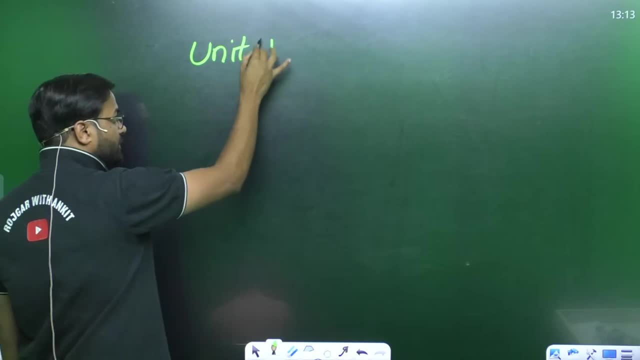 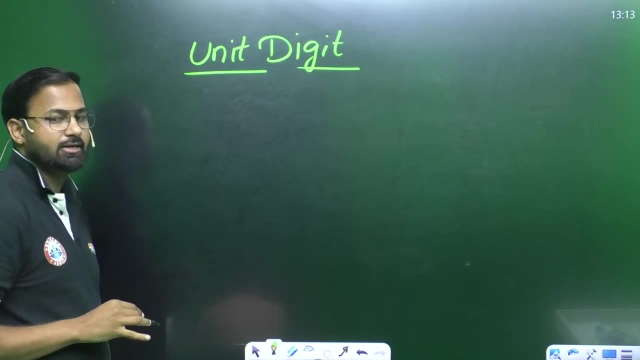 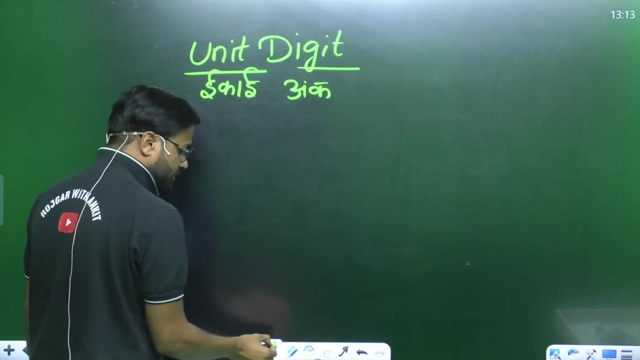 Unit digit. I will teach bilingual, don't worry at all. I will teach bilingual to both English and Hindi students. Unit digit, ie unit number. First of all, what is unit? What is unit? Let's talk about unit number. 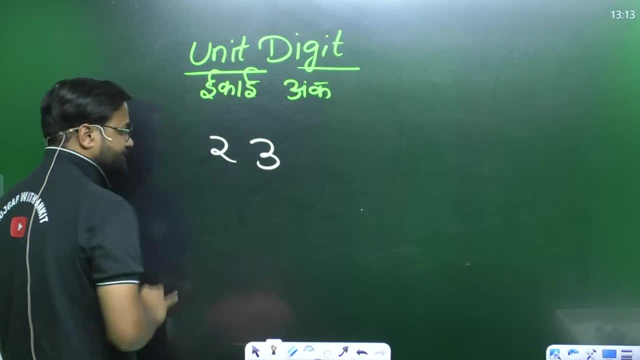 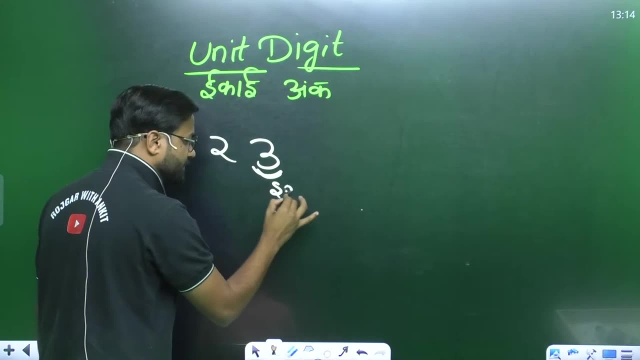 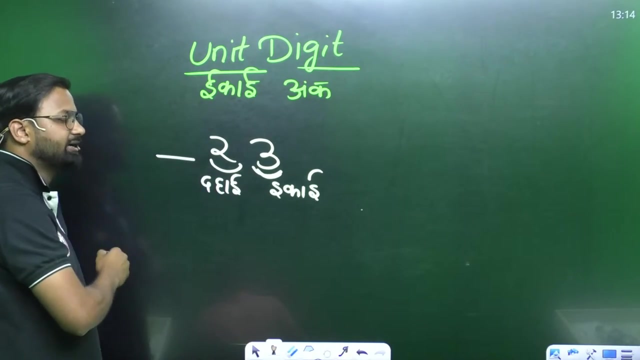 I have written a number 23 here. The first digit on the right hand side will be unit. What will happen? It will be unit. The second digit on the right hand side will be unit. The third digit on the left hand side will be hundred, and then thousand. 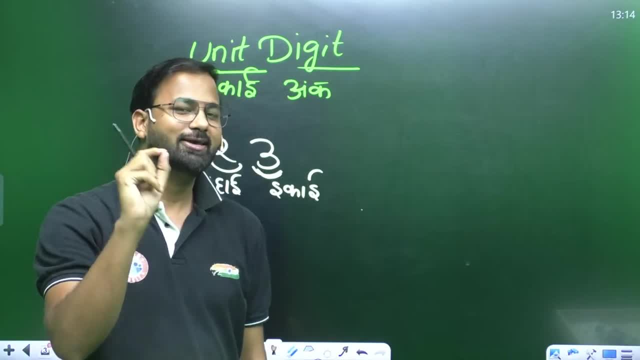 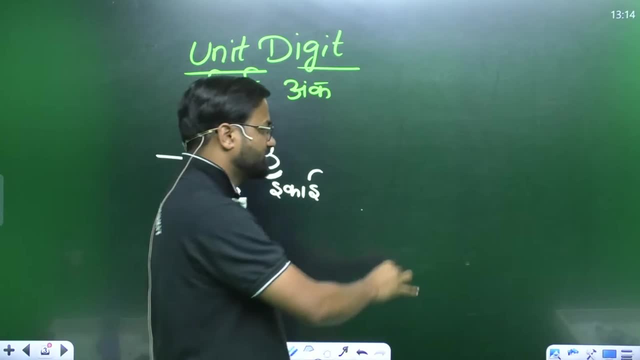 What is the name of the chapter? The name of the chapter is unit number. No need to take tension, Just read it with a smile. Math will be clear with a smile, And even if you get 24 numbers out of 25,. 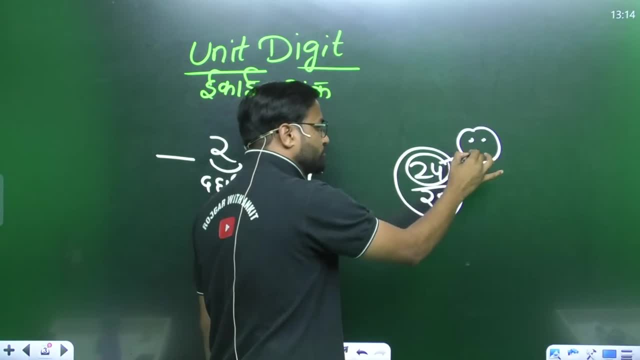 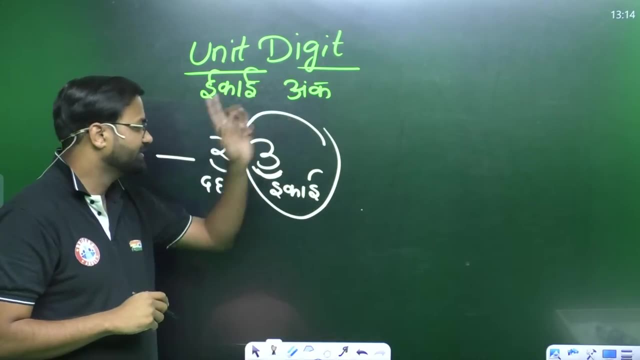 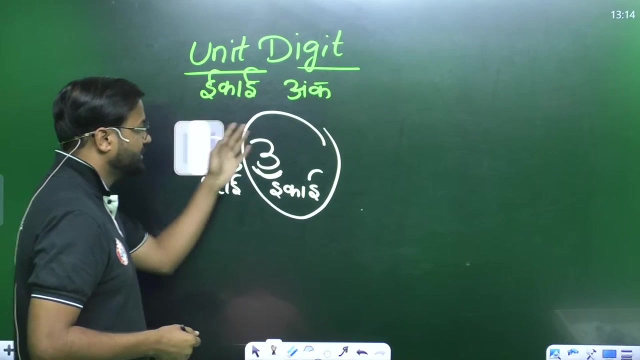 believe me, 24 numbers, you will be sad. 25 out of 25 will be your number. Okay, So here I am talking. We just have to talk about last digit. What can be the last digit in any number? Like I wrote a number here, 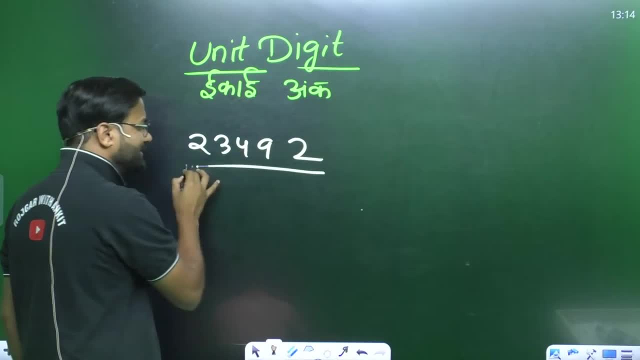 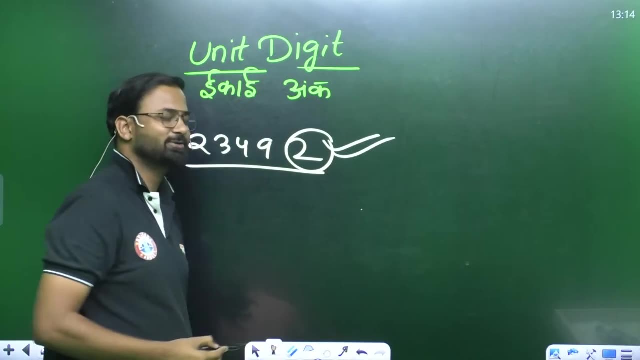 I wrote 23492.. What is the unit number, Sir? you just told the number of the last digit. The number of the last digit will be the unit number 2.. Why do not you ask such questions? I won't ask such questions. 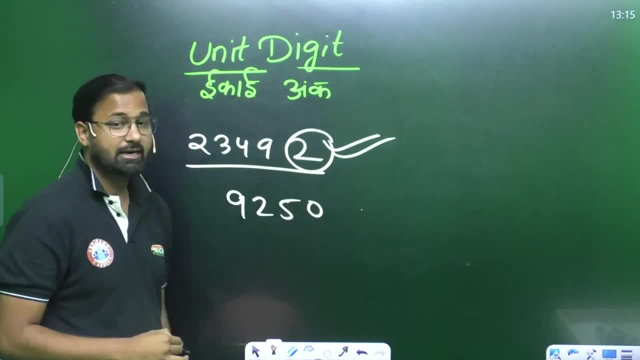 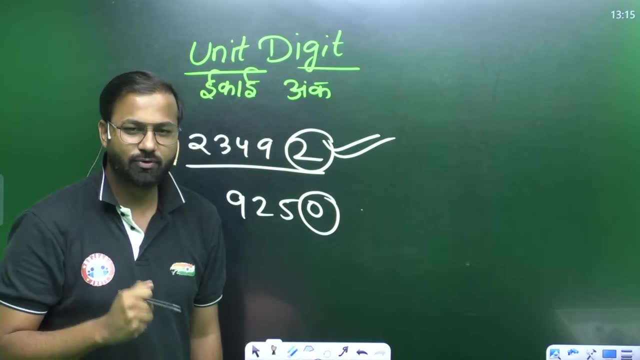 I will tell you now. I said 9,, 2,, 5,, 0.. What is the last digit, Sir? the last digit is zero. This is how the last digit is. But, sir, we have not seen such questions in any book till date. 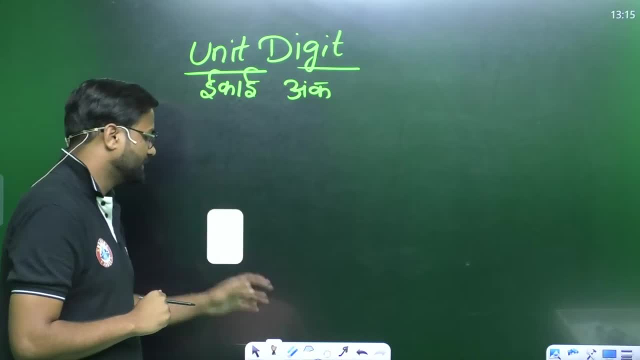 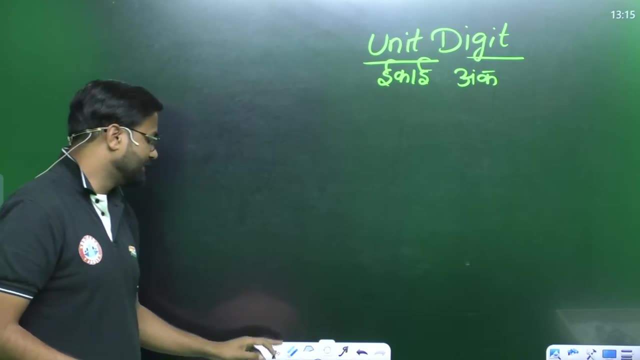 No problem, I am just starting now. Okay, I am just starting now. The warm-up before running. that is the warm-up, Don't worry, All right, So I will move a little further in the last digit. Last digit. 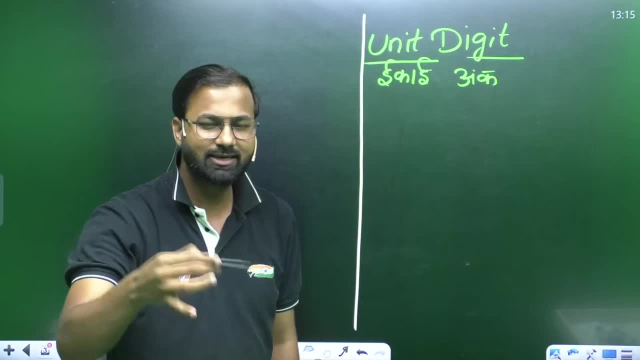 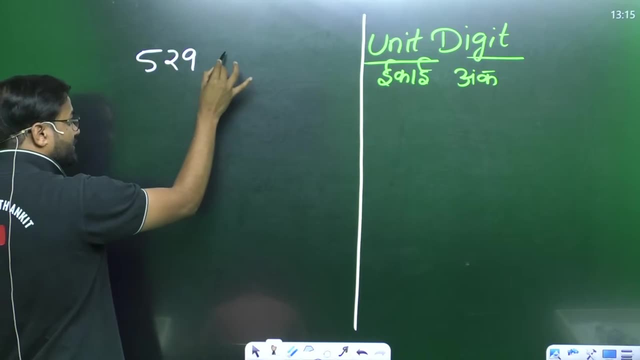 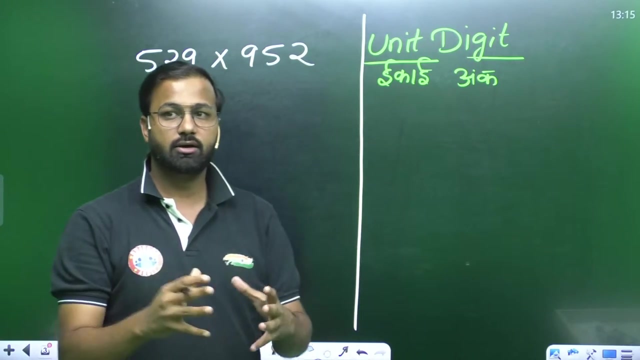 I have told you what happens. The last number of any number is the unit number. Suppose I write a number 529 x 952.. Sir, what will be the unit number when I multiply such a large number? When I multiply such a large number, what will be the unit digit? 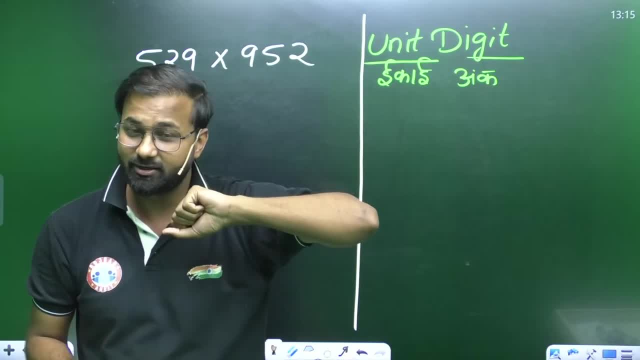 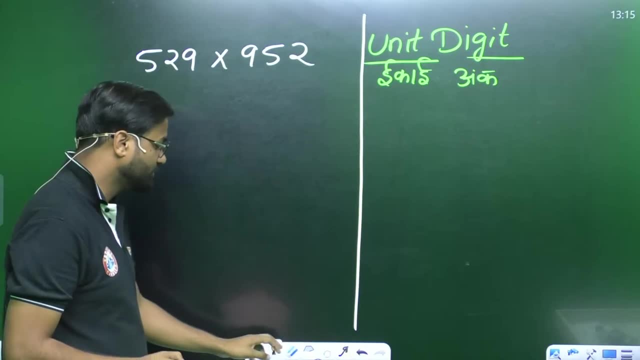 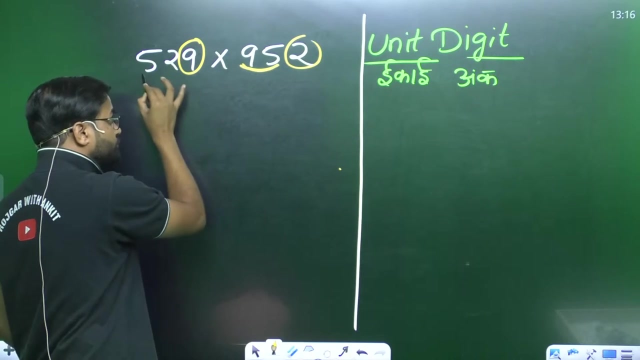 Sir, you have told the numbers directly. What will be the unit digit of such a large number? You have to remember a simple thing: In the unit number, our meaning will be only from the last digit. Only from the last digit. Sir, whatever food is being cooked here, we have no meaning. 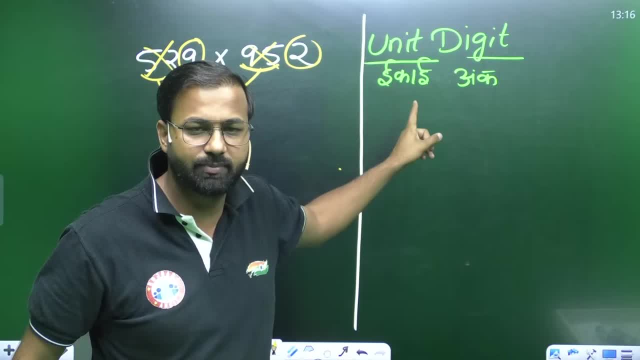 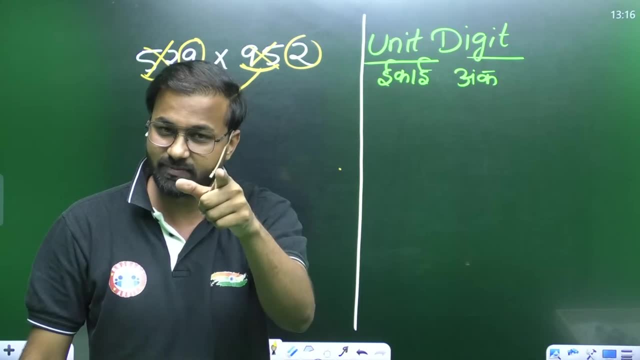 We have no meaning. Whatever food is being cooked before the unit number, we have no meaning. Our focus is on the eyes of the fish. Where was Arjun's focus? Our focus will be on the eyes of the fish Only in the unit number. 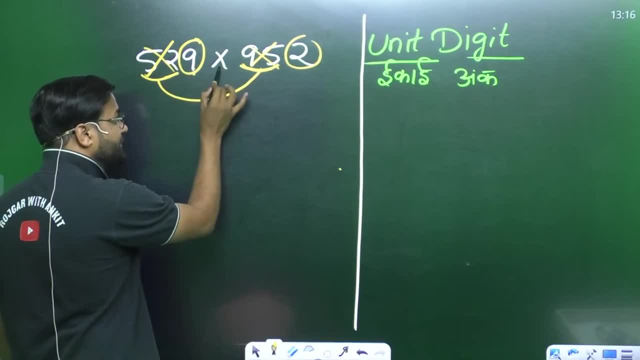 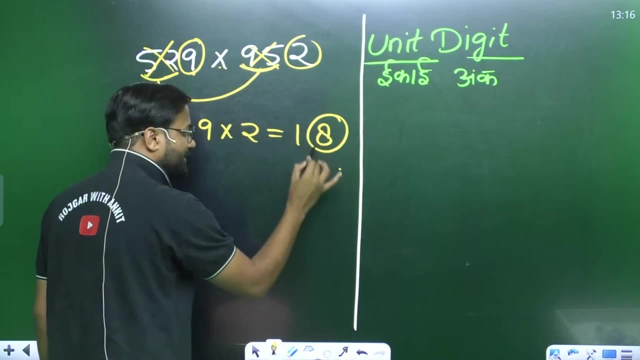 Only in the unit number. So here the unit number is 9.. In the middle is the sign of the number And here the unit number is 2.. What is the unit number of 9?? 18.. And the unit number of 18 is 8.. 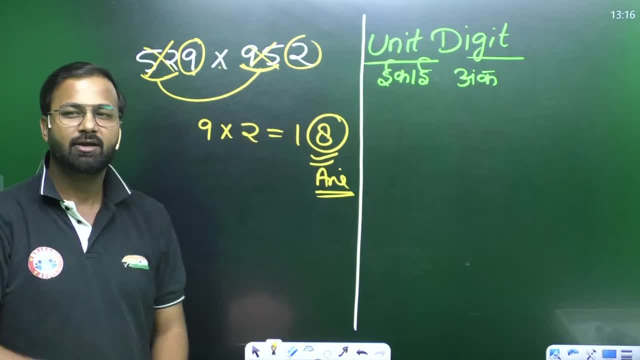 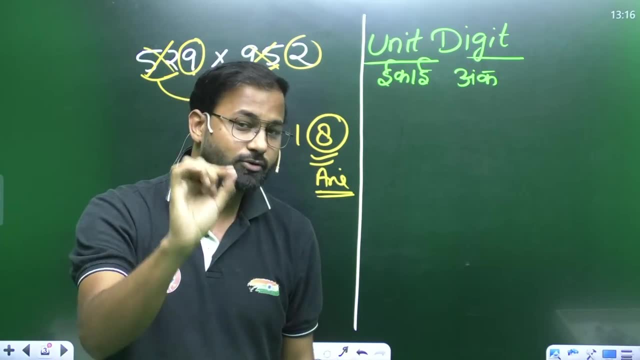 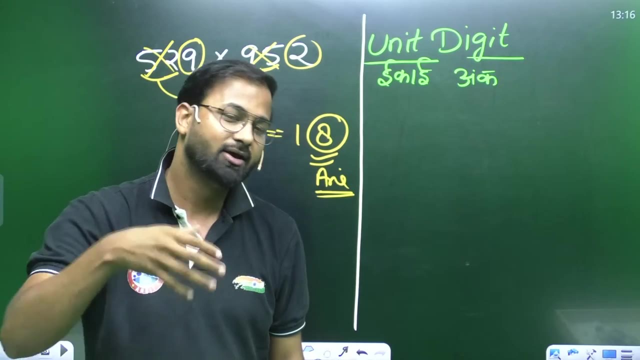 And this will be your beautiful answer. Don't try to make fair notes in the notebook. You will get PDF notes. Download the Rozgar Vidankit application. You will get a free PDF. And this is not the first time. We do this- every time. 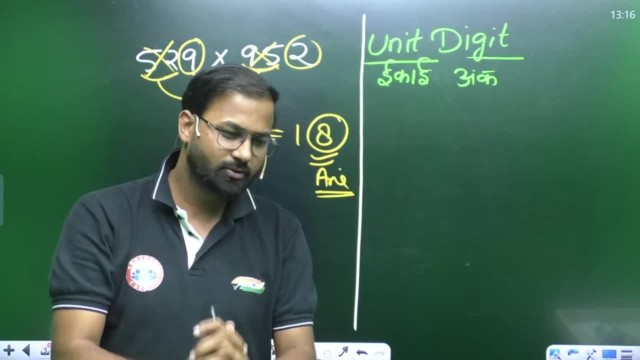 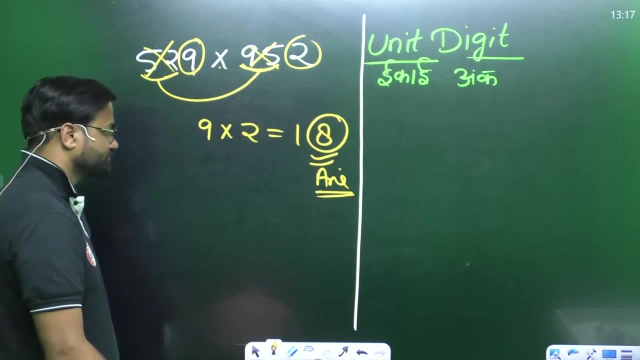 Our channel does this every time. You are our family, We are your family, So things are our responsibility. Give the things properly. You will get the PDF. Don't worry. Don't write. No need Sit with a rough copy. 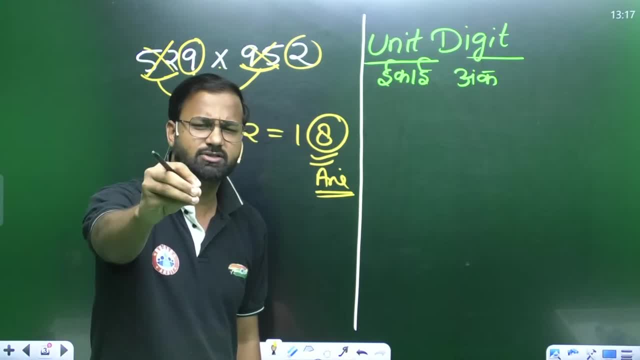 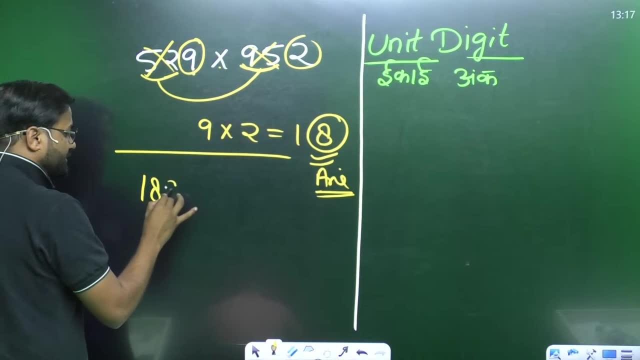 Whenever you do my math class, sit with a rough copy. Focus more on what I say, Not much on writing. I deliver things a lot. I said here: 1895, times 292.. Tell me what is the unit digit? What will be the unit digit? 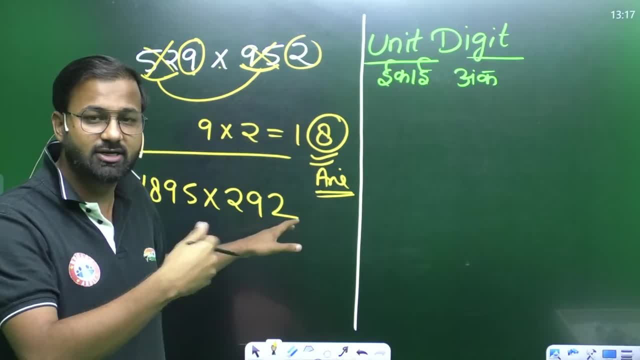 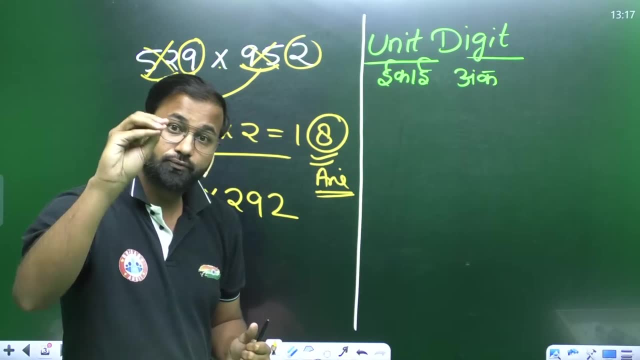 What will be the unit digit? This warm-up is going on. I will tell you more slowly The number of powers. The ones that are on the Ghat, They will also get the unit number. The factorial ones will also get the unit number. 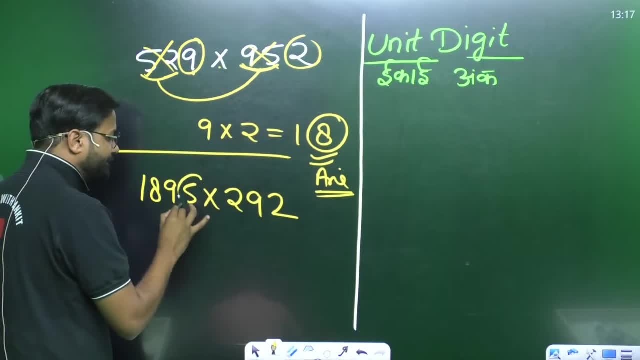 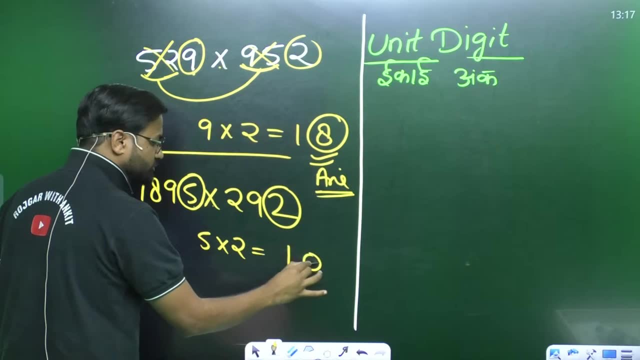 I will teach you. There is nothing to worry about. There are 5 units here. There are 2 units here. There is a sign of quality in the middle. How much will it go? 5. 10. 10- very good numbers. 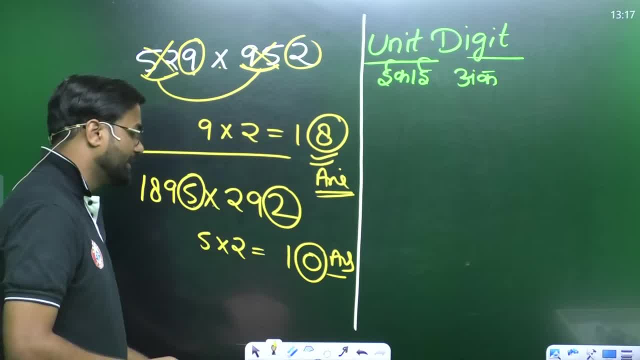 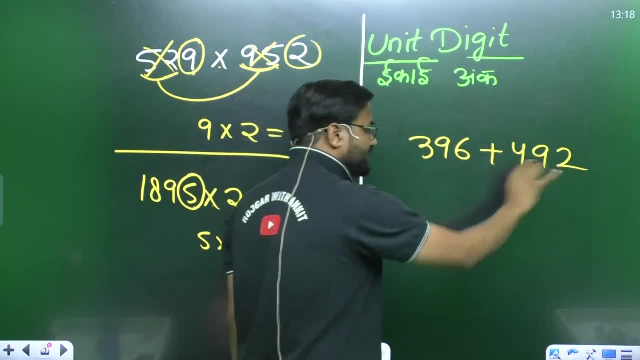 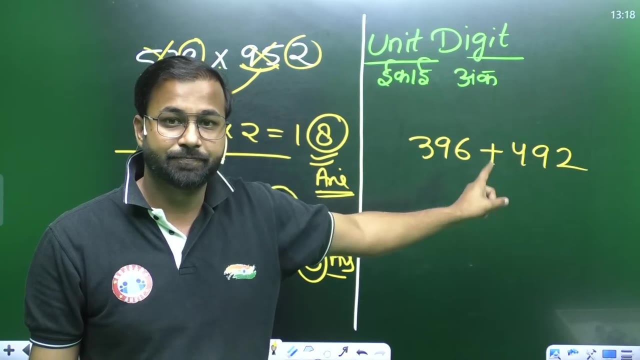 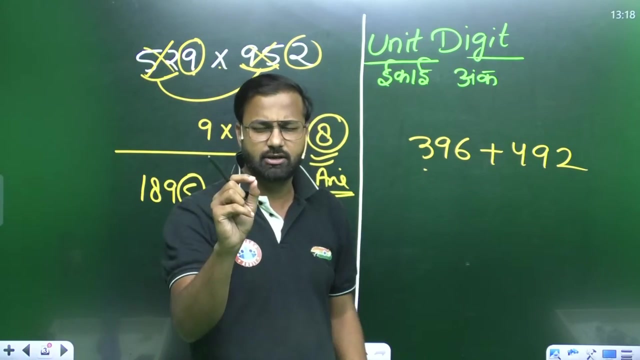 10 will be the benefit of this wholeif 고민. It will also will be the success of this knowledge. So father falls 490.. It is tell all to connect 396 with 492 to write a joint number. I said that whenever I talk about the unit number then I should only mean by the unit number. 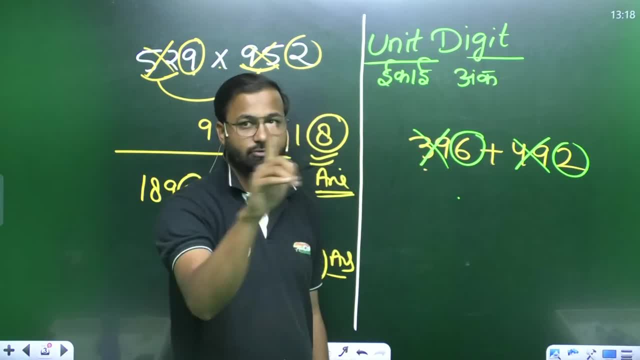 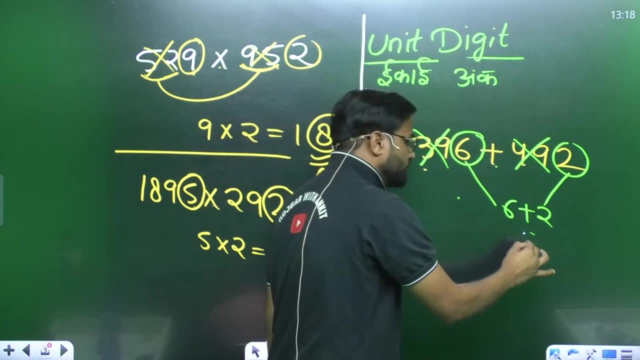 I don't care about the rest of the khichdi, I am unit digit, focus, unit digit. So how much will be the unit digit? 6, plus sign in the middle 2.. Unit digit will be 8 and this will be your correct answer. 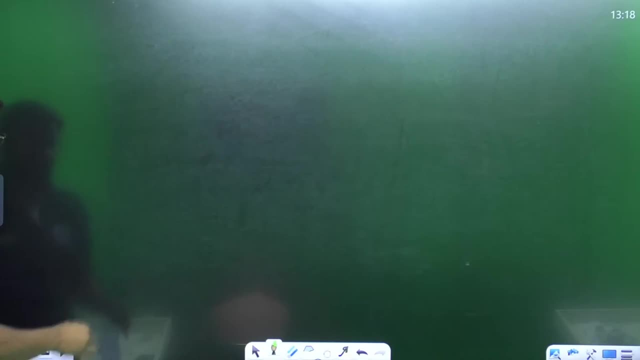 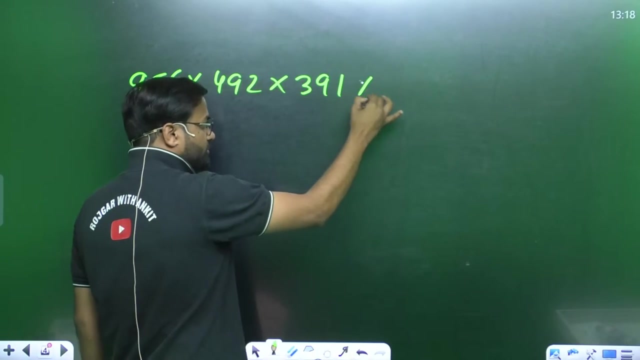 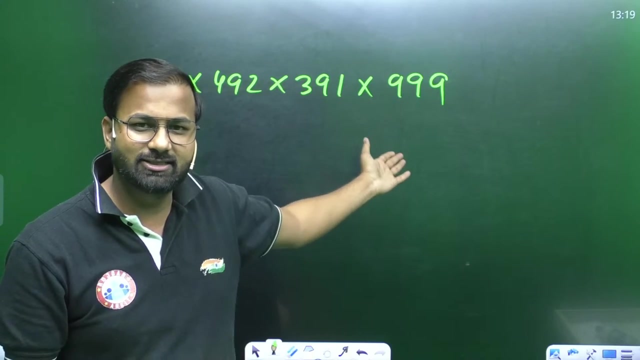 Is it clear? Shall I give you a question: 956 multiplied by 492, multiplied by 391, multiplied by 999.. How will you tell such a big unit digit? Even a calculator cannot tell this much. Are you less than a calculator? 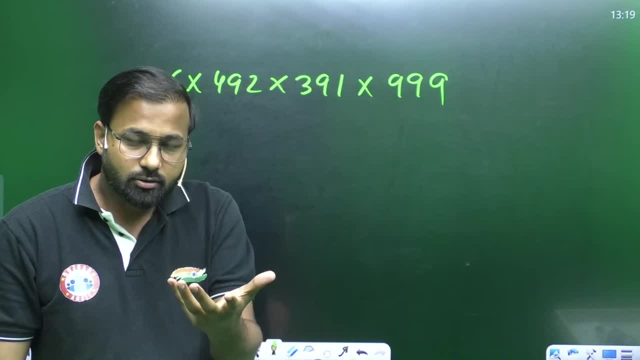 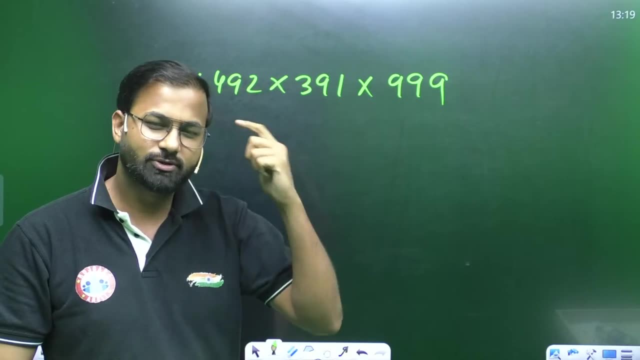 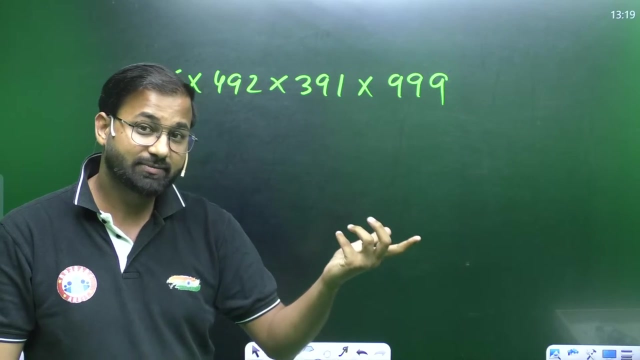 Who made the calculator? Did the person make the calculator or the calculator made the person? If the person made the calculator, then it is important that our mind should be faster than the calculator. We are the progeny of the calculator. If our mind is faster than the calculator. 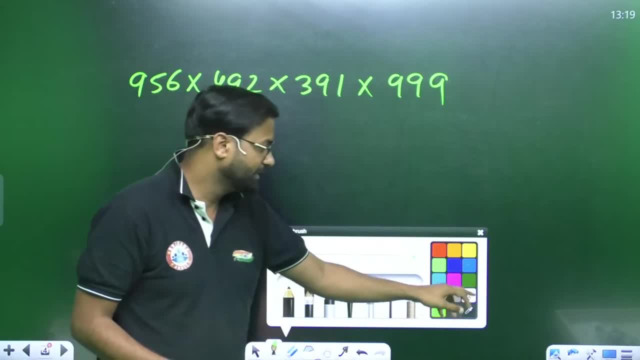 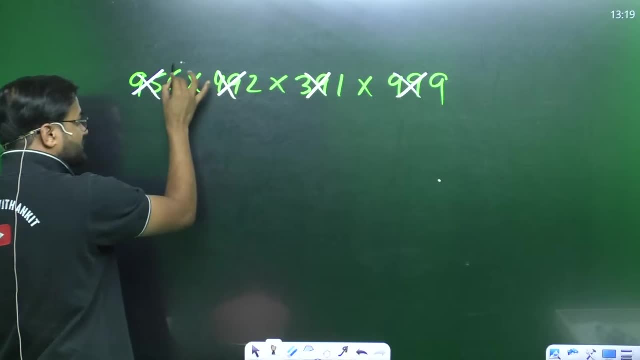 then the unit digit will be very fast How You will see that the rest of the khichdi does not mean anything. Our focus should be only on the last part. 6, plus sign in the middle. 2, plus sign in the middle. 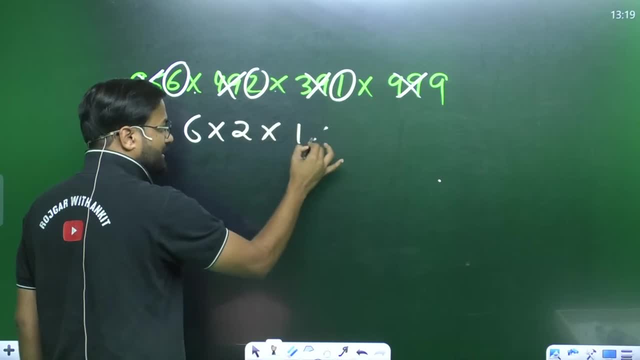 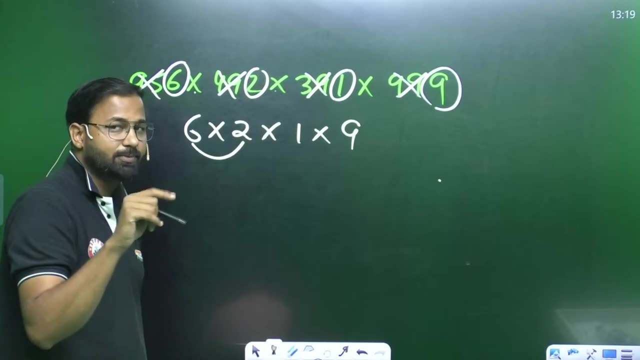 then 1, plus sign in the middle, and then 9, plus sign in the middle. Now multiply it here too: 6 times 2,, 6 times 2,. now see what you have to do here. Look at the front. 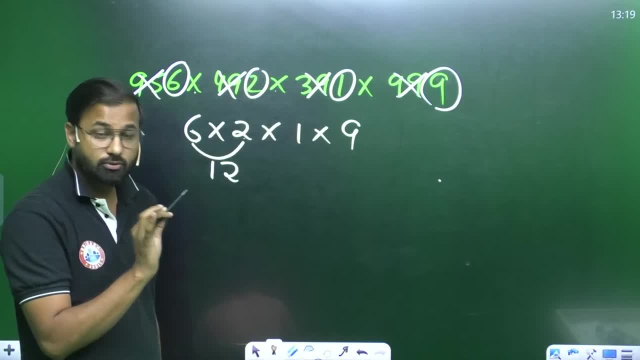 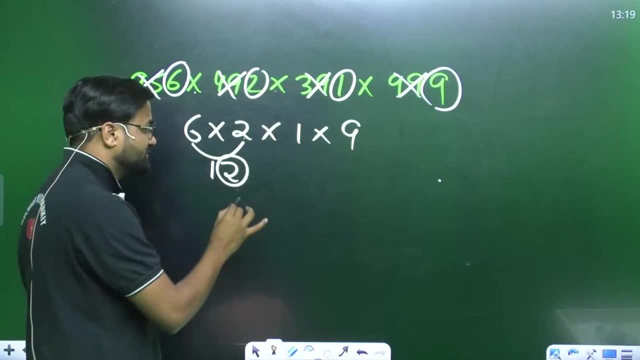 6 times 2, 12.. 12 is here After multiplying 2,. take the unit digit of this 12 too. Yes, take the unit digit of this 12 too, And multiply the unit digit of that unit by the next number. 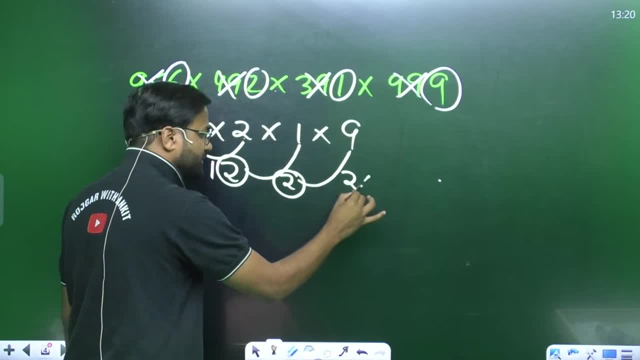 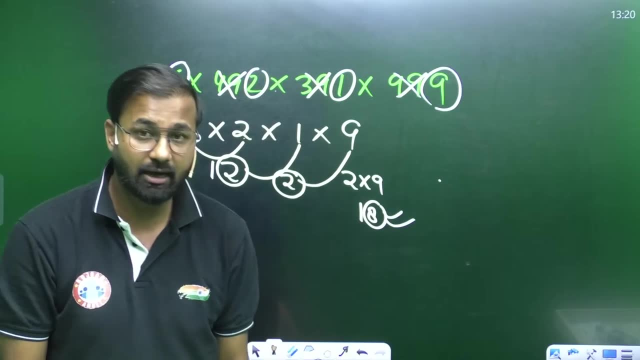 2 times 1 is 2.. Then multiply 2 by 9.. How many are 2 names? 2 names are 18.. 18 is 8.. You are absolutely correct, Sir. I have understood a little less. 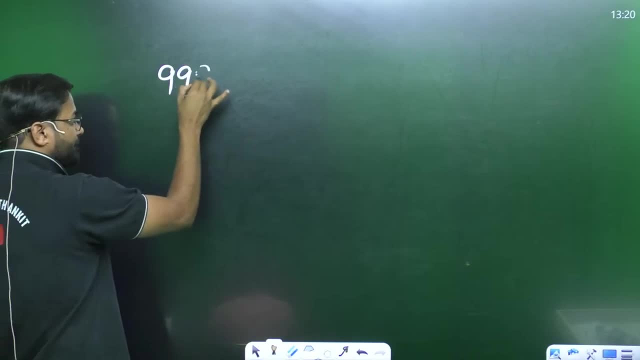 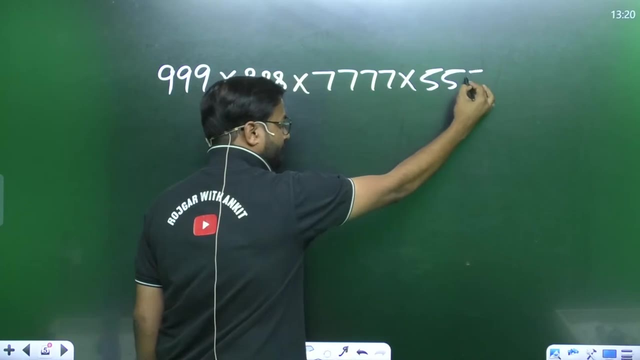 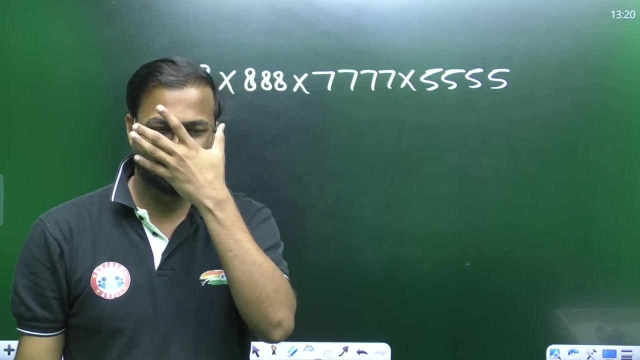 Ask me one more question. Let's ask, Ask this question: How big is the unit digit? You have improved a little. I have to tell you a lot of things now. It's just the beginning. What has happened now? What has happened now? 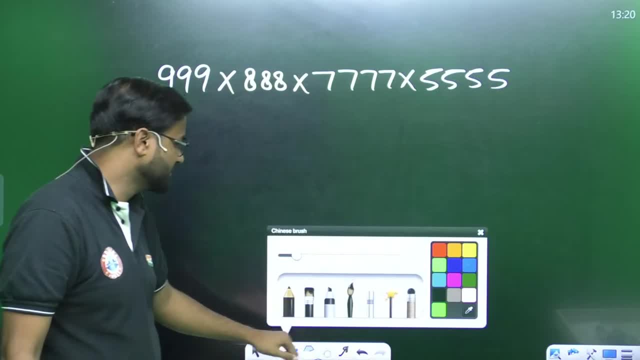 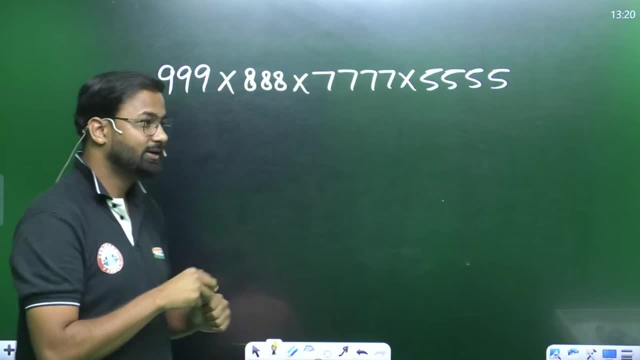 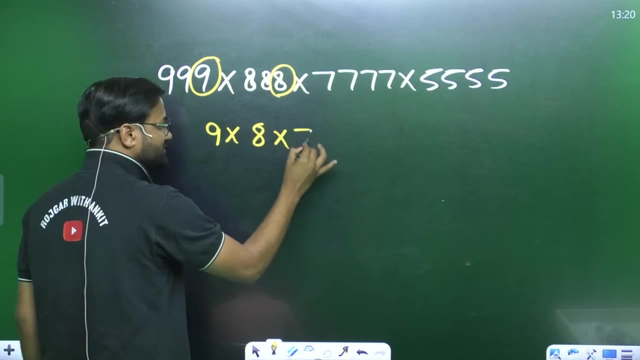 Nothing has happened. I have to tell you a lot of things now. As I wrote this number here, I said I don't care about the rest. I mean the unit digit. I will take the last number: 9,, 8,. 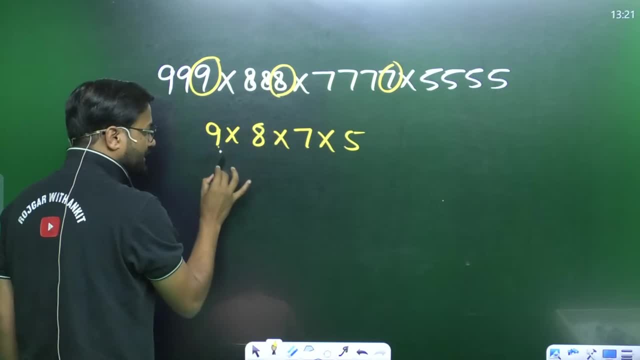 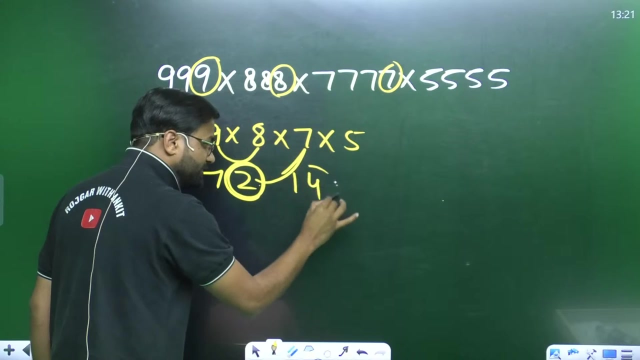 7, 5.. We will multiply 9 by 8, 72.. Now don't multiply 72 by 7. The unit digit of 72 is 14.. Take this and multiply 2 by 7.. 2 times 7 is 14.. 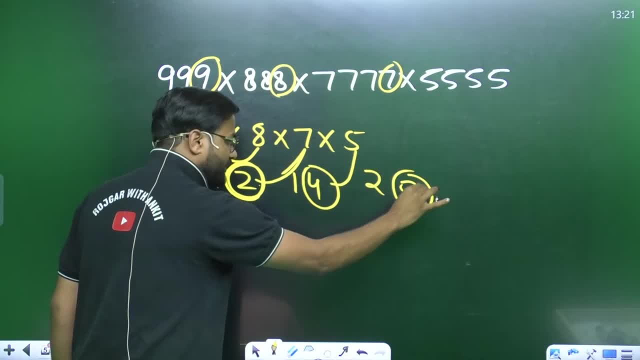 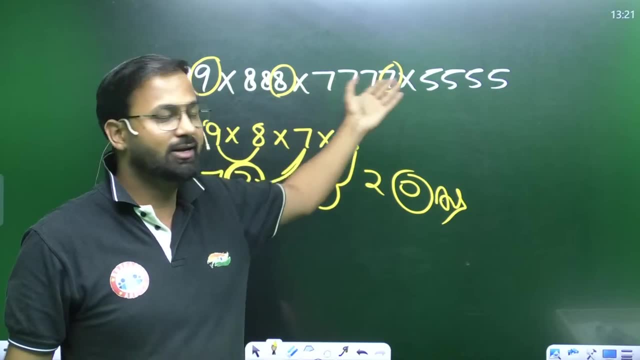 Take 4 of 14.. 4 times 5 is 20. And 0 will be your answer. The unit digit is over. You have taken out the strength of the question. I have written such a long calculation and you have given a zero answer. 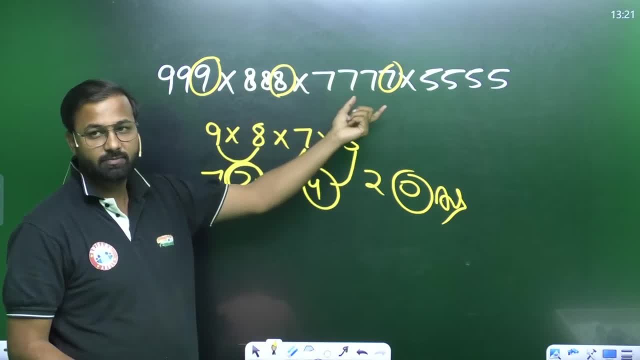 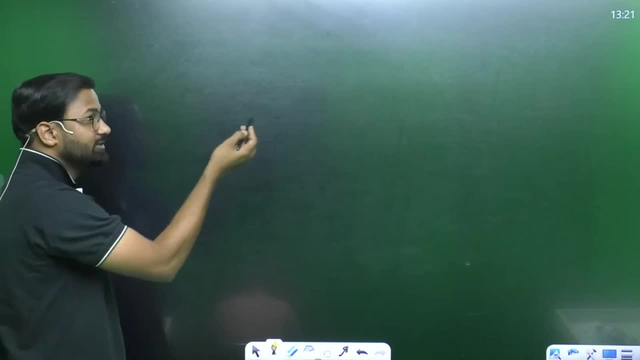 It doesn't happen like this. Have some respect for the question, Put a little mind in it. Why are you getting so fast? Very good, Now let's go through the unit digit of powers. Unit digit of powers. Unit digit of power. 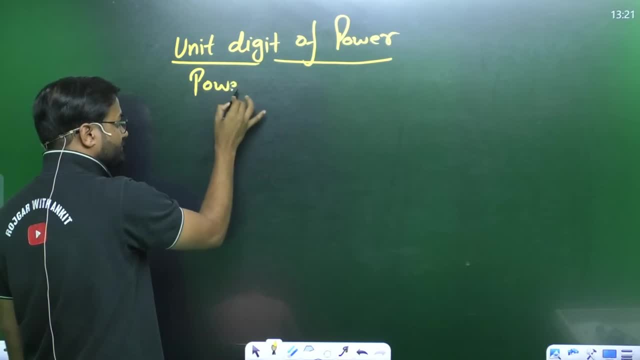 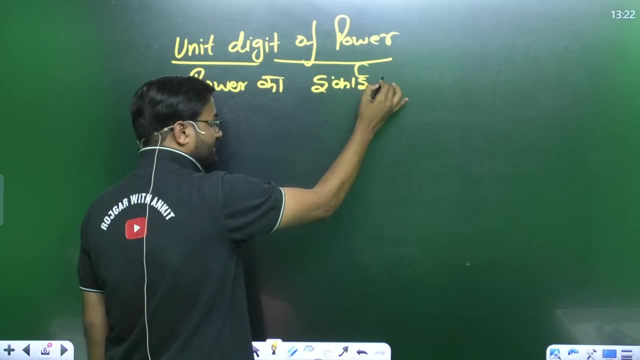 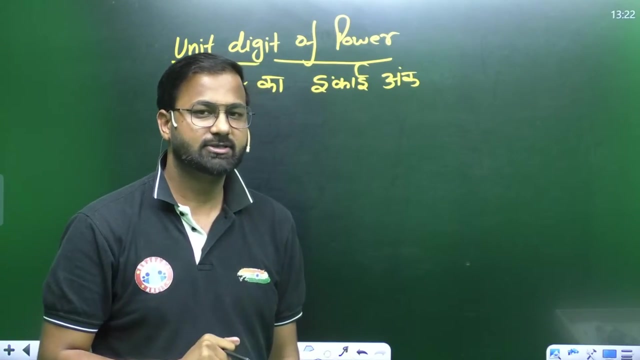 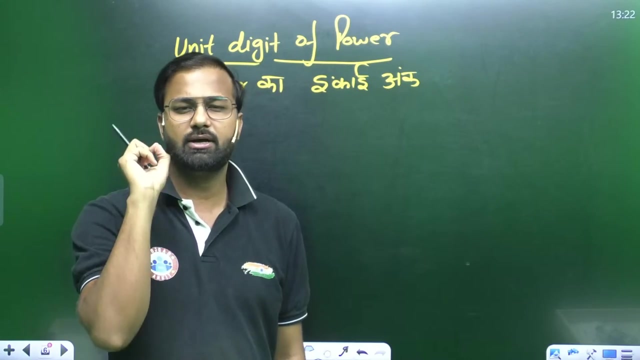 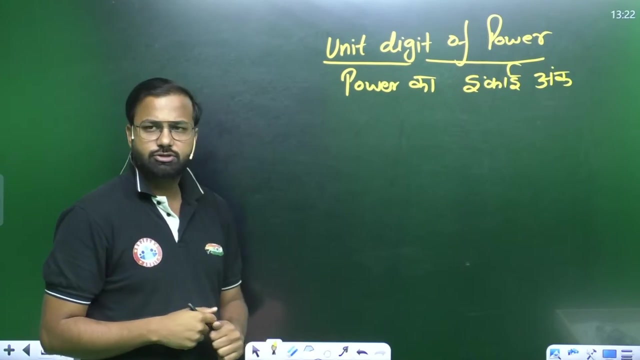 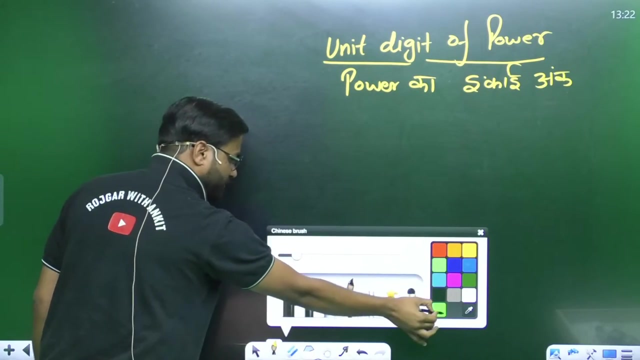 Unit digit of power. We will write: unit digit of power: Ikaai ang Power, Ikaai ang Basic. Now let's go to power. There are some rules in this. I will not give you many rules because I find it very confusing. I will give you a simple rule from which you have to do things. is it a topic of power, sir, power is a very big power. we have seen there is no problem. now I will tell you what the first rule number one says: in the power of Ikaian. you can write this in the copy: what does rule number one say? rule number one: rule number one says: 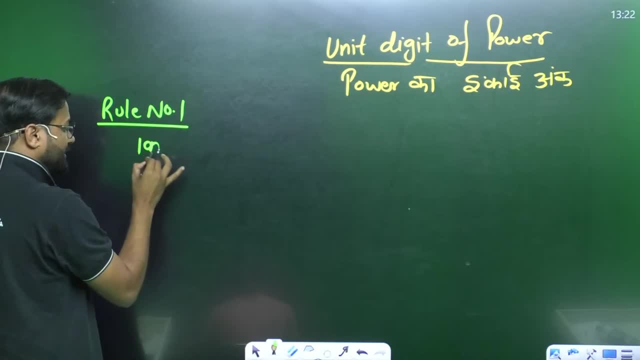 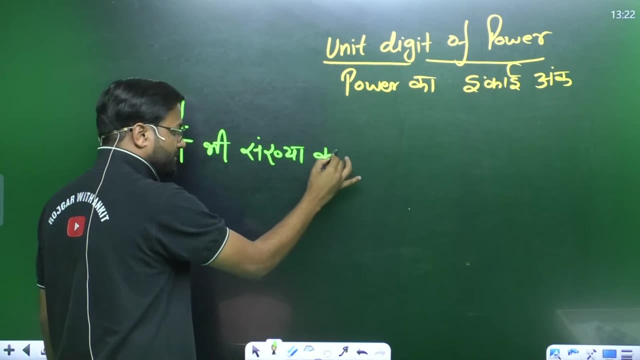 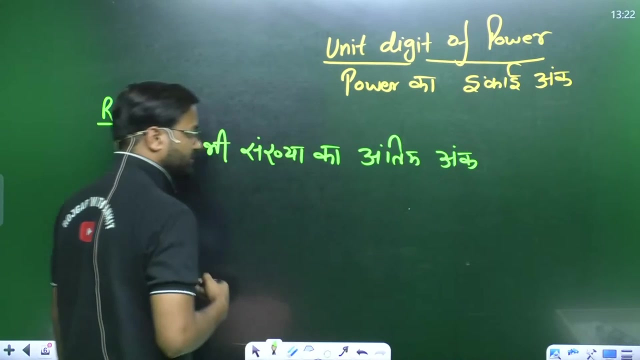 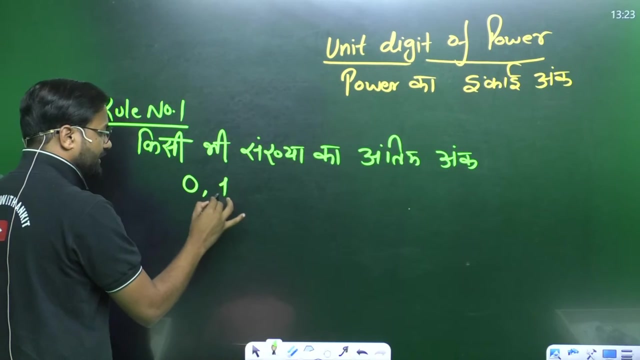 any number's last number. what does it say? any number's last number, last digit of any number. English people will see: last digit of any number. if the last digit of any number, any number's last number- 0,, 1,, 5 and 6, what is the number? this code should be written. 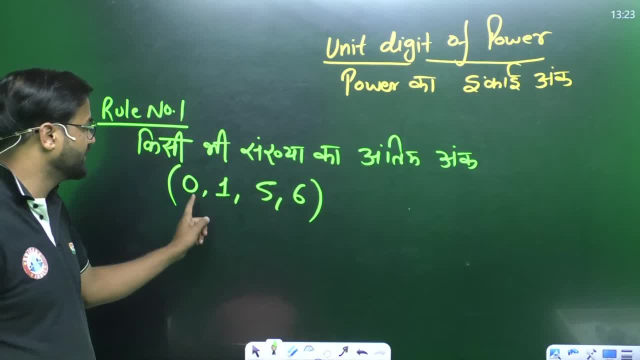 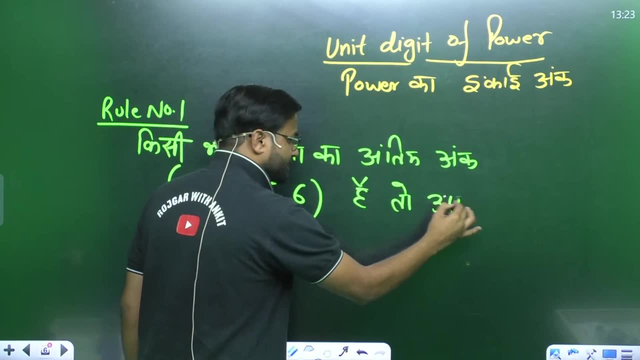 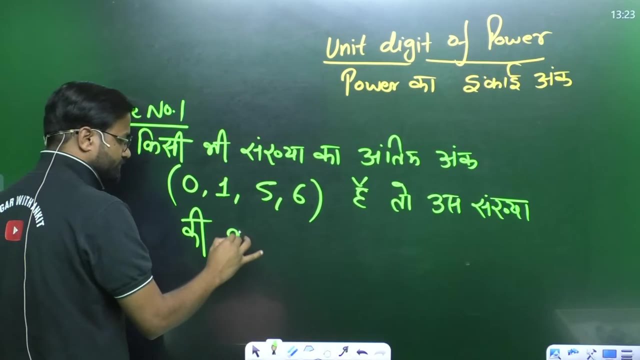 you people? what did I say? any number's unit, digit, 0,, 1,, 5,, 6, if there is then that number, that number, that number, whatever power, whatever power of that number, whatever its loss. 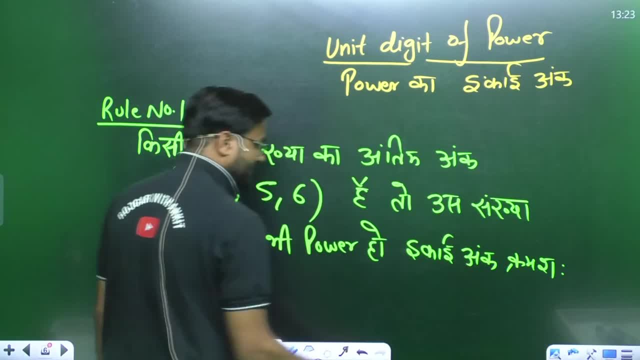 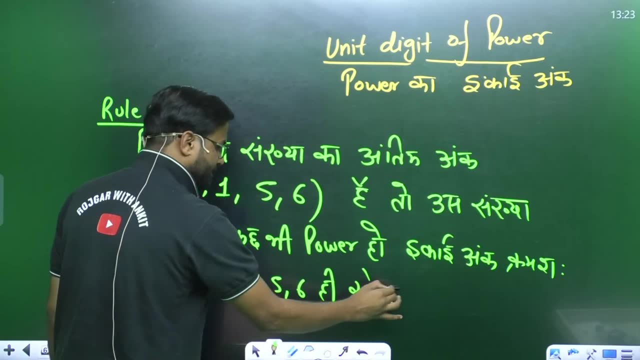 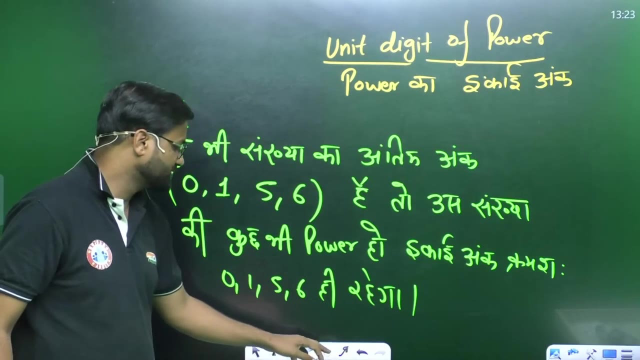 all of this will be written as a number of circle, from the circle what will be? 0,, 1,, 5, and 6,. this is the very important lines I have written. it will remain the same. sir. I have written this statement. tell me some examples on it. 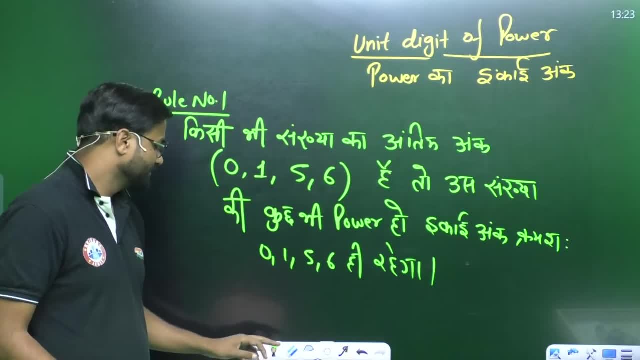 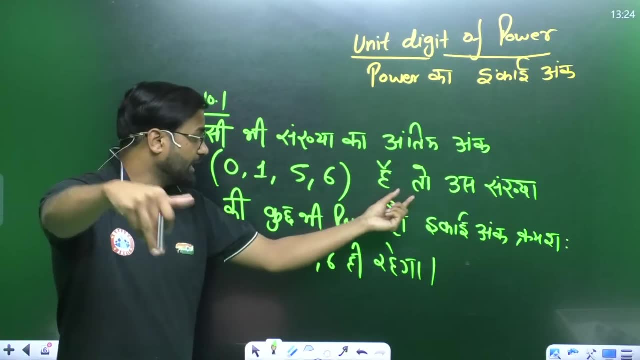 there are a lot of questions on your mind. first write it properly. if there is any number's last number- 0,, 1,, 5, and 6, if there is, then its No matter what. no matter what the power of the world is, except for zero. 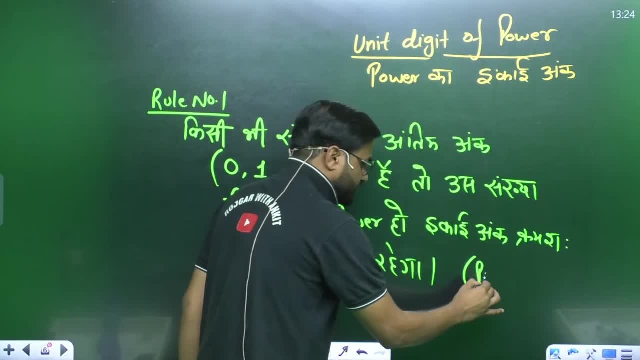 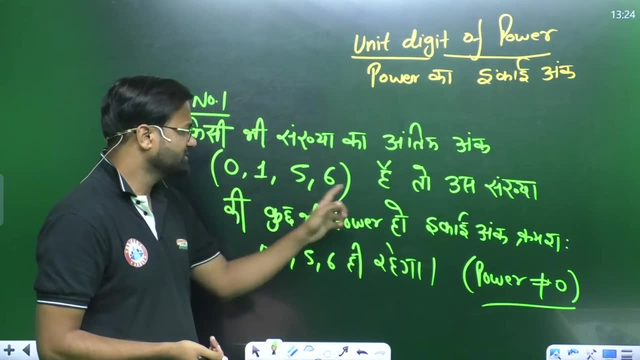 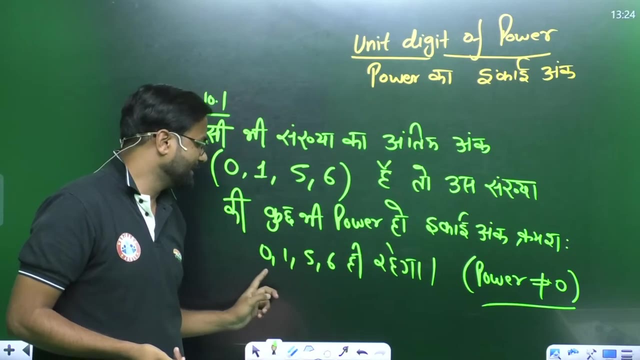 except for zero. the power should not be equal to zero. I will tell you the importance of zero. If the last number of any number is 0,, 1,, 5,, 6,, then no matter what the power of that number is. 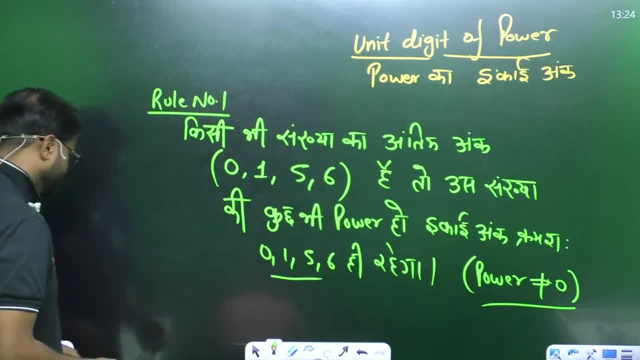 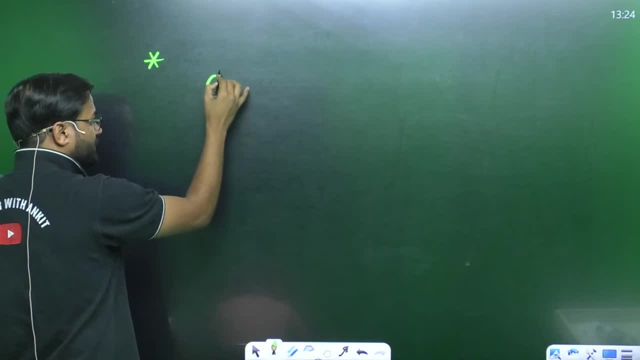 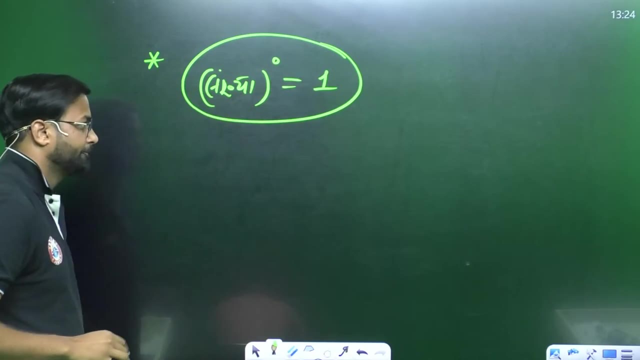 the first number will always remain the same. The power should not be zero. Why? Why should the power not be zero? Write it down For any number. take any number. take any number. if its power is 0, its answer is always 1.. 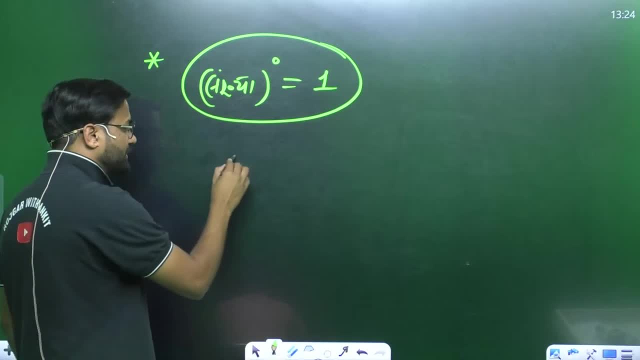 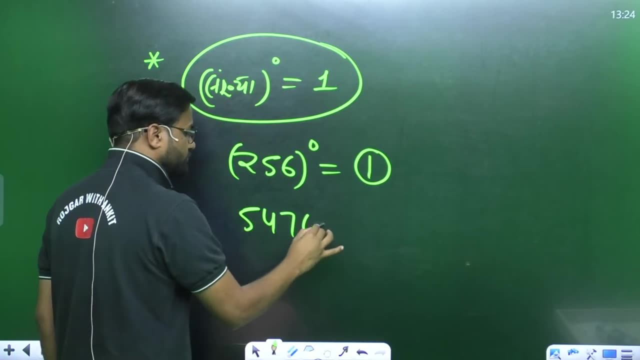 That's why Take any number of the world. I took 256, its power is 0,. answer is 1.. I took 547, 4, 6, 0, its power is 0, answer is 1.. 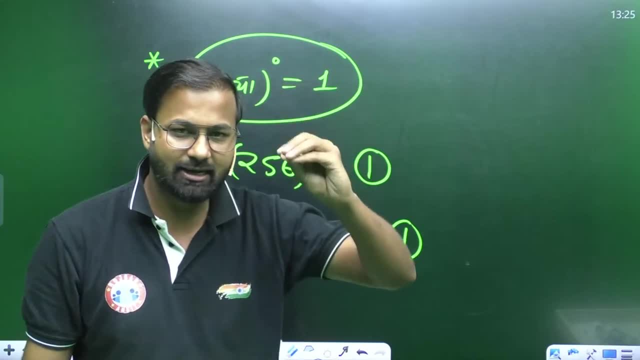 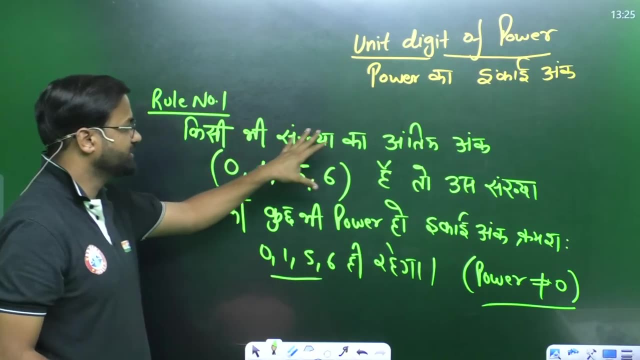 Always, If there is a zero on someone's head, then the answer will be 1.. You have to keep this clear. So in our statement this concept is clear. What is the statement If the last number of any number is 0,, 1,, 5,, 6,? 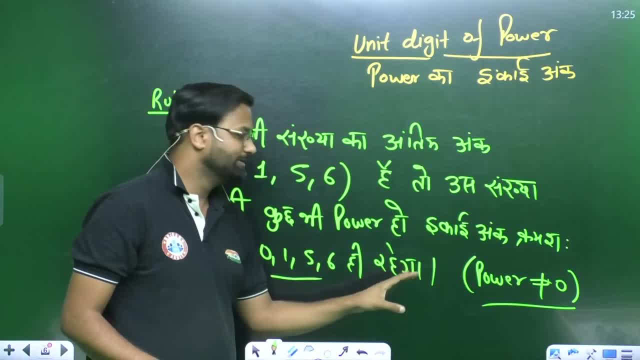 then, no matter what the power of that number is, the first number will always remain 0,, 1,, 5,, 6.. the first number will always remain 0,, 1,, 5,, 6.. the first number will always remain 0,, 1,, 5,, 6.. 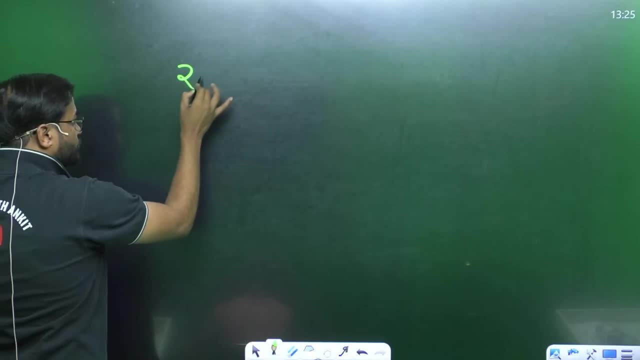 Now I will give you an example. For example, I said 2,, 3,, 5.. Its power is 4, 2,, 9,, 6, 2.. Its power is 4,, 2,, 9,, 6,, 2.. 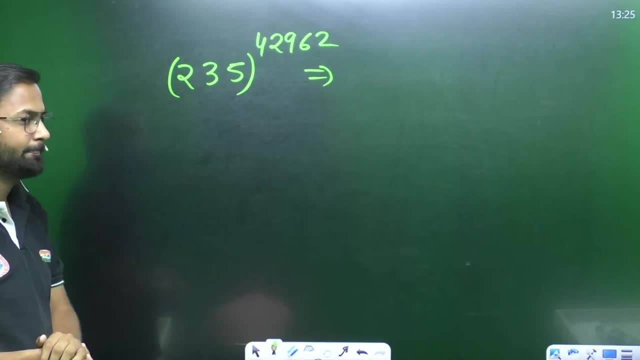 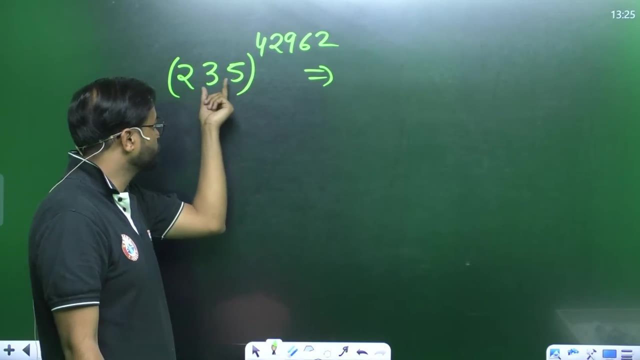 What will be its unit digit? What will be its unit digit? Can you tell me? Don't insult me. Tell me the answer quickly. I said 235's power is 42,962.. I said 235's power is 42,962.. 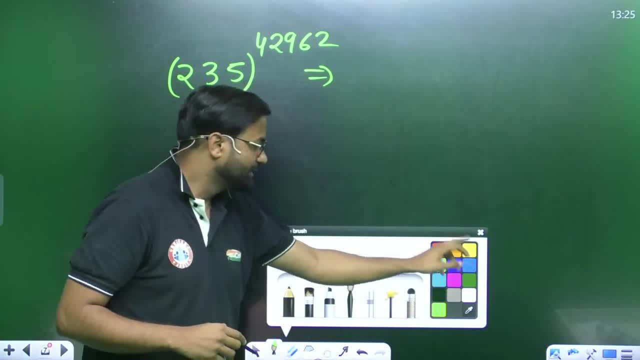 Sir, how do I get it out? I just told you that the last number of any number, if there is 0,, 1,, 5,, 6,. if there is 0,, 1,, 5,, 6,. 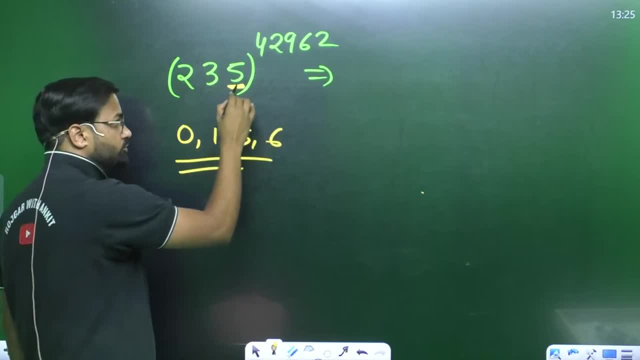 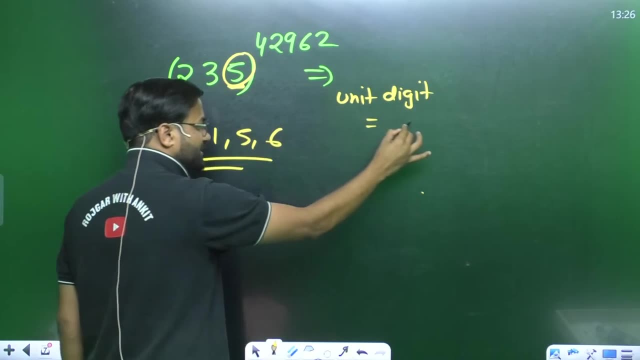 if there is 0,, 1,, 5,, 6,, then, regardless of its world power, what will be its unit digit? The unit digit will always remain the same number. The unit digit will always remain the same number. The unit digit will always remain the same number. 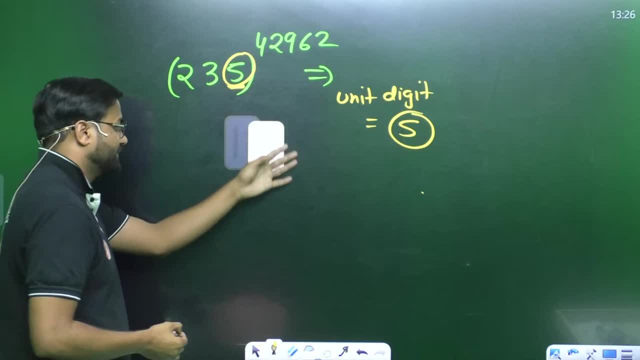 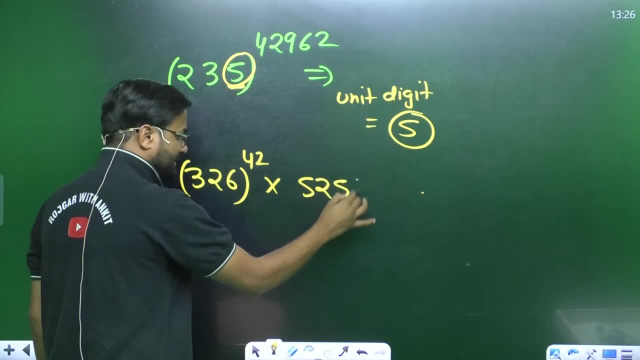 And your answer will be 5.. Wow. Another question. I said 326's power is 42, times 525's power is 43. times 525's power is 43. Tell me quickly what will be its unit digit. 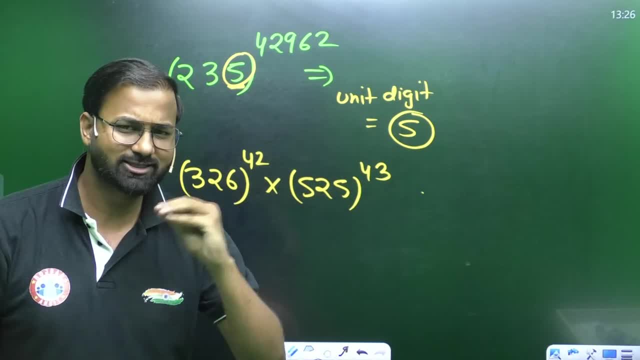 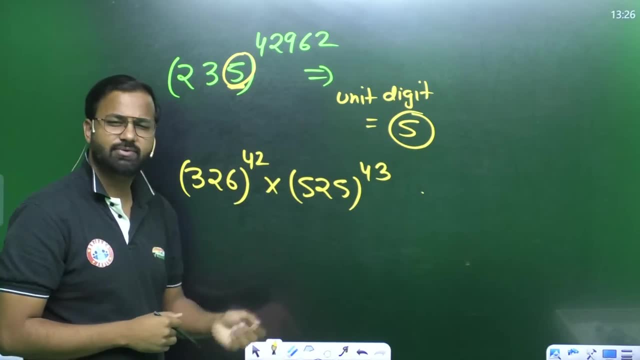 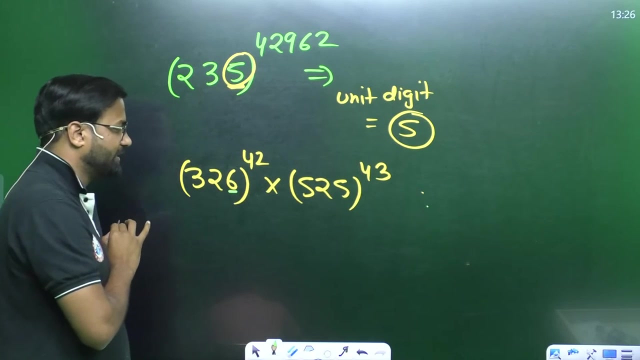 What will be its unit digit? Many concepts are slowly becoming a theory in the mind. I can't believe it. when you look at the question in the book, These are also asked by me. You will ask many questions in some time Now here. I knew it is a 6's power. 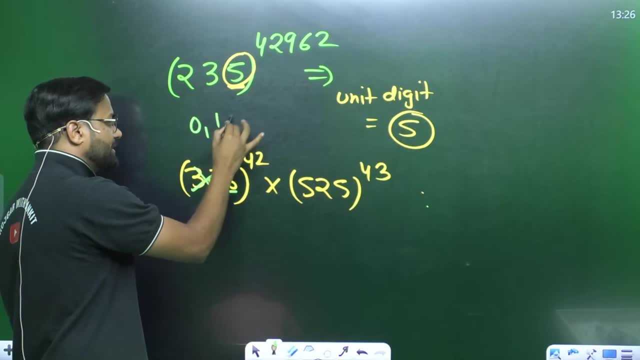 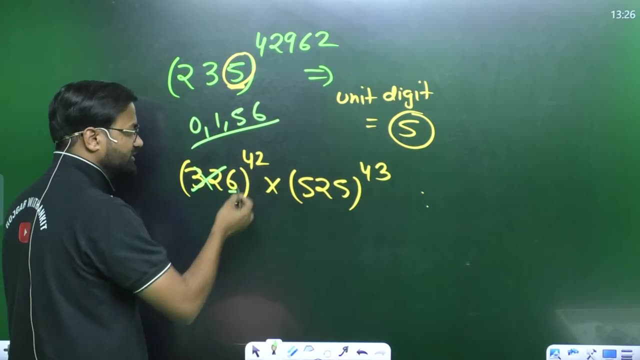 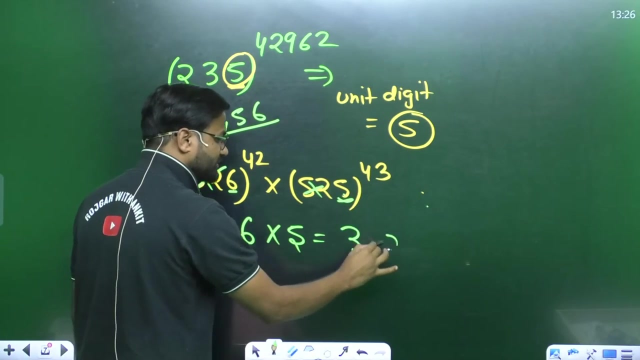 no matter what真ally, I told you 0.. 1.. 5 and 6.. Will you smile slightly and give it the answer? You will know it is a 6's power. Will you smile slightly and know that 5's power? 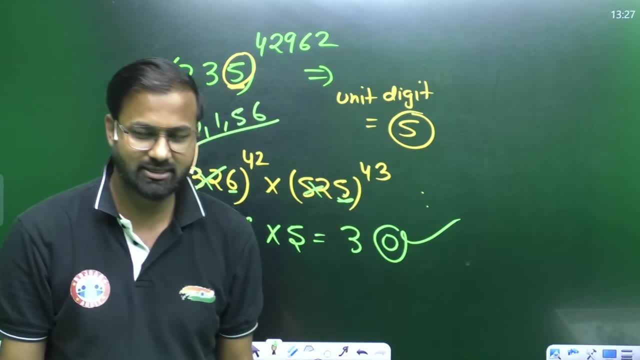 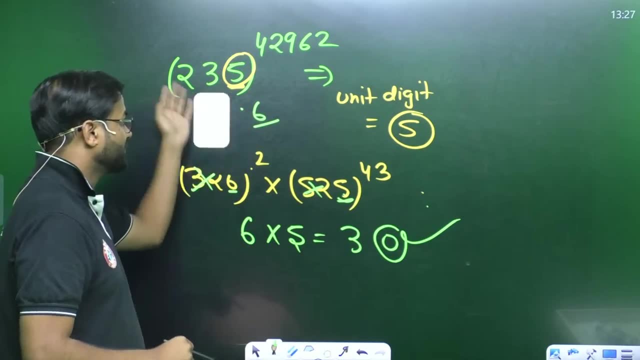 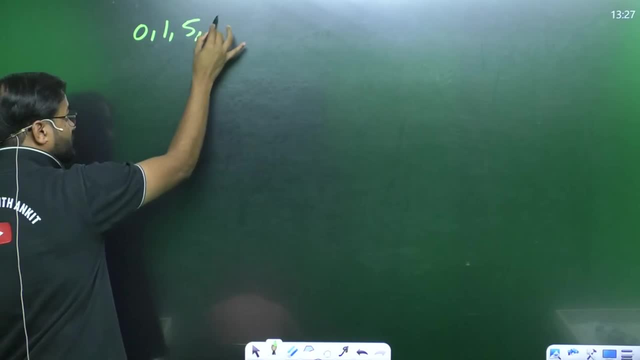 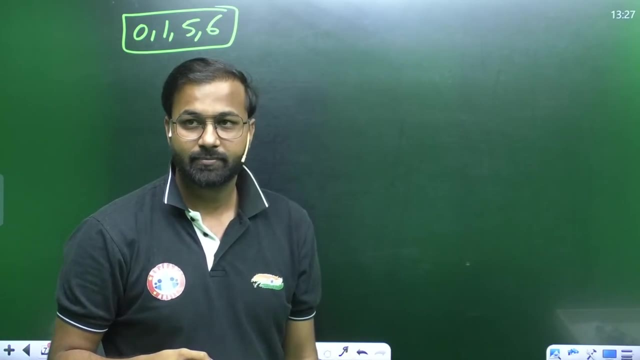 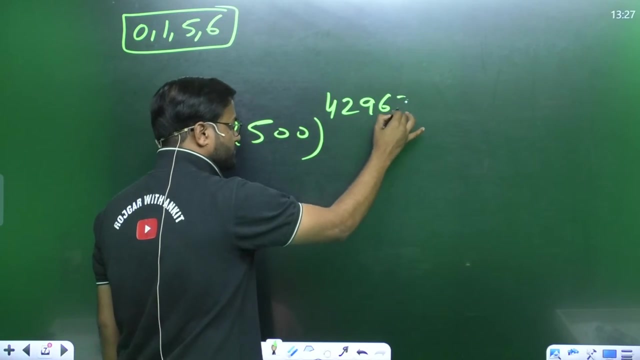 Who just had our power case: Zero one, five and six. Now, sir, what if there is more power than this One, zero, Okay, wow, very good. Power of 2500, if you said 4,, 2,, 9,, 6,, 2,, 3.. 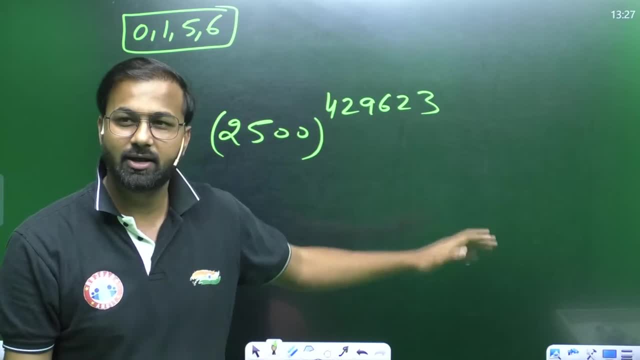 What will be the unit digit? Tell me. one kid said: sir, please do the zero one more time. Tell me, brother, what will happen Quickly, Okay. one kid said zero, so I didn't even write the number. 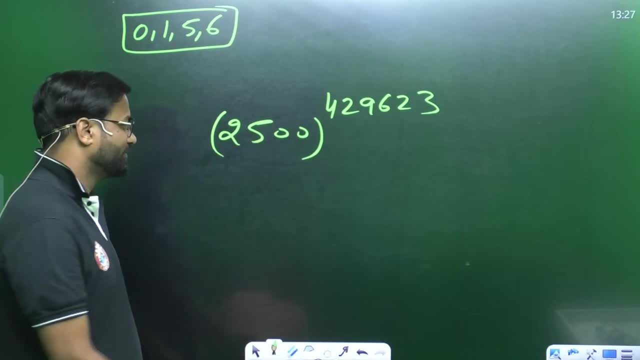 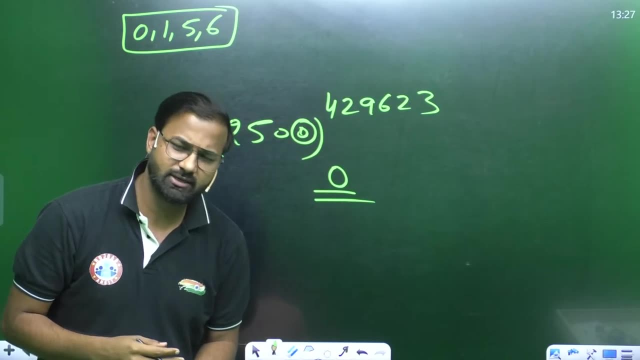 So many answers came: zero, zero, zero, zero. Oh man, you are very good. The last digit is zero. whatever power is there, the unit digit will remain zero. What will be the unit digit? It will remain zero. 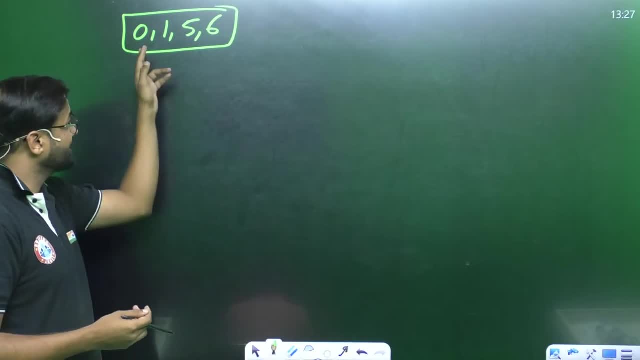 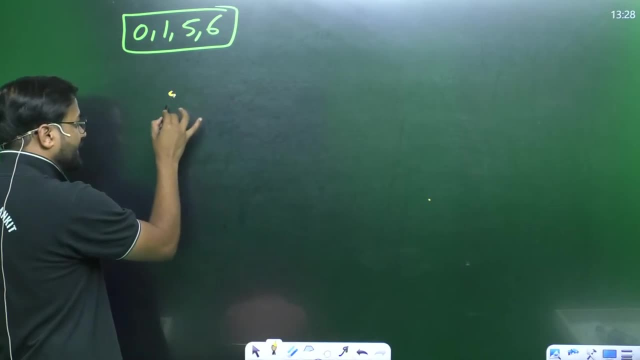 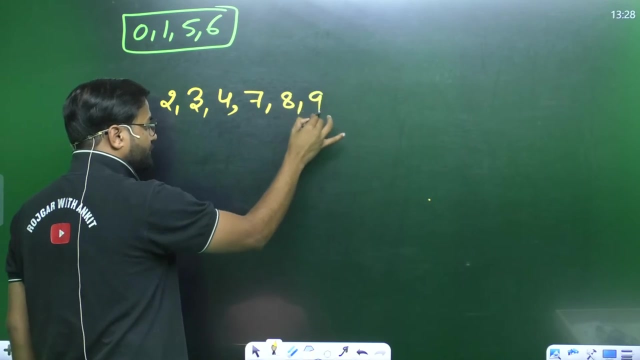 The matter is over, Okay, Okay. So Next, If, sir, there is anything other than this, zero, one, five, six, whatever it is, the unit digit can be two, three, four, seven, eight, nine. 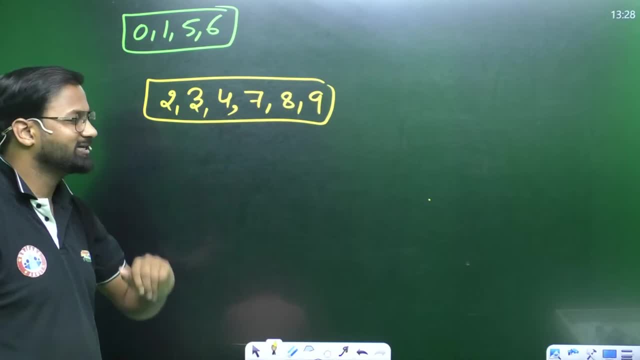 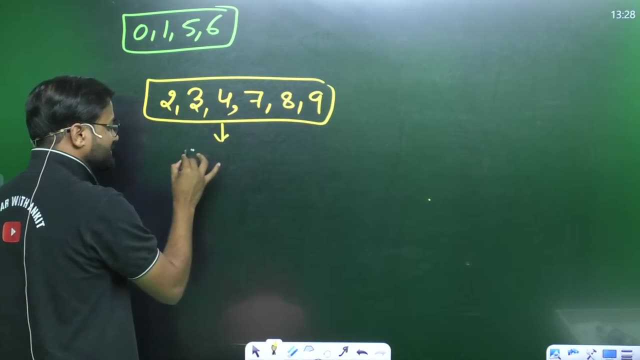 These are also numbers. These are also numbers Two, three, four, seven, eight, nine. What about these? I will tell you the treatment of these too. The concept of cyclicity is for their treatment. What is the concept of cyclicity? 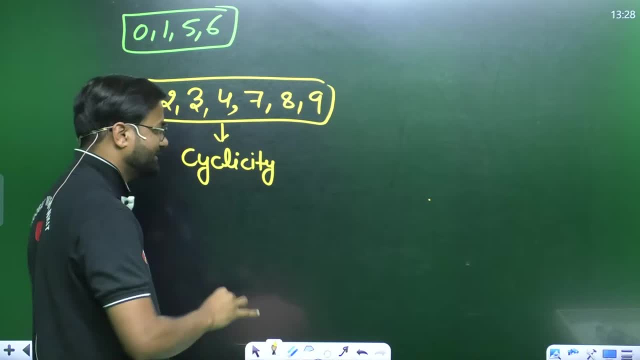 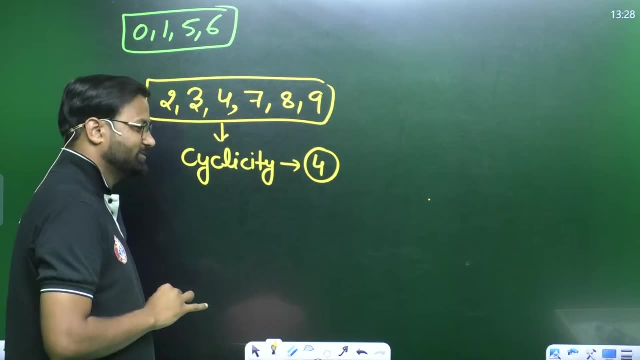 The concept of cyclicity is called circular concept. Okay, The concept of cyclicity is called circular concept. What is the concept of cyclicity? It is of four. How is it, Sir? Is it retro? No, I will prove it. 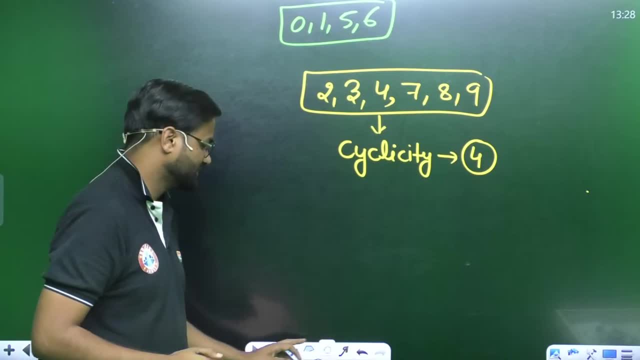 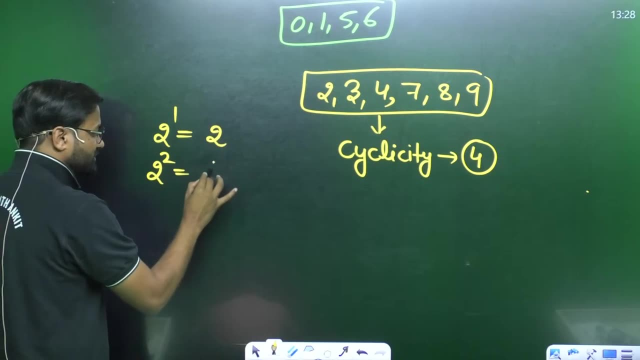 If someone had to use cyclicity, then how does it have four? Tell me something: What is the power of two? Two? What is the power of two? How much is 2? 4? How much is 2's power? 3? 8? 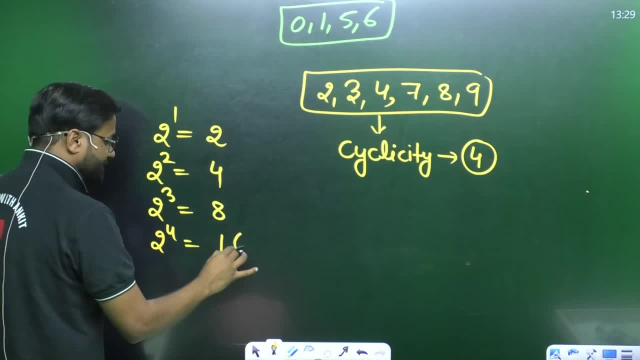 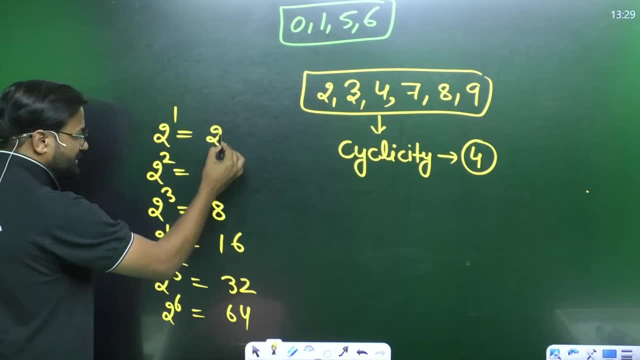 How much is 2's power 4? 16? How much is 2's power 5? 32? How much is 2's power 6? 64? Tell me one thing: when did this last digit start repeating? 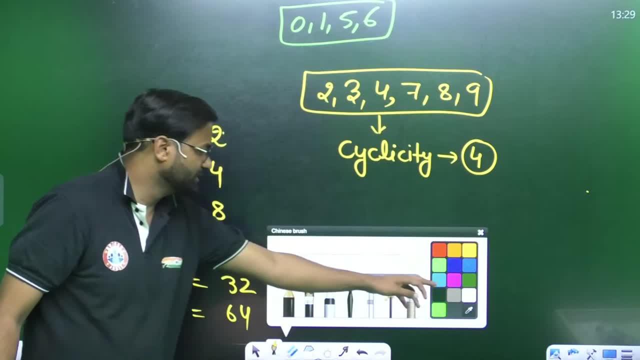 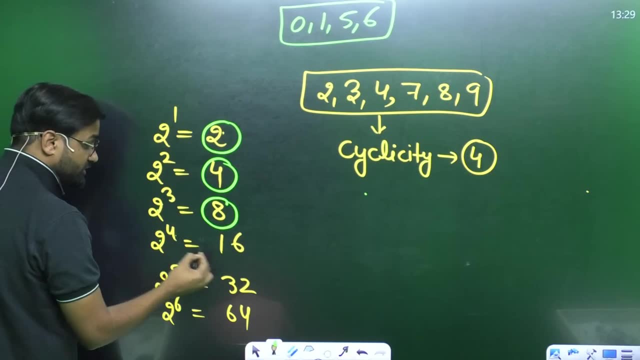 When did this repeat? start repeating. You saw that 2's power is 1,, 2, 2's power is 2, 4. 2's power is 3,, 8 Till 2's power is 4,. all the numbers were different. 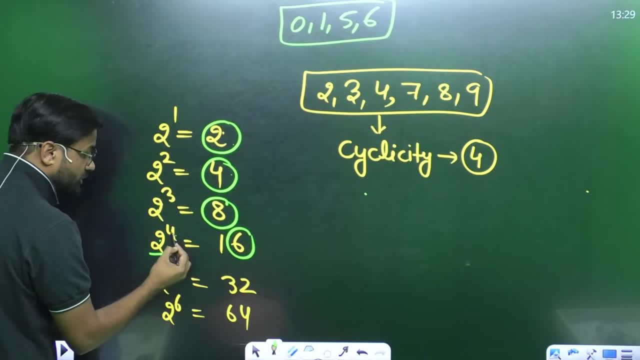 Look at the front. Till 2's power is 4,, all the numbers were different. But as soon as 2's power is 5, 2 again started. Then 2's power is 6, then 4 came. If you do 2's power 7, it becomes 128. 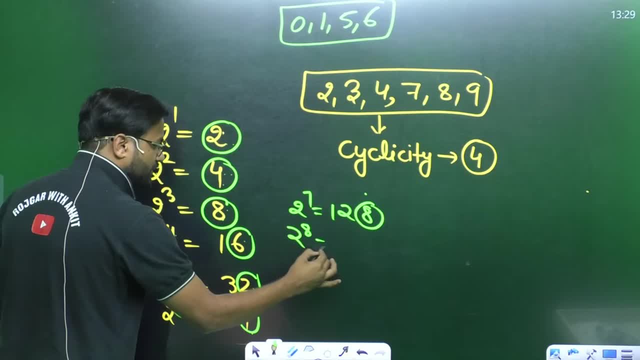 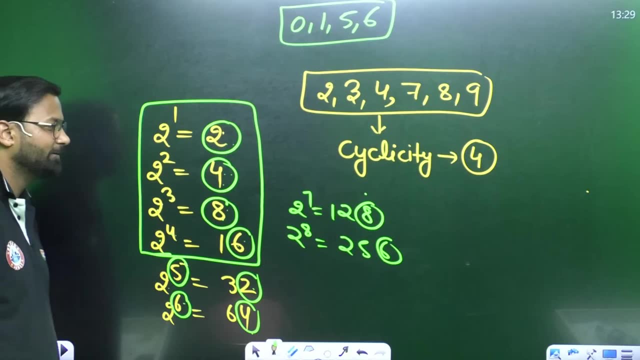 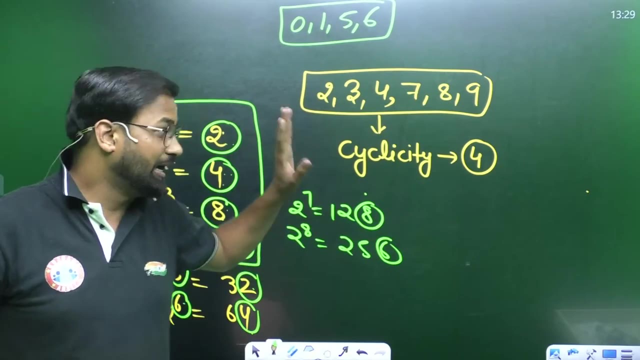 Then 8 came. If you do 2's power 8, it becomes 256. Then 6 came. That means the number of numbers that came separately, That came separately, The power of 2 came up to 4. That means That means Brother. let me tell you something. 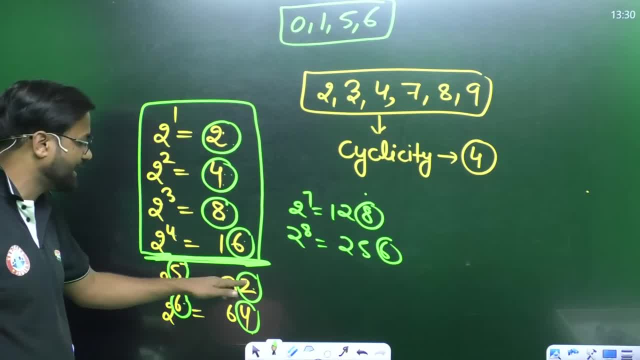 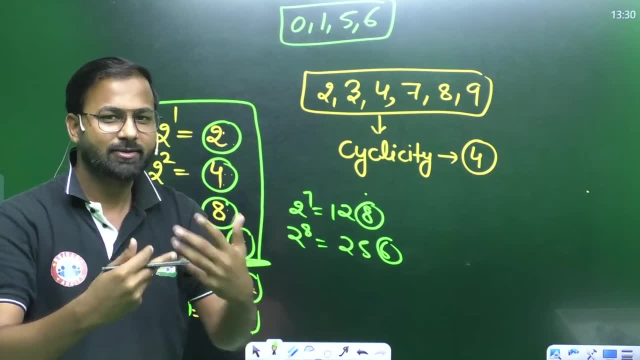 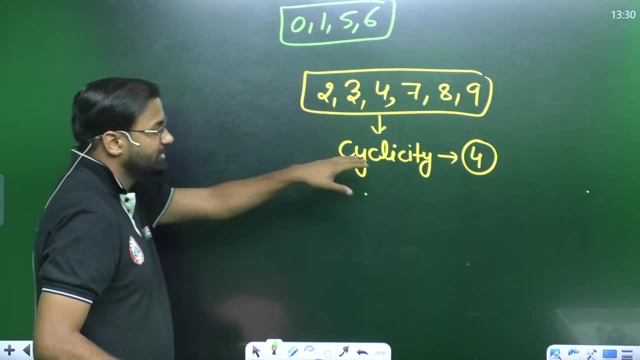 Cyclicity happens because after 4, the unit digits start repeating themselves, They start rotating the number of 1's, So cyclicity happens after 4. I told you this concept. Now, the concept of this cyclicity is not necessary, That these 2,, 3,, 4, 7, 8 numbers are not necessary. 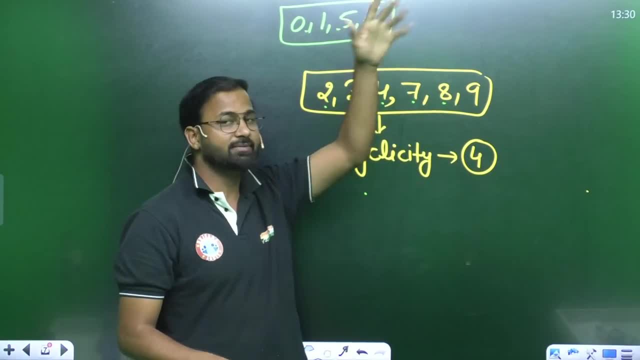 That these 2,, 3,, 4,, 7,, 8, 9 numbers are necessary. Brother, you can put them in 0,, 1,, 5, 6. This is a universal concept. What did I say? This is a universal concept. 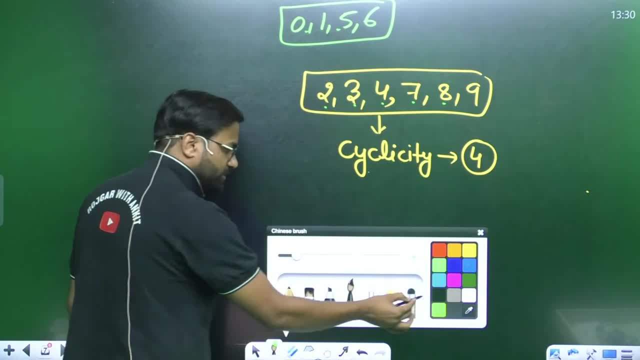 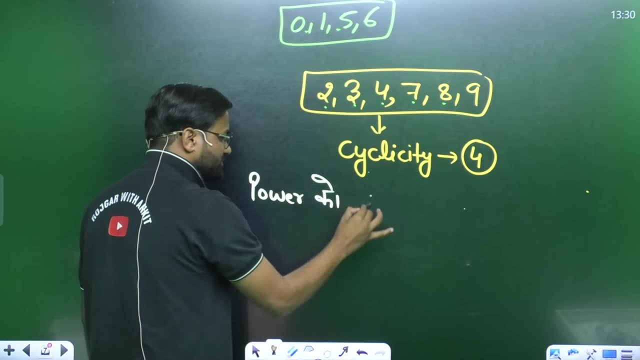 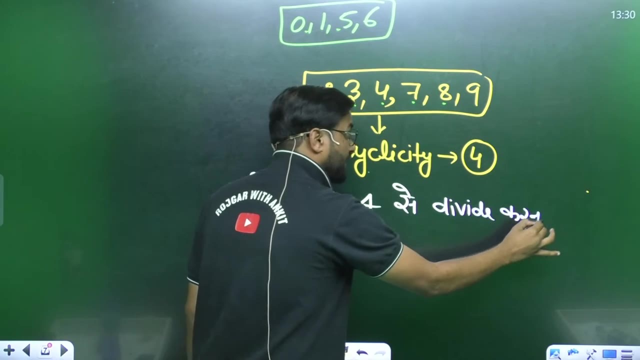 So here, the cyclicity is 4. For that, what will you do? I will give you a topic. What you have to do is Power, Power. You have to divide it from 4. You have to divide it from 4. You have to divide power from 4. 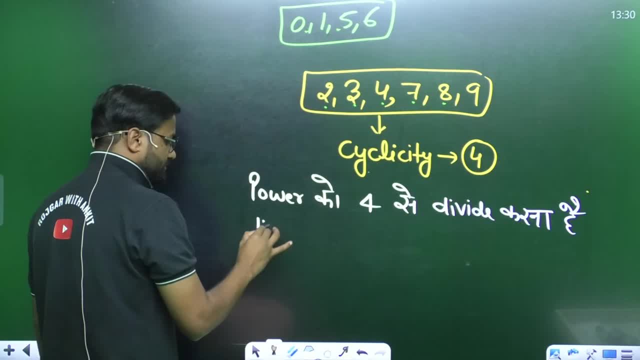 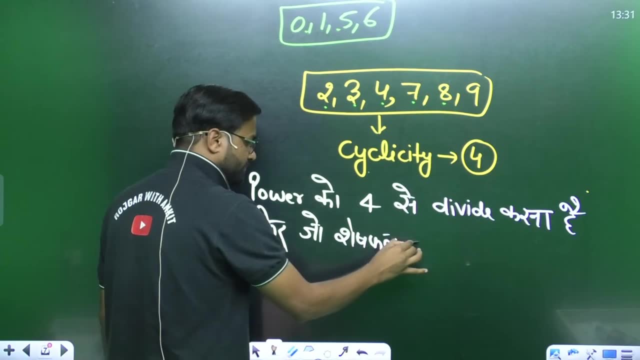 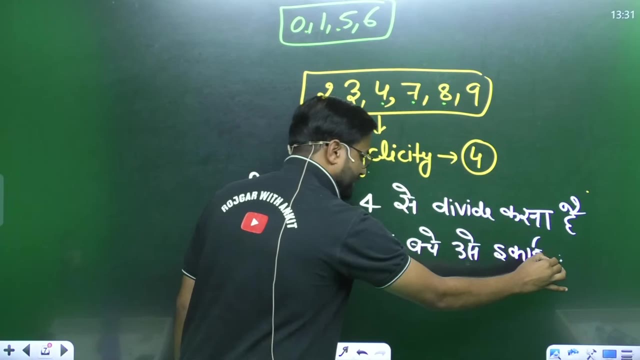 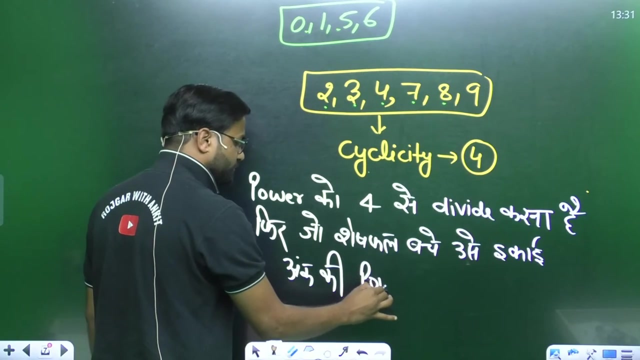 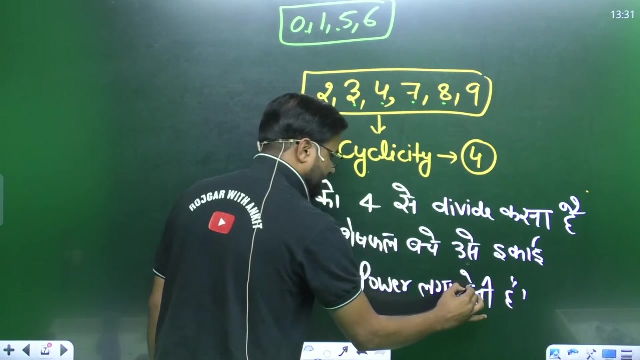 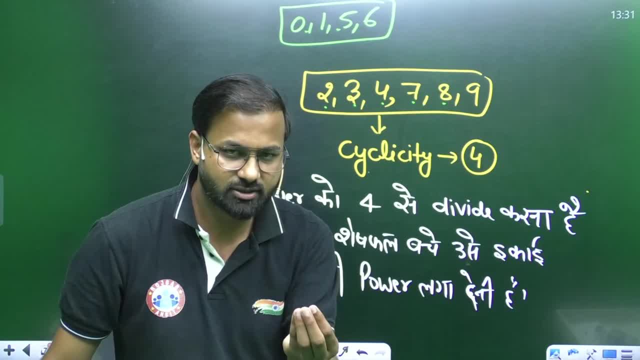 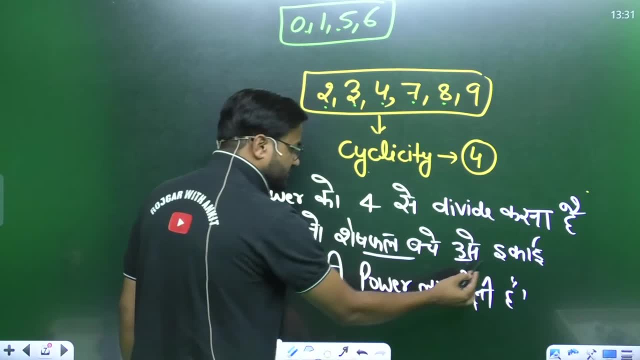 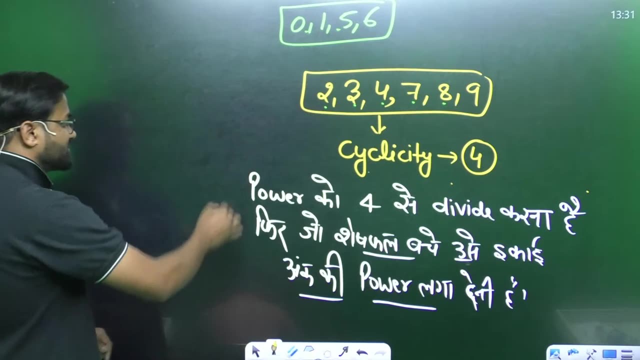 you can divide it by 4.. Yes, sir, you can. You have to divide the power by 4.. Then the remaining number of the number 1 has to be given power of the number 1.. Okay, Yes, make one star in this. 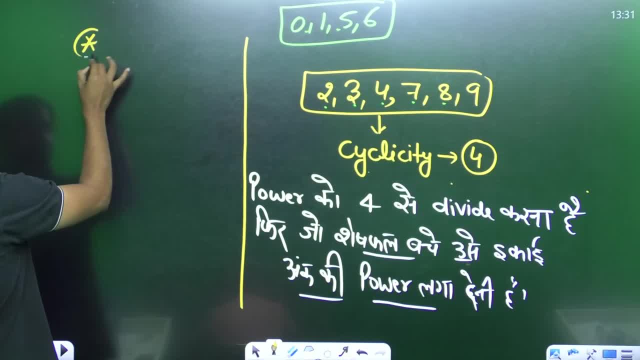 and write one more concept. I will do it for the sake of example: If the power comes to 4, the remaining number? if the remaining number comes to 4. You have to divide it by 4, but if the remaining number 0 comes, 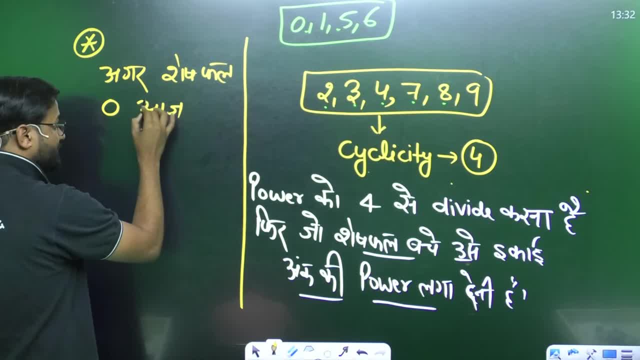 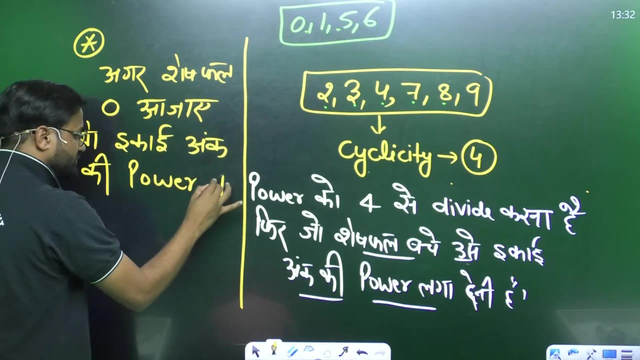 if the number is completely cut, then you do not have to put power 0. If the remaining number comes to 0, then the power of the number 1, the power of the number 1 will be 4.. Let's do it. 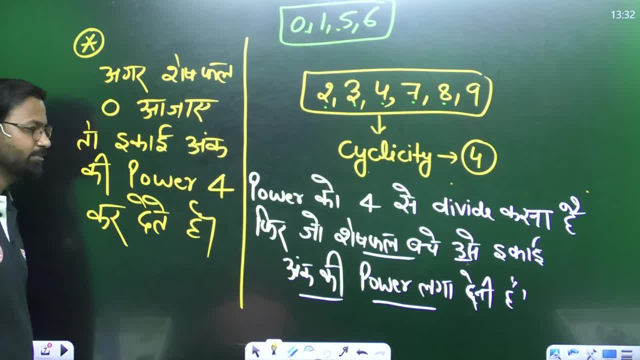 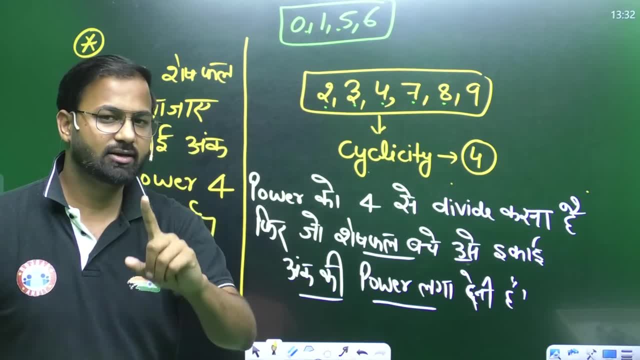 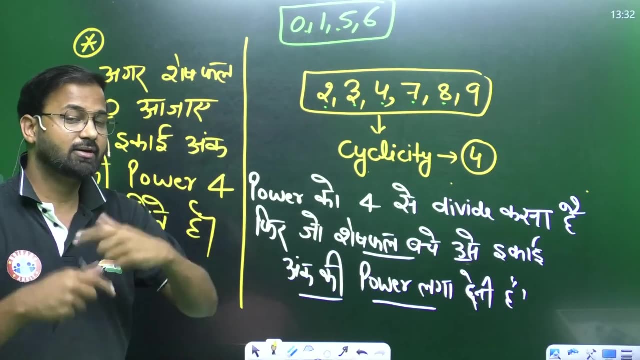 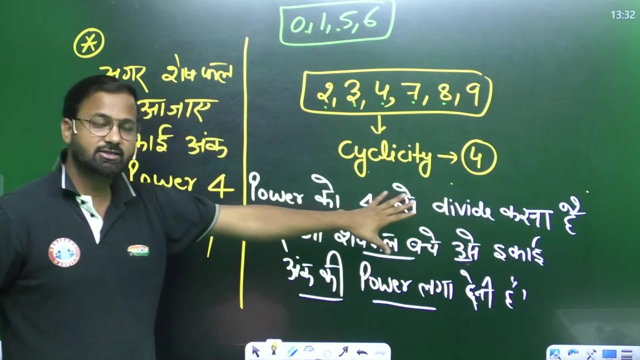 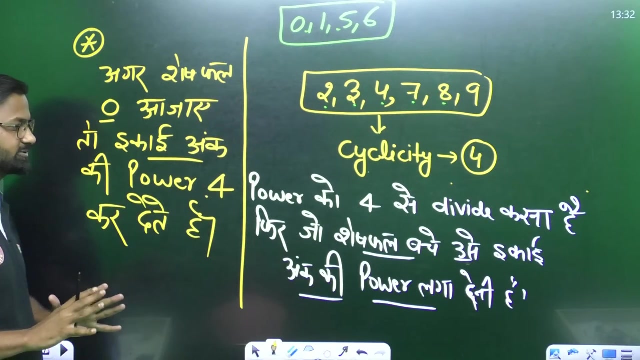 I would have asked you to write this question directly, but if we want to remember something for a long time, then we should have short notes in this way so that we can recall things very well. We have to divide the power by 4,. we have to apply the power of 1 to the rest of the results. if the result is 0, then we will divide the power of 1 by 4.. 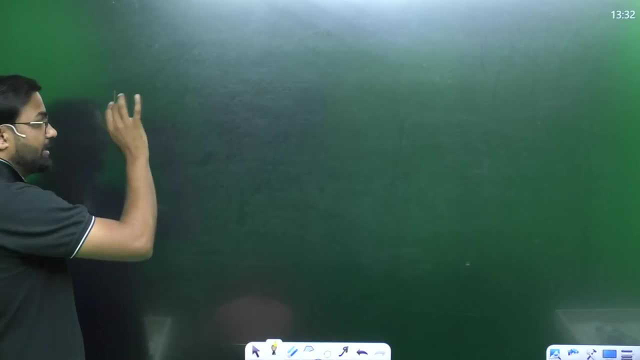 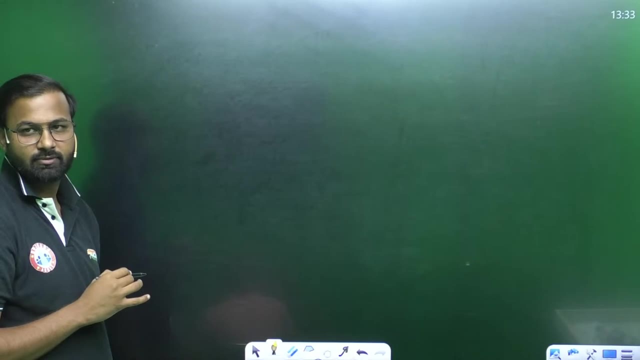 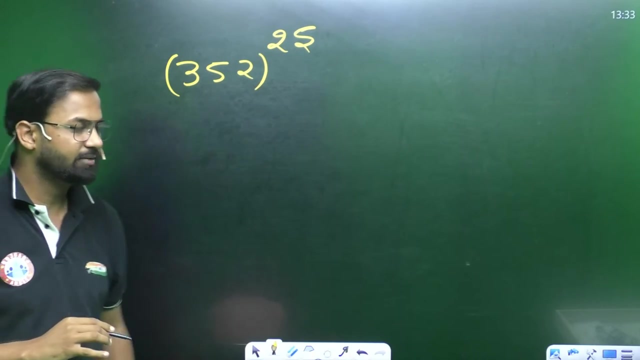 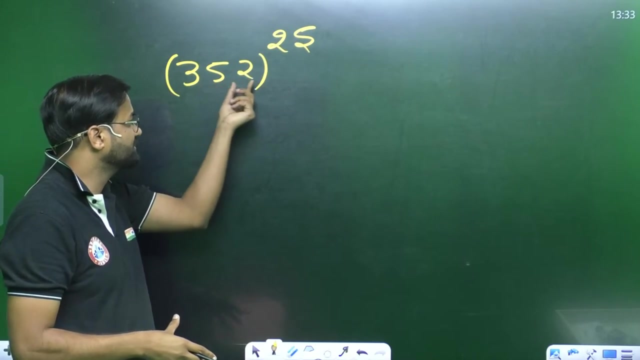 Now let's do an example. How did the video stop here? Is the class going well? I will give you a question. 352 and its power is 25.. Tell me quickly, how will we do things in this number? Power of 352.. 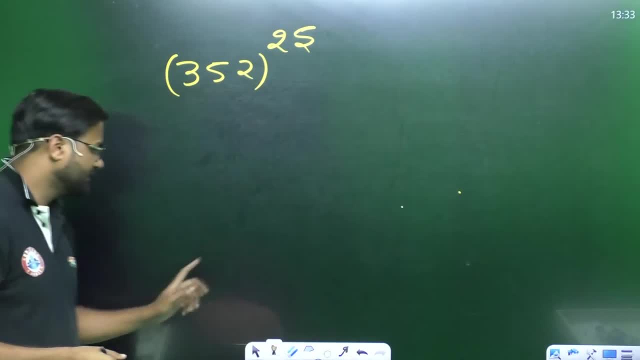 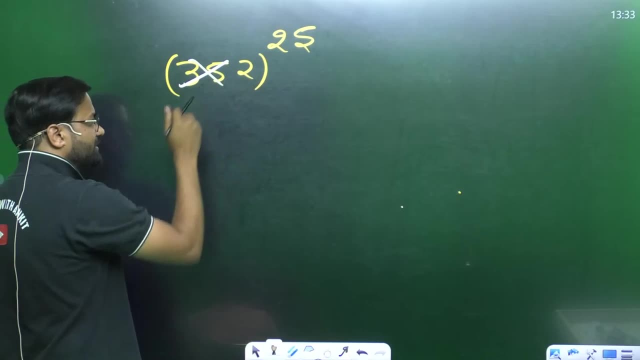 Is it 25?? What concept did I tell you just now? I told you that power is divided by 4, the rest of the results, It has the power of 1.. Don't get stuck in this mess. What number do we have? 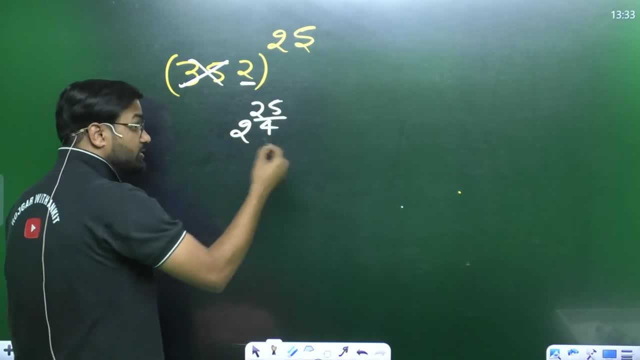 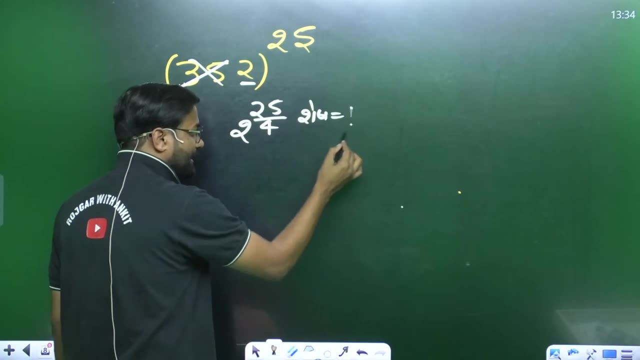 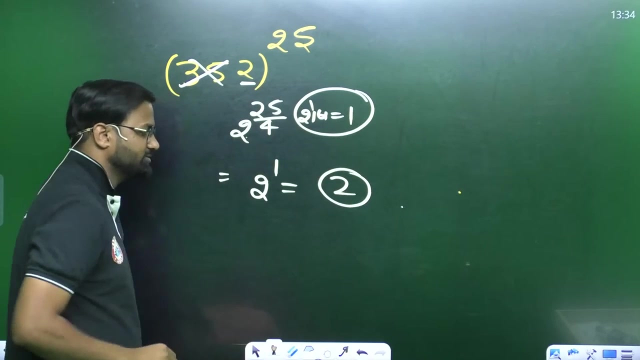 The power of 2 is 25.. Divide 25 by 4. How much will it come Remainder? How much will it come? Charging is 24.. Remainder, The result is 1.. This is your answer. You have the answer. 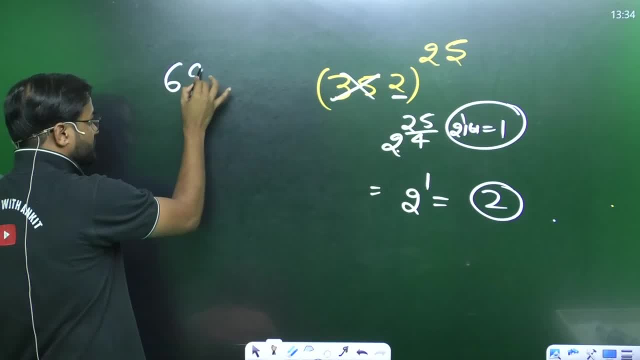 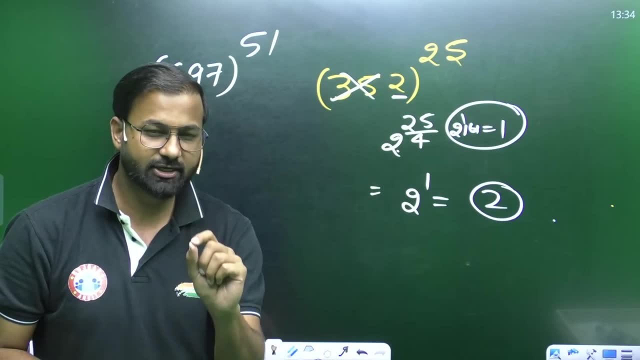 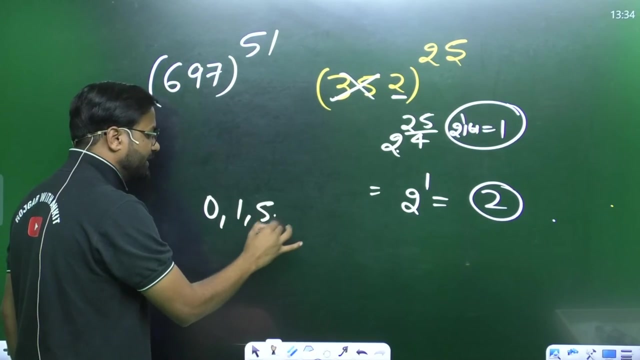 I will ask you another question. I said 697 and its power is 51.. Tell me quickly, how will it come? Its power is 51.. What is your answer? It is 7 and we have read 0,15 and X. 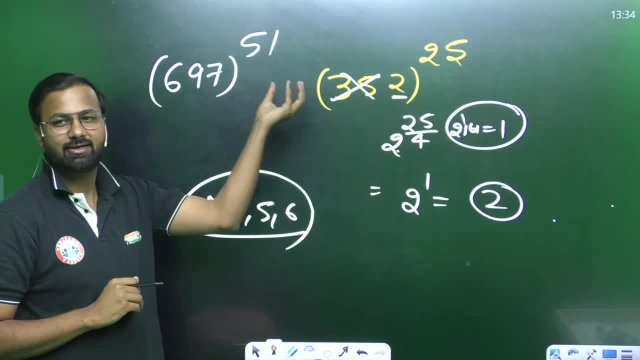 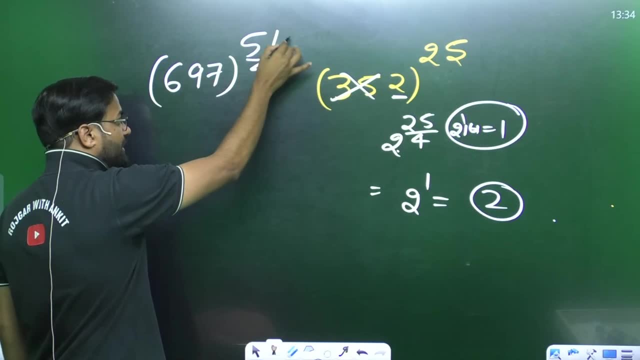 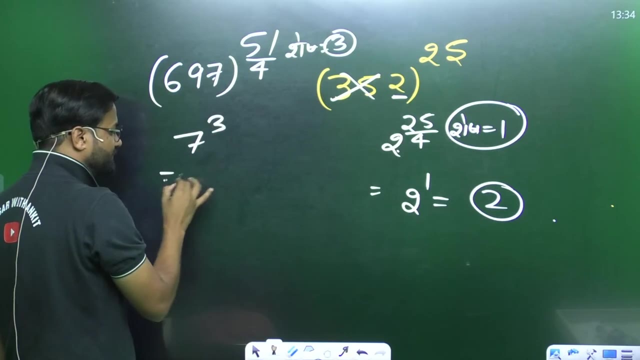 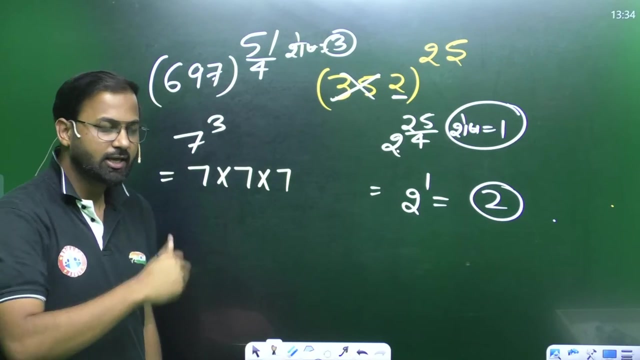 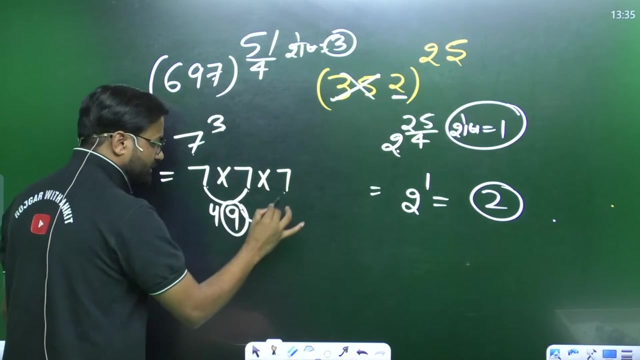 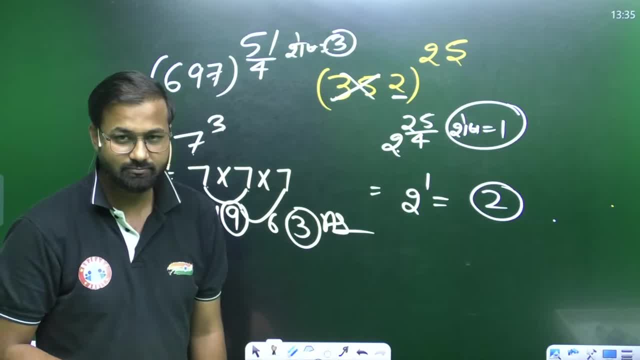 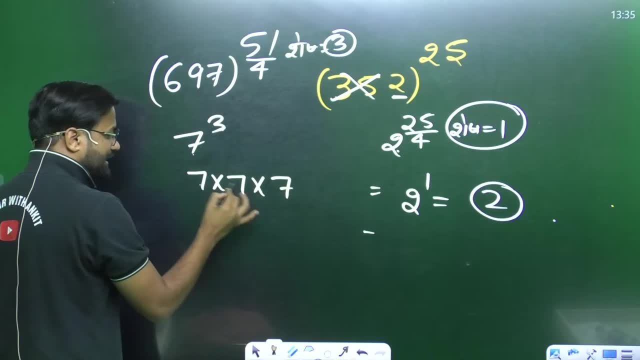 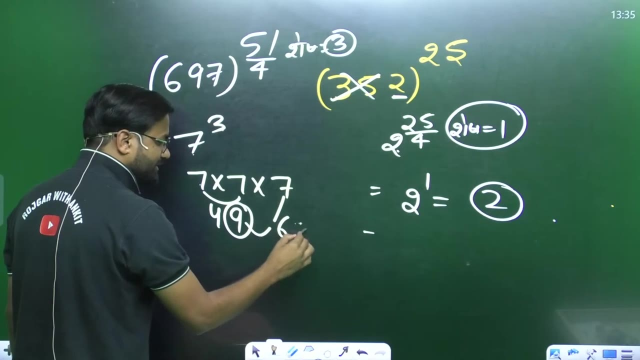 How did I do it? I got 7 power 3, so I wrote it like this: 7 times 7 times 7,, so 7 times 7 is 49,. take its unit digit 9 times 7 is 9 times 7,, so 9 times 7 is 63, and 63 times 3 is your answer. 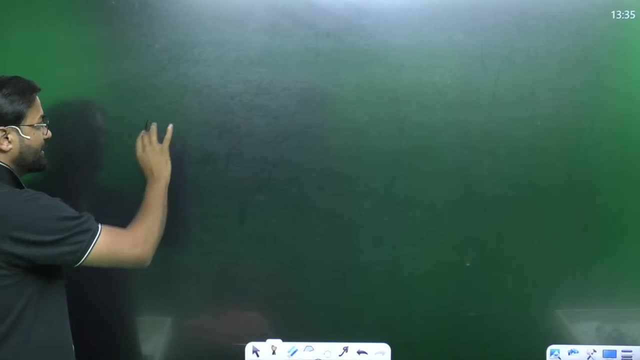 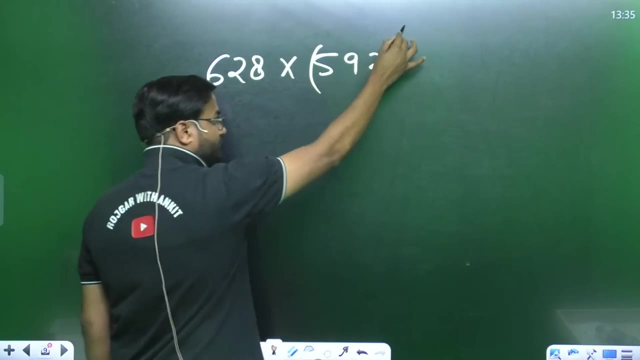 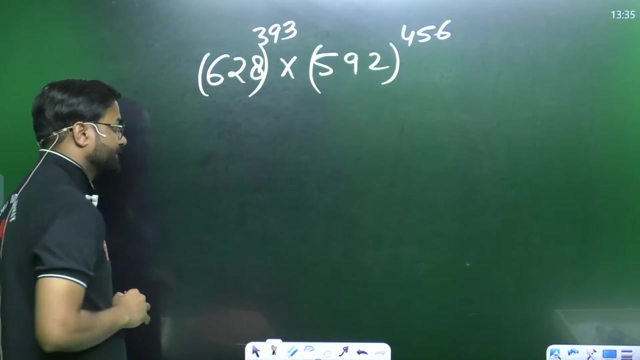 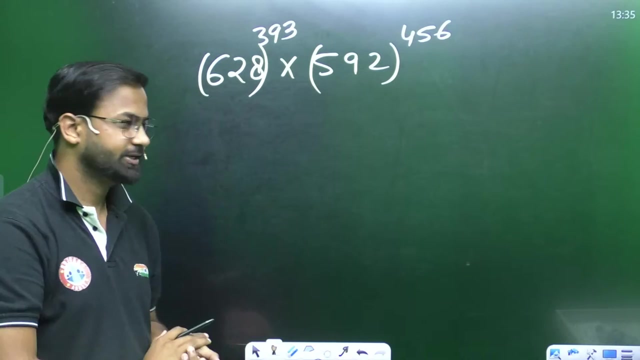 Done. Okay, I will give you one more question. I said 628 times 592.. Its power is 456, its power is 393,. now ask this question: how will this question be done? How will this question be done? Tell me. 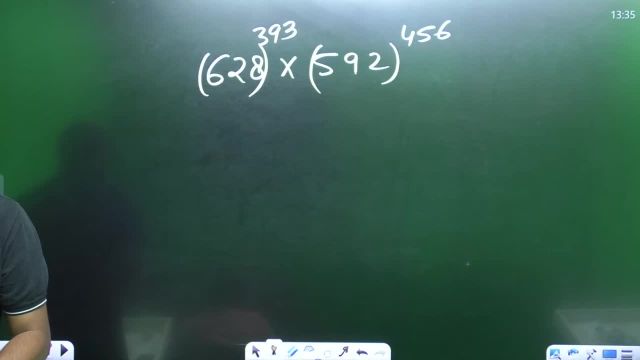 Put your mind to it. who will get the most answer? who will get the first answer? Let's talk. we are at 8, I want to fix the problems I have. I will divide the power into 4, now listen to me. 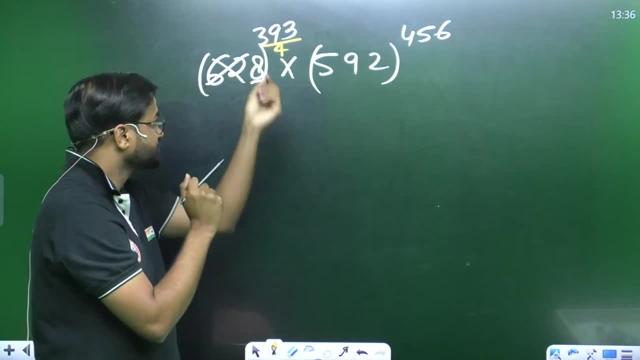 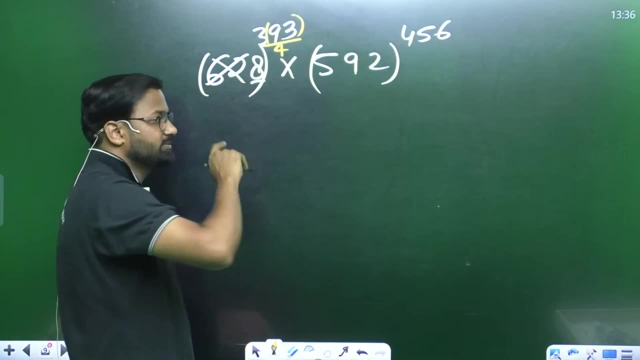 Listen to me. let me see your picture first and see on screen. Don't divide 493 with 4, the last two digits need to be divided, the divisibility of 4, And we will read the divisibility rule: Medienoka Vibhajeta. 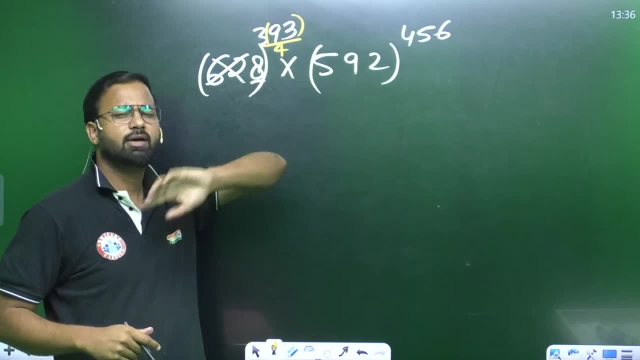 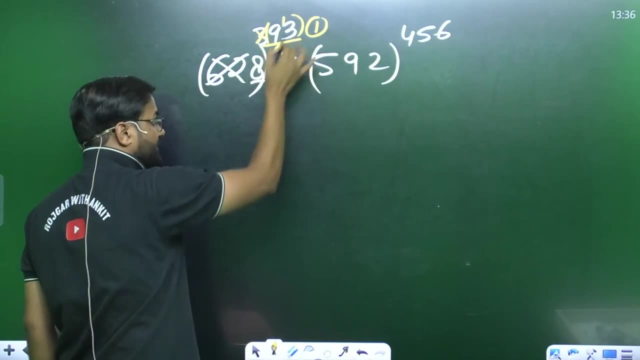 Vibhajeta of 4, it's five gigabit, third of last on the line Hold 4 because, as 10 Hold 93,. 93 does not mean 3, so 4 times 2 is 8,, 4 times 3 is 12, the final result is 1, so the power of 8 is 1.. 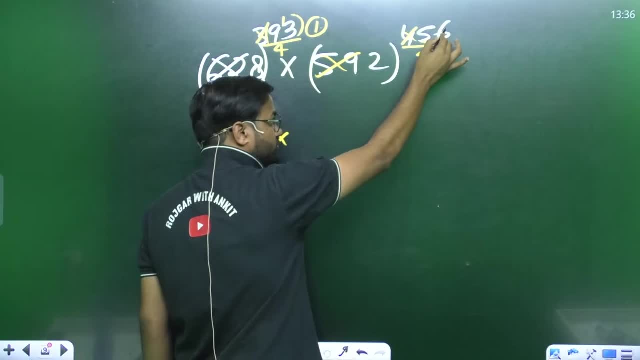 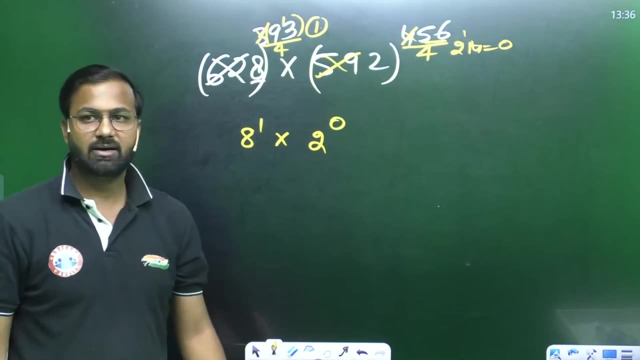 We will divide by 4, last 2 digits means 14,. 4 is 56,. it is completely cut. the final result is 0.. Oh sir, if the final result is 0, then will I keep the power of 2 as 0 here. 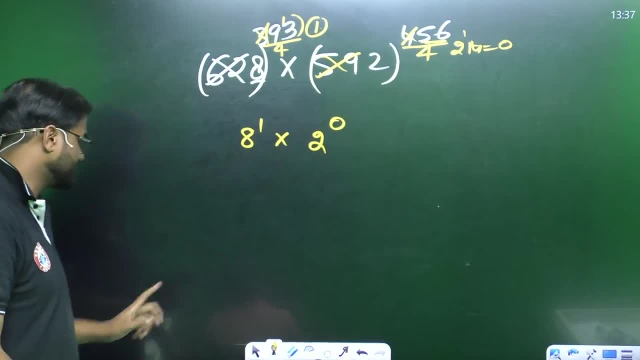 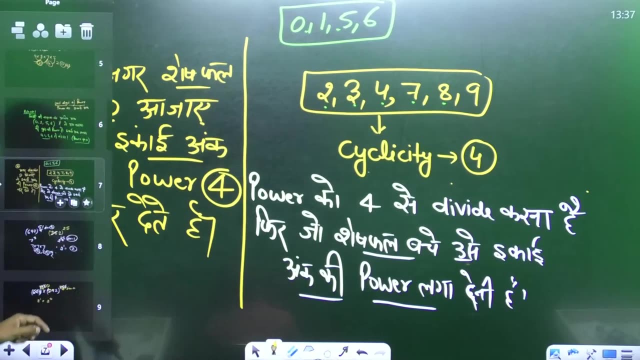 I said, if the final result is 0,. if the final result is 0- and this is also written in the special- if the final result is 0,, then how much is the power of the first number? the power of the first number is 4.. 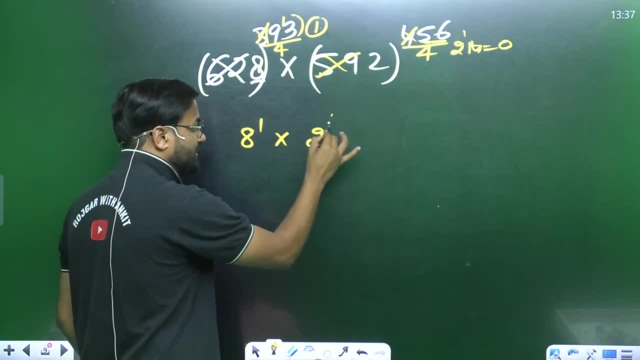 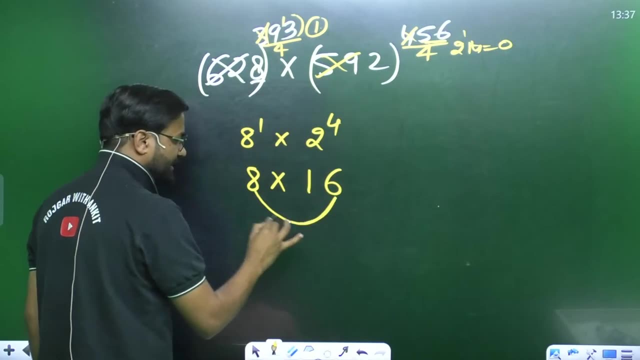 How much do we do? We do the power of the first number, 4, because the final result is 0.. So, children, 8 times 1 is 8, 2 times 4 is 16,. multiply by 6, 8 times 6 is 48,. the unit digit is 8, it is completely cut. 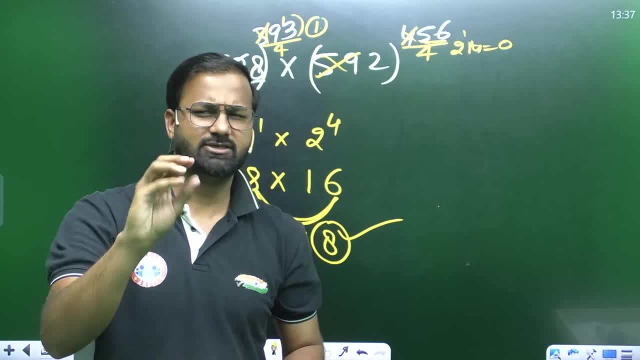 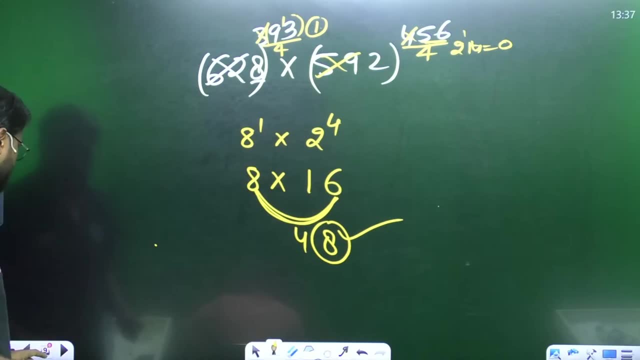 8 is here. let's go to the questions now. the factorial concept is left. What is the concept of 10 minutes? What is the concept of factorial of 10 minutes? There is nothing now. the main concept was this. now the lion is ready to ask questions. 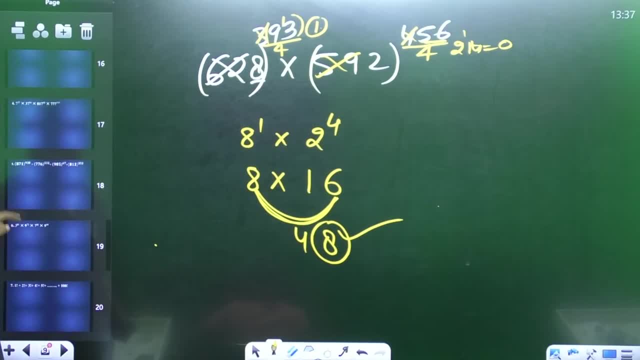 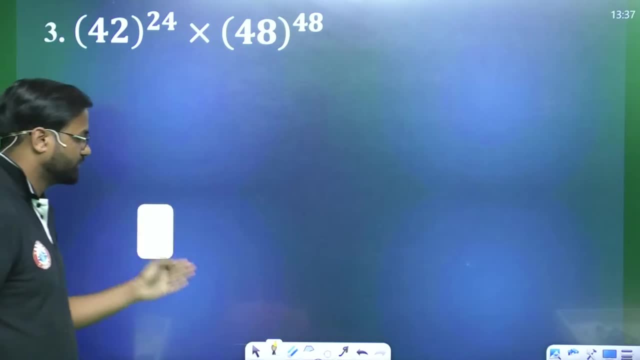 What will be the answer to this question? Which question, Which question? I don't feel hard for you. I am scared of the question. so tell me what will be the answer to this quickly. What will be the answer to this question, Will you tell? 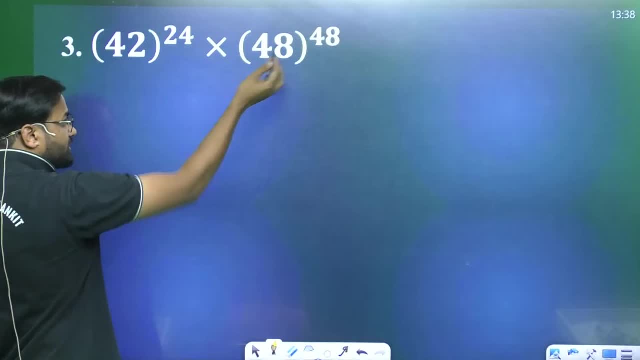 All people. what is the power of 42?? How will we do this question? We will do this question in this way, brother: we will divide by 2,, we will divide by 4,, 4 times 24,. the remainder came to 0.. 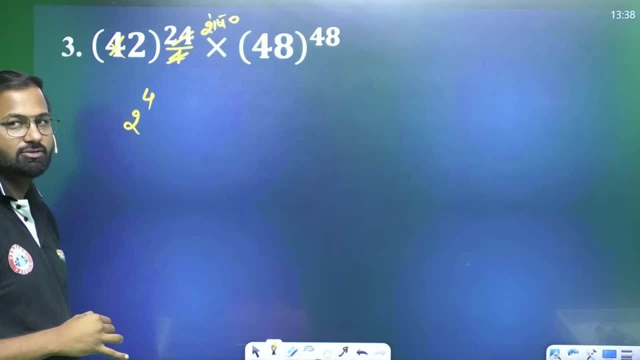 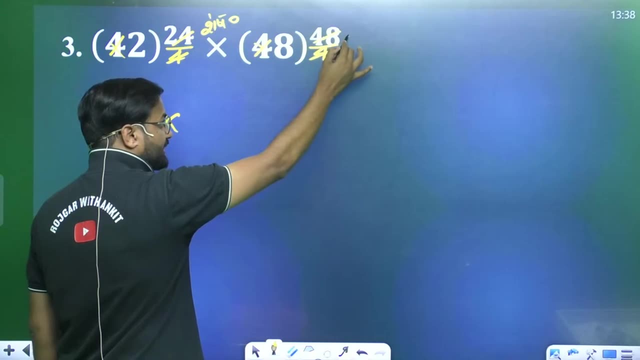 So, brother, here we will do the power of 2 in the case of 0,, we will do the power of 2 in the case of 4, now we will divide by 4, it is completely cut 12 times. the remainder came to 0, and on the remainder of 0,, the power of 8 will be 4.. 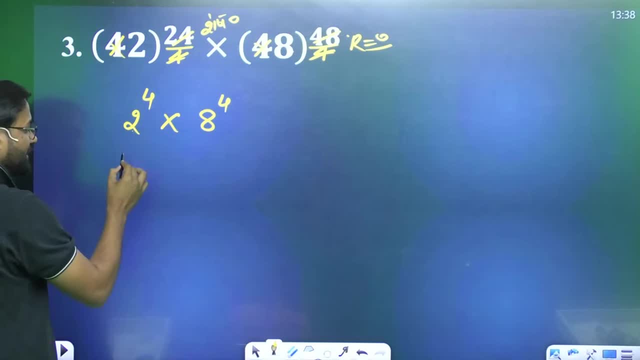 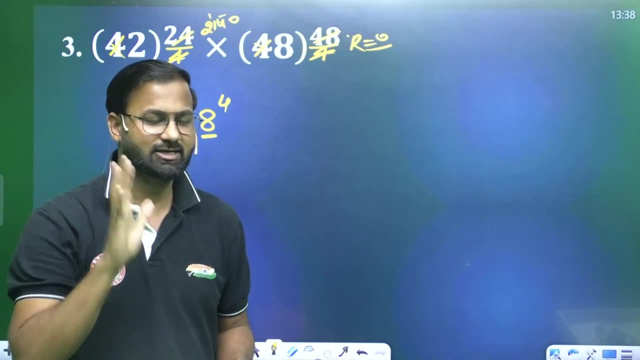 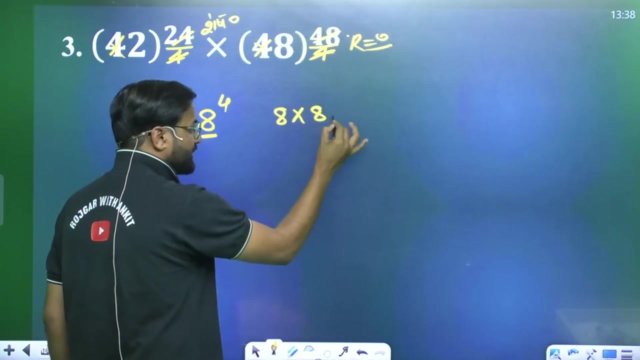 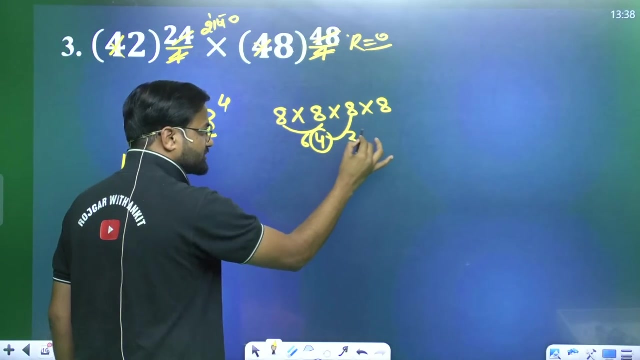 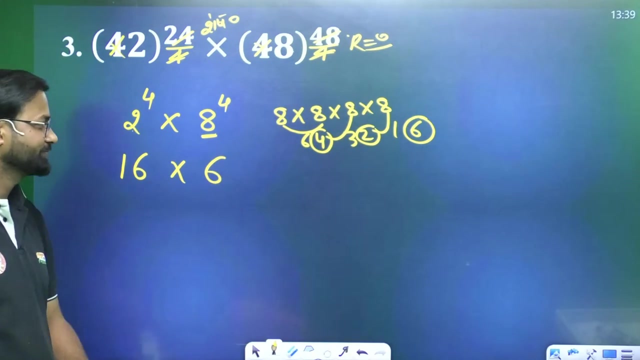 Will there be any problem? No problem, There is no problem. the power of 2 in this case is 16,. this is easy. but how to get the power of 4 in the case of 8, this is the challenge in front of us. we don't know the power of 4 in the case of 8,, so you do one thing: divide the power of 4 in the case of 8,, divide it by 4 times. so how much will it be? 8 times 8 is 64,. take 4,, 4 times 8 is 32,, take 2, and 2 times 8 is 16,. take 16,, take 6, and write that 6 here. 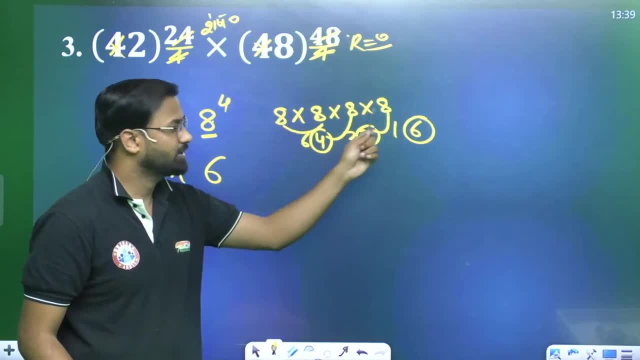 What did I say? I said that 8 has the power of 4,. I wrote 4 times 8, and 8 times 8 is 64,. I took 4, and 4 times 8 is 32,. I took 2,. 2 times 8 is 16, and took 6.. 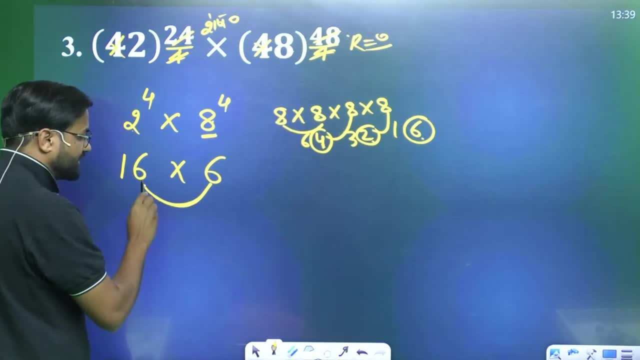 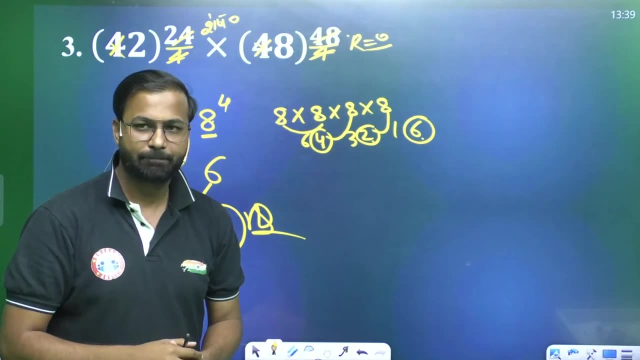 Let's move on to the last digit Now, distinguished 6, multiplied by 6,, 6 times 6, is 36, and 6 is your perfect answer. just sign it. we will get the answer right away. Got it Once again. tell me in the comments: did things come in, understands, or did you have a water glass kept on one side? 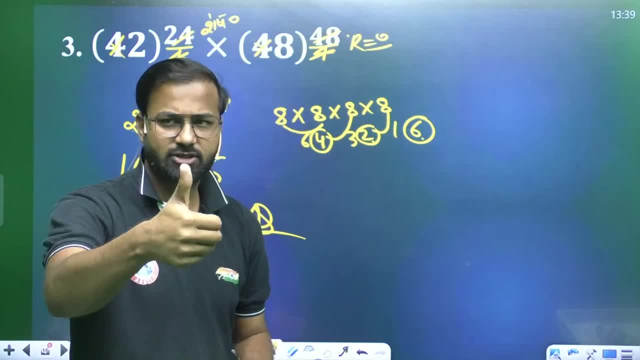 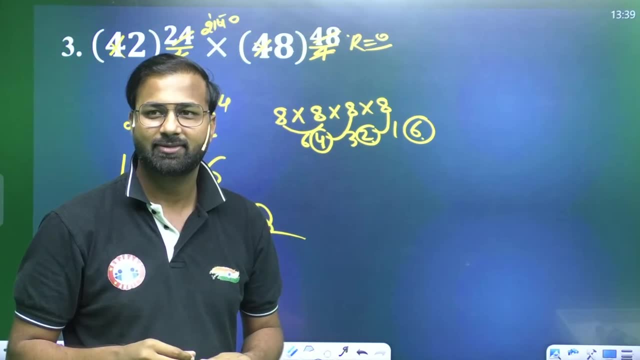 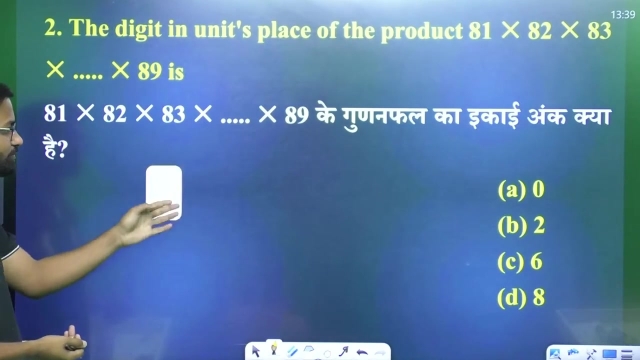 a glass of water. tell me what is happening. tell me quickly my shout, my hard work is going on. yes, very well, like this, lets move on. tell me the answer, tell me any answer, I will believe it. 81,, 82,, 83,, 89. 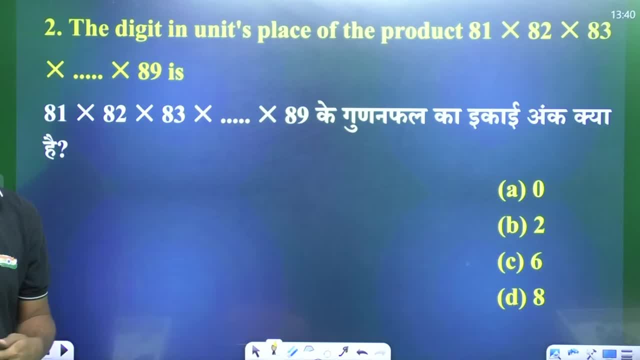 what will be the answer? tell me quickly What will be the answer to this question. 81,, 82,, 83, and so on, And things have gone up to 89.. Why are you guys so fast? How did you tell the answer to zero? 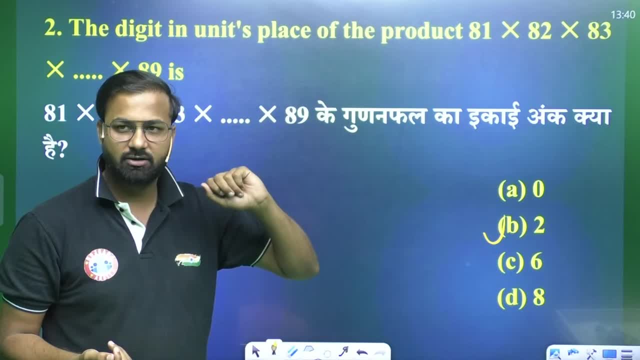 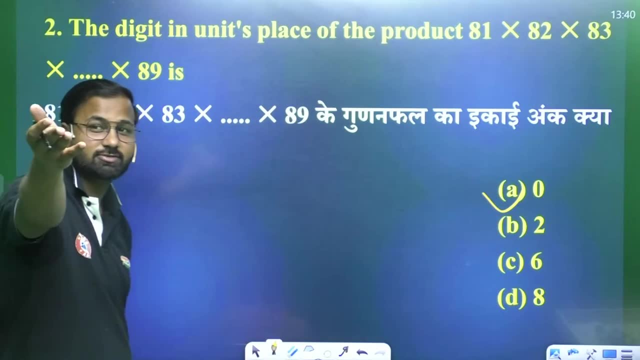 There will be two answers. What is the use of zero? Get me the answer to zero: Zero. people will run away like this: Zero answer is right. Don't run away. Have confidence in yourself If you go. 5,, 7,, 10,, 20,. 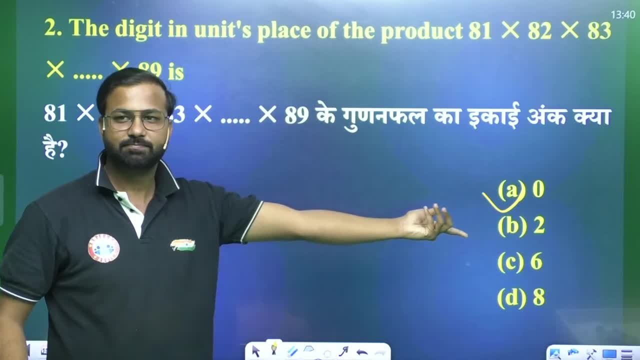 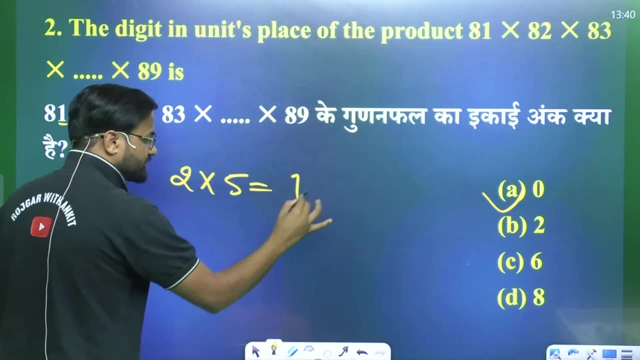 then even two answers will come. I have given two answers in a split second. Look here: you tell me Any number. if it is 2 times 5,, it becomes 10.. And it becomes 1 zero Wherever it is 2 times 5,. 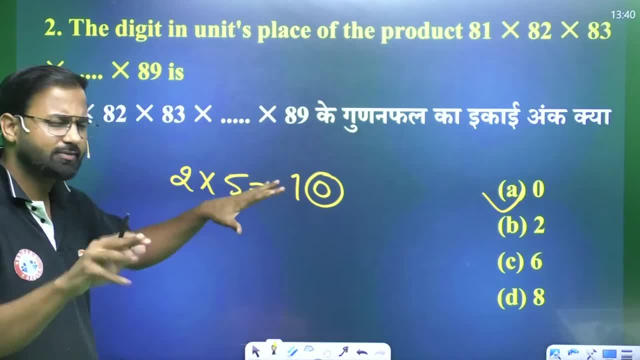 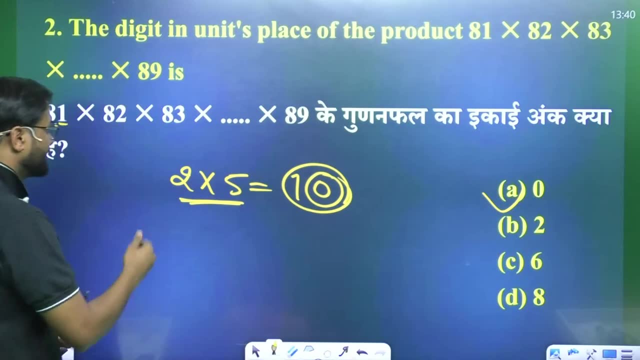 that number of zero. when we will read the number of zero, then we will read: But this is a basic concept: 2 times 5 is 10.. And you know 1 zero of 10 very well, Okay, So here you see. 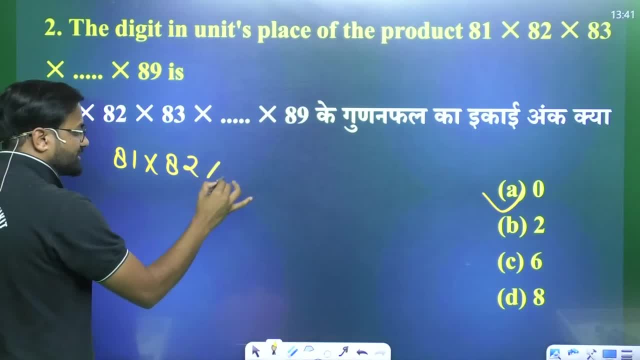 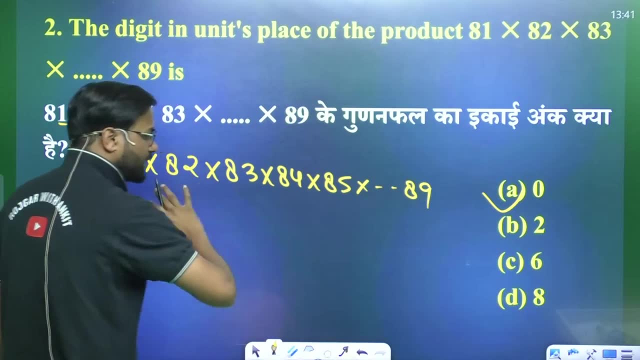 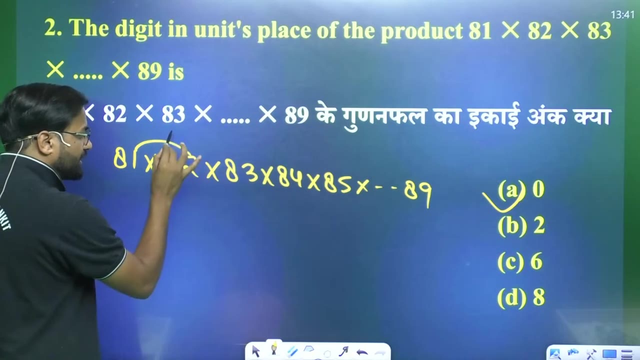 It is 81,, 82, and so on, 83,, 84,, 85. And so on until 89.. Now you don't have to find the unit digit even till the end. What you have to do is you will do this one times 2,. 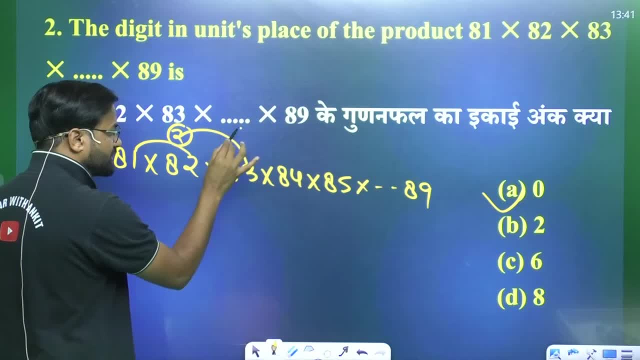 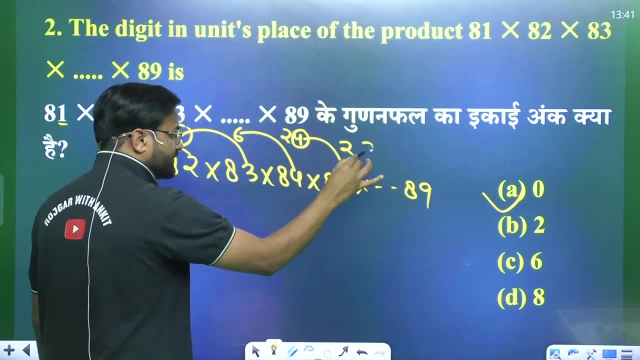 then 2 will come, 2 times 3 will come, Then 2 times 3 will come And 6 times 4 will come, Then 24 will come And 4 times 5 will come, Then 4 times 5 will come. 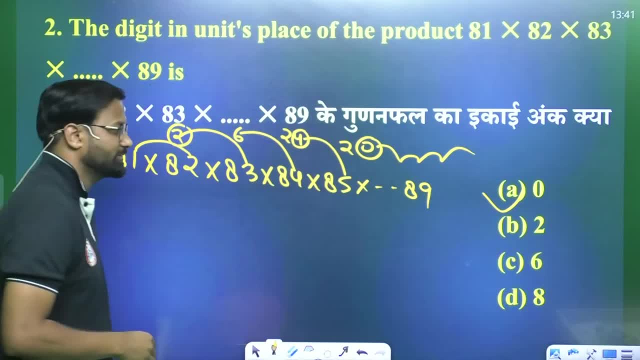 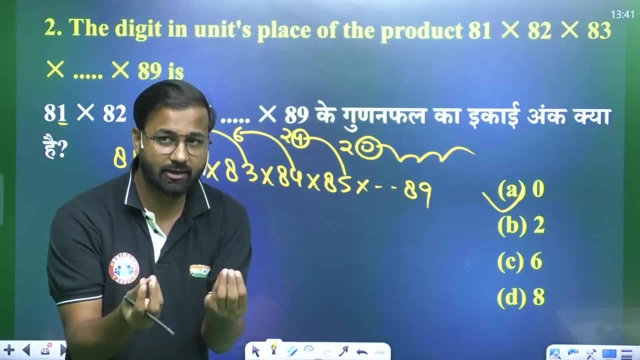 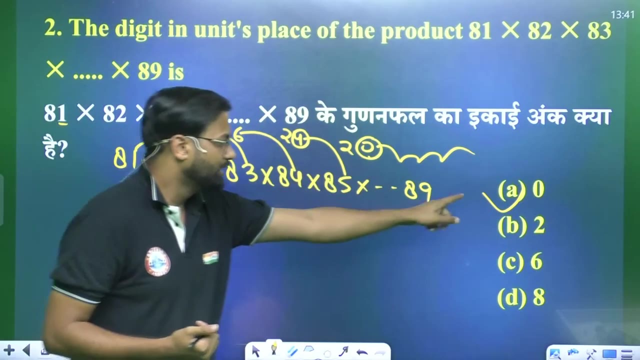 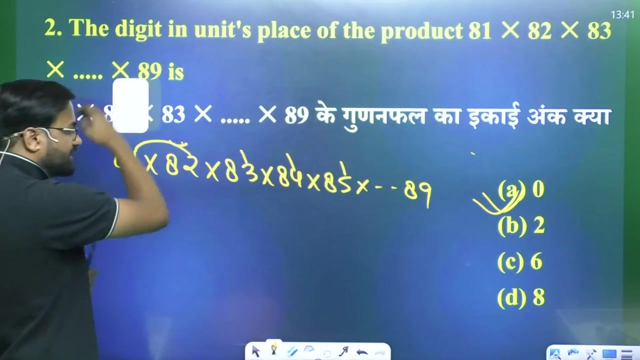 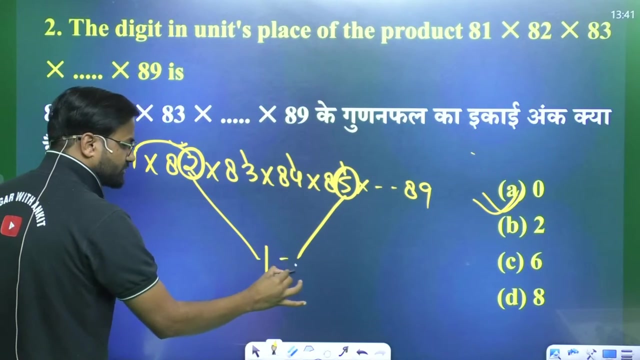 And then it will come zero, And then we will do the zero times in someone else. The second method is that you have seen that there are two units digits and one unit digit five. When these two units digits will be equal to each other, then we will create zero. we will 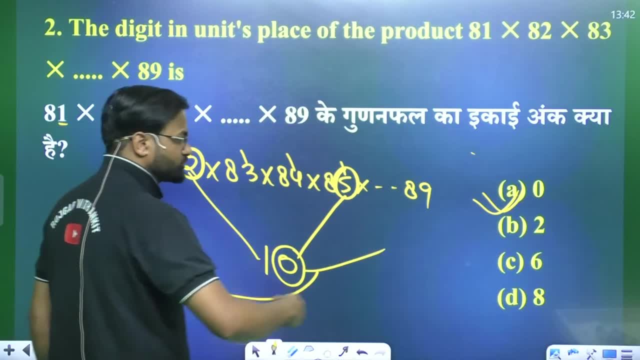 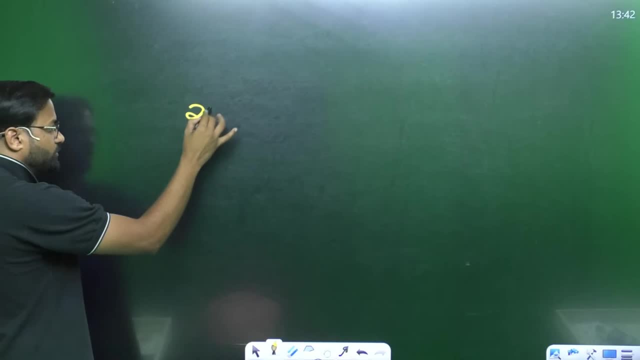 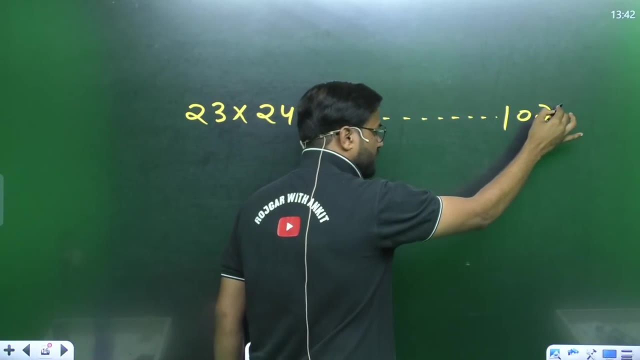 create zero, and then zero will be equal to anyone. smile, your answer has come. option number A. Option number A is absolutely correct. I will give you a question. I said 23 times, 24 times, 25 times and this number went like this till 1024 times. you will be scared to see this. 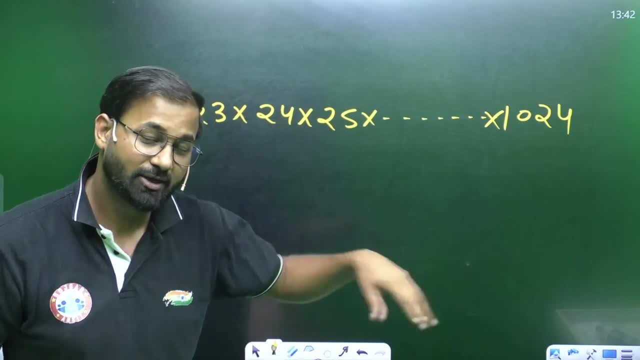 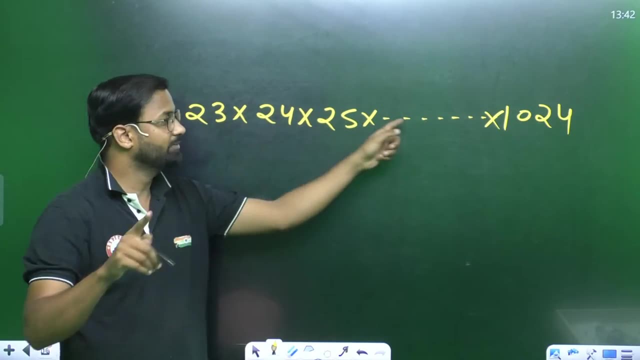 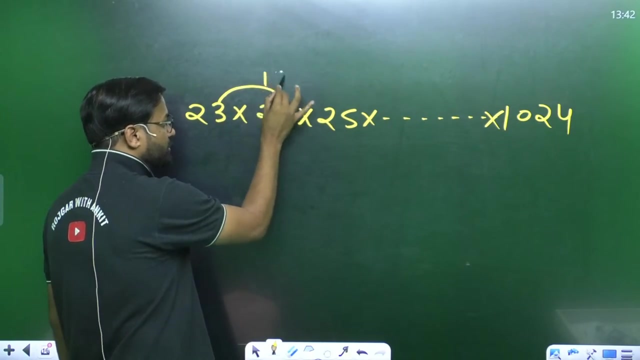 question For concept. If you are not scared, then why will you be scared? now, things have been set in your mind that wherever we got one zero unit digit and the number is in the number, then you have to smile a little and the answer will come. what will happen if you smile three, four, twelve? 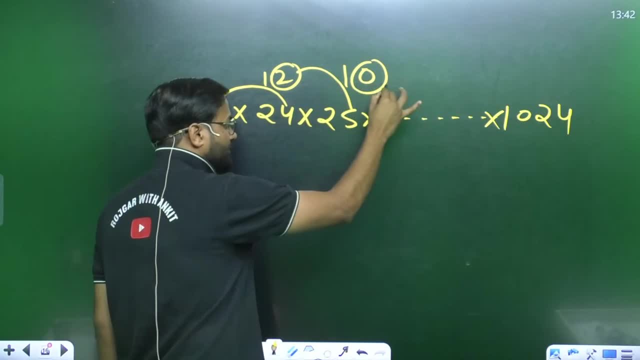 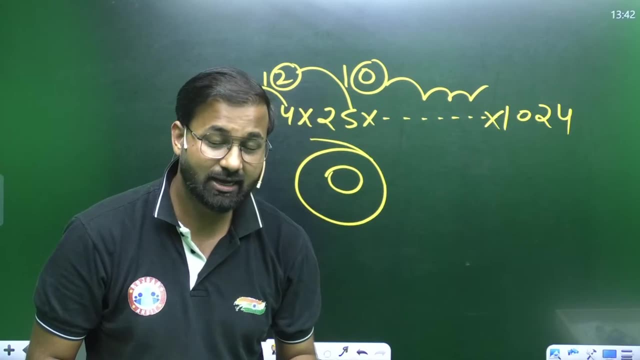 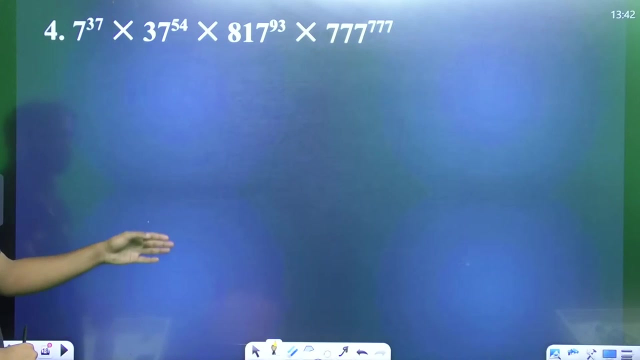 and then two came two times five will be ten and zero came, zero will be the number of any number in the world. your answer will be zero. your answer will be zero. then this concept is also clear. I will take you to some different type of question. tell me the answer of the question. 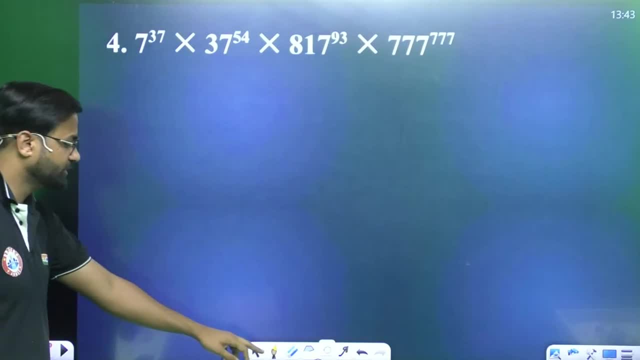 put your mind in it, practice, do anything. I don't know, but I want the answer from you. I want the answer from you people. what will happen? Brother? it is seven. I said 015,. if there is power, then whatever power the world has. 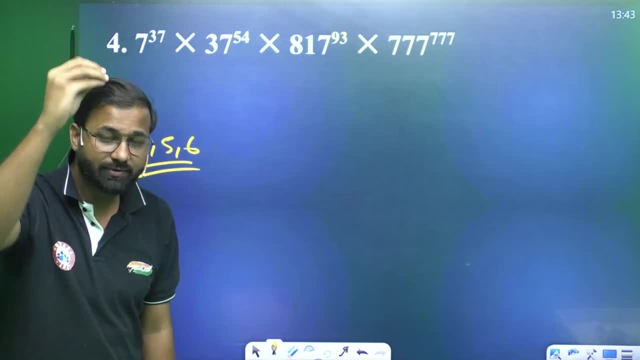 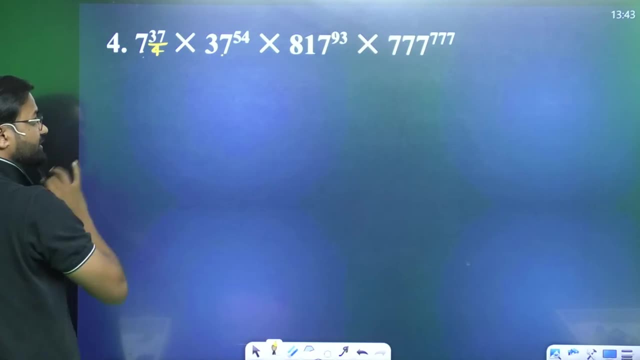 his friend. the unit digit has to be the same. the unit digit has to be the same we have. We have to see other than this. this is 7, 7, then divide the power of 7 by 4, how much is 4? name 36,, the final result is 1, then the power of 7 is 1.. 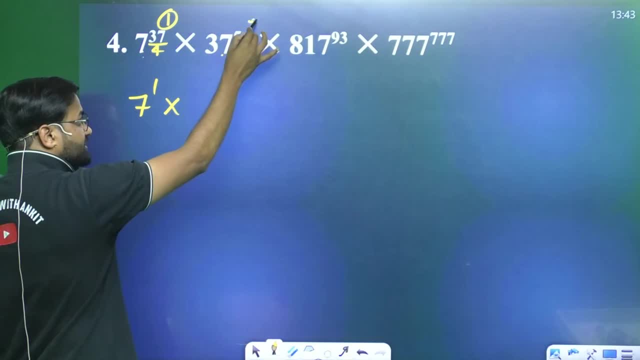 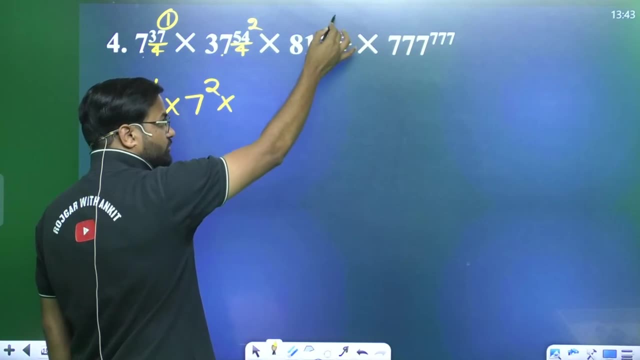 How much will this be? we will divide by 4, 13 square 52,. the final result is 2, the power of 7 is 2.. How much will this be? we will divide by 4, 13 square 92,, the final result is 1, the power of 7 is 1.. 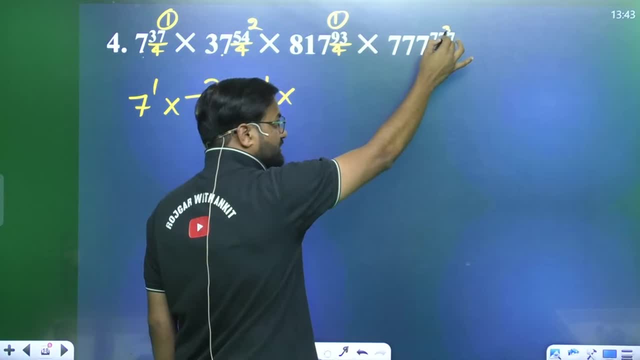 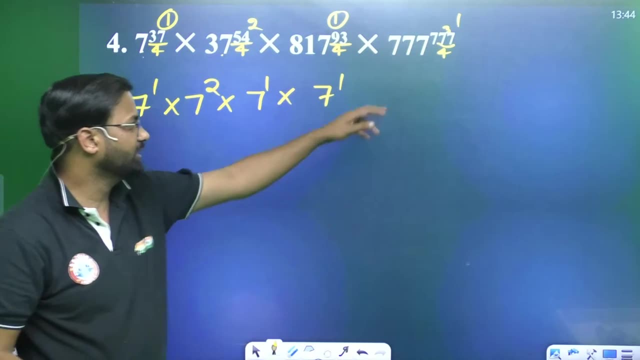 Here the last two digits mean 4 times 4, 3, 4. name: 36, 1,. the power of 7 is 1.. We have to write the final result remainder. we have to write the remainder. final result. the last two digits are 77,. 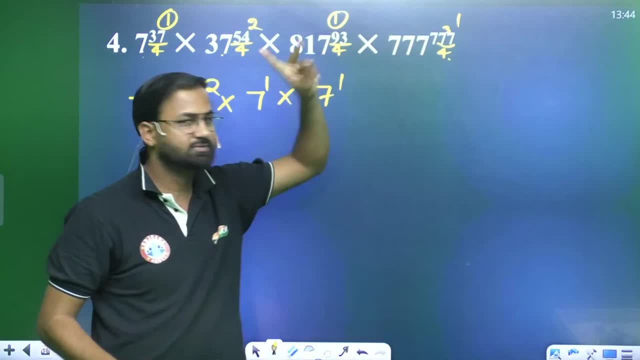 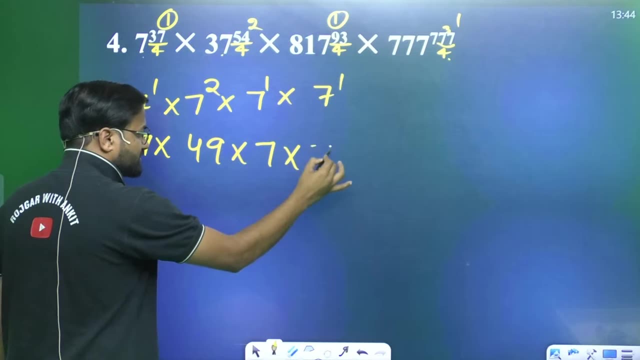 divide by 4, 4 times 4, 3, 4 name 36,. the final result is 1,. let's move ahead Now. what is 7 times 7, square 49, times 7, times 7.. 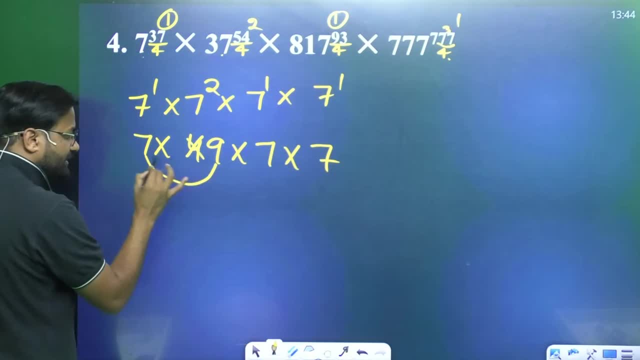 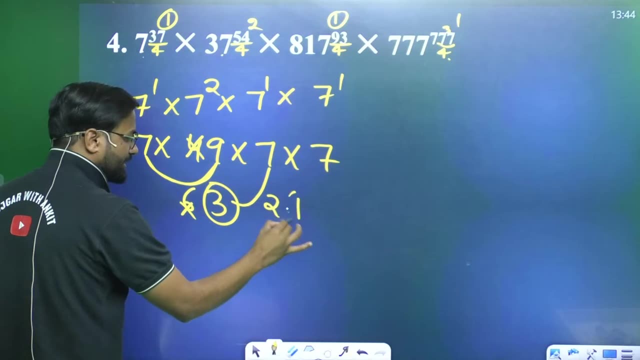 Now, last unit digit means this: 4 does not mean 7, name 63.. If you take 3, it does not mean 6,, 3 numbers 21,. if you take 1, it does not mean 2, and the 1 number 7,, and this will be your answer. 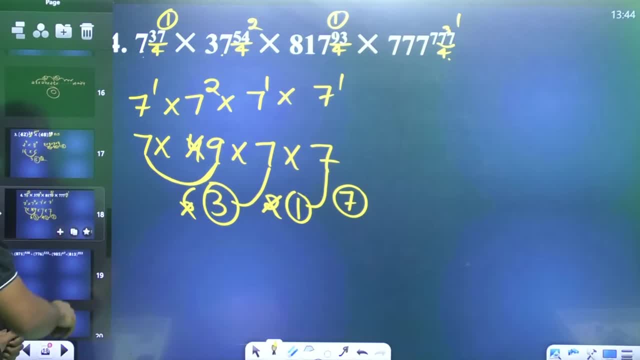 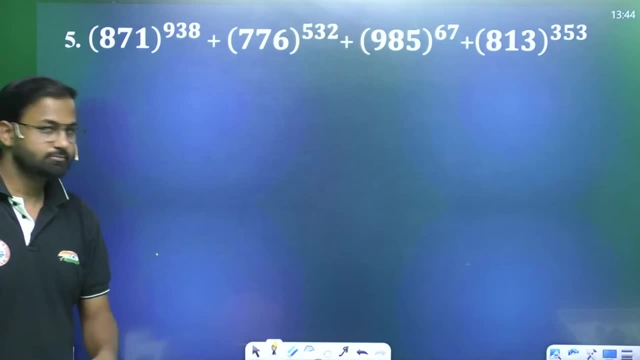 This 7 will be your answer. Dude, you have become very sharp in such questions. Do one more. tell me the answer. what will it be? What will be the answer to this question? tell me, Put your mind into it, what will happen. 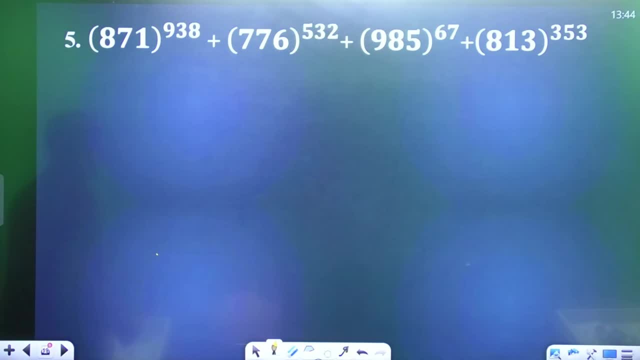 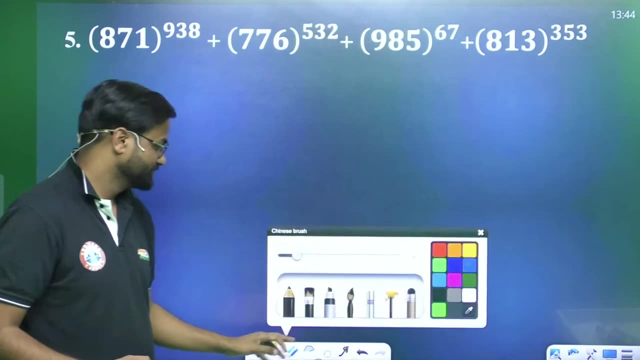 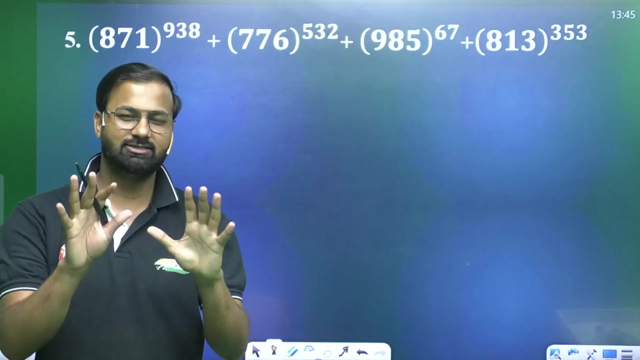 You are watching, Vinod, how sharp the children have become. Yes, Vinod, You are getting famous in the name of Vinod. then you are happy. Our country is a very different kind of country. People of our country know how to be happy. 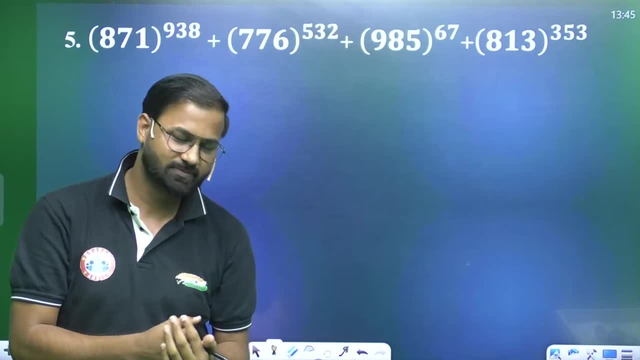 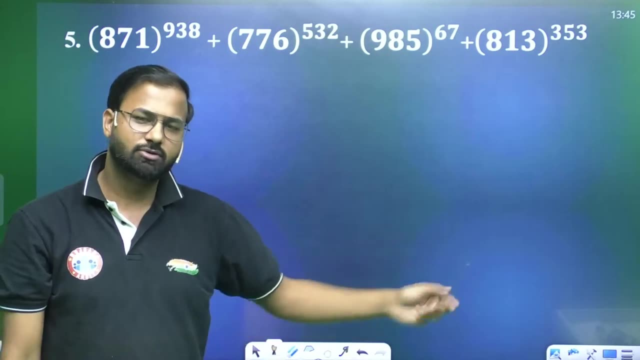 They find happiness in small things and this is the most speciality. Vinod- what is there? There is some dialogue. He is watching Vinod, Who says We have been saying since childhood: Look at Vinod, Look at mom. 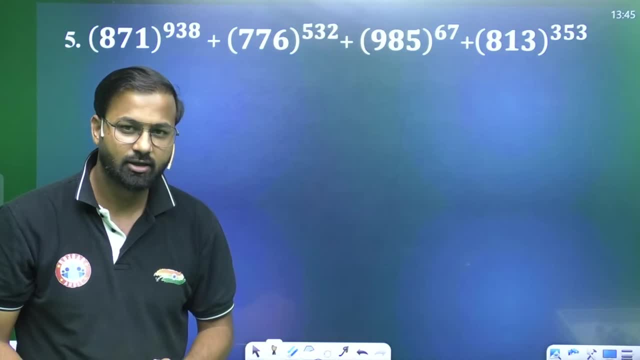 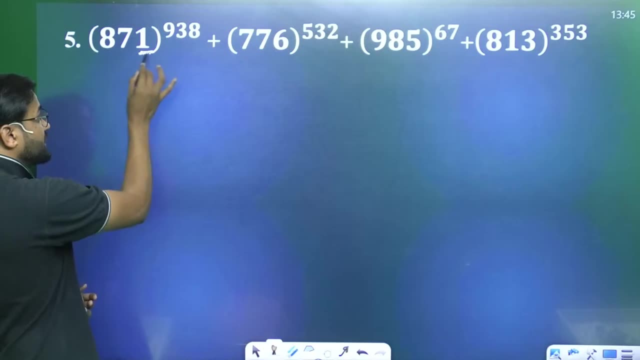 He is not giving me food, Brother. Look at papa. Look at papa. Brother is not giving food. Look at Vinod Brother has become famous. So this is my country. So here is one. One has the power of the world. 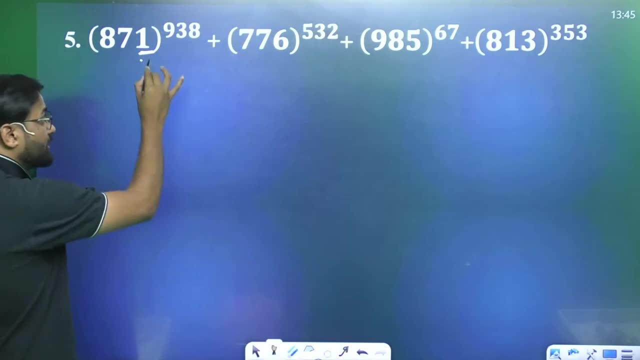 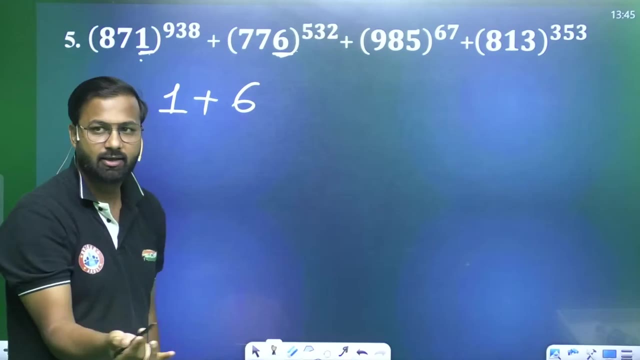 One has the power of the world. One has the power of the world. Unit is at one Plus sign in the middle: Six has the power of the world. Unit is at six. We don't have to see, We don't have to divide from four. 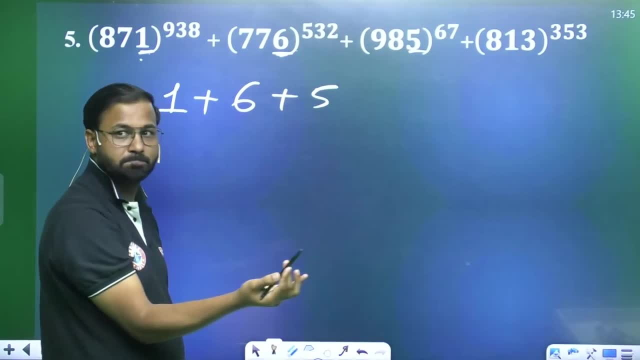 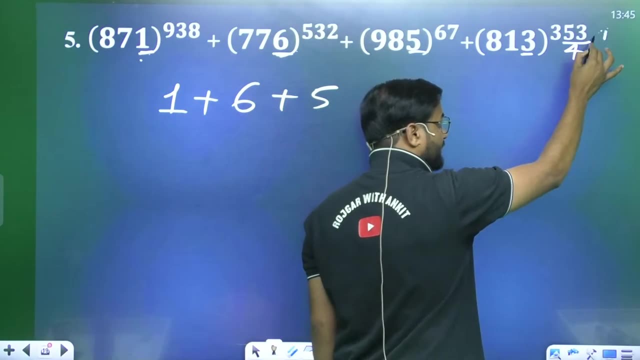 Five has the power of the world Unit is at five. Wow. But in the case of three? What to do in the case of three? Divide the last two digits by four, Thirteen, Four, Fifteen, Come Successful one. 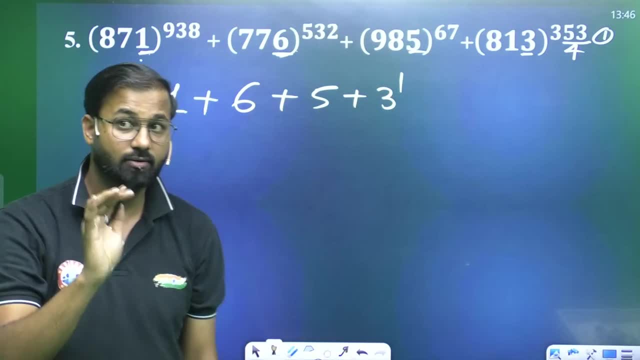 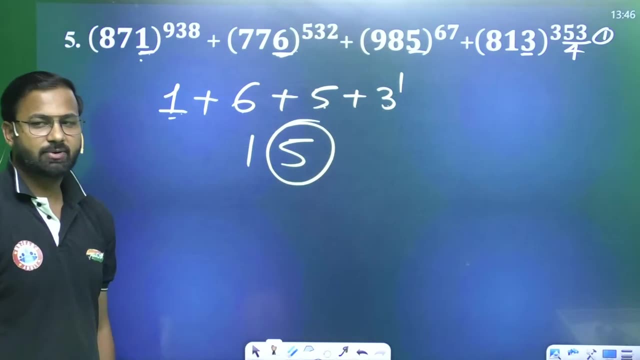 We have to put the power of three here. Wow, Wow, Wow. What will do here? Join all here: Six and one, Seven, five, Twelve and three, Fifteen. Unit digit is five. Your answer is absolutely correct. 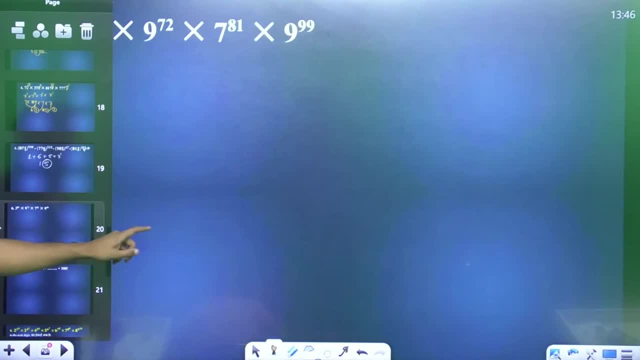 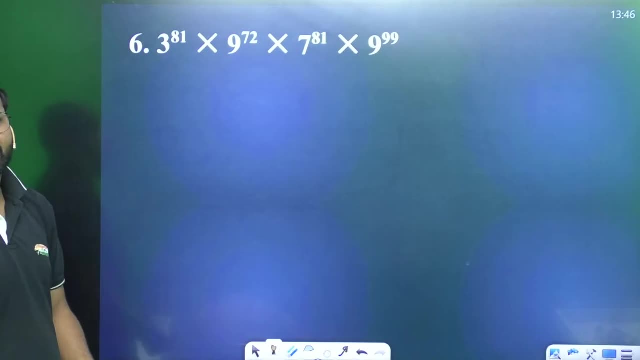 You keep doing big questions in such small ways. Okay, Do this question quickly. Quickly, I will find the answer to this question. If you want the answer to this question, what will you do in this question? Will you quickly tell everyone that 3 has power 81,, 9 has power 72,, 7 has power 81, and 9 has power 99?? 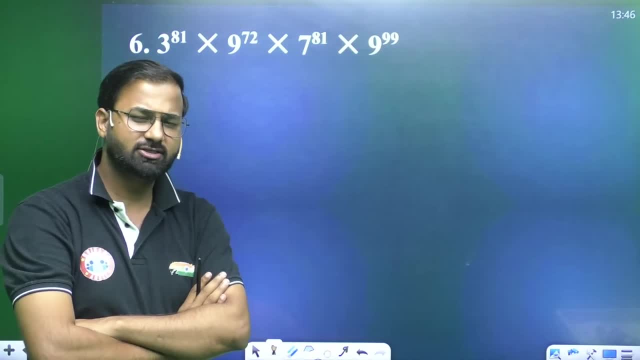 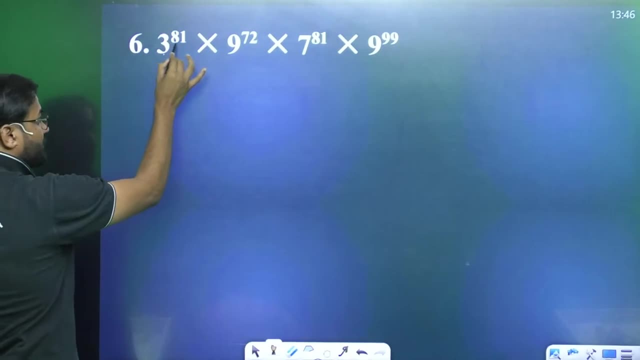 Tell me quickly Now. you will think that I have been shouting for an hour and still you are not getting the answer. So here you have power 81 of 3, divide by 4.. Power of 3 is 1.. We will divide 72 by 4.. 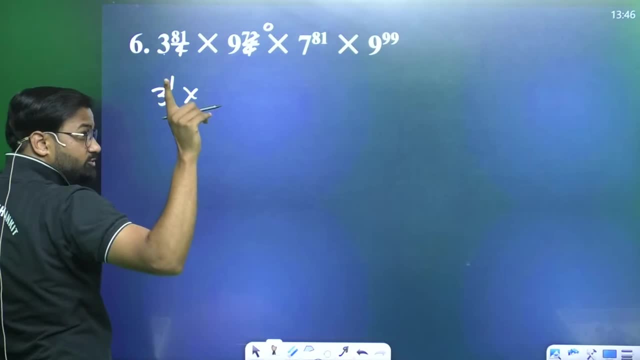 18 square is 72.. The final result is 0.. And where the final result is 0,, the power is 4.. Here we will divide 82 by 4.. 20 square is 80.. Final result is 1.. 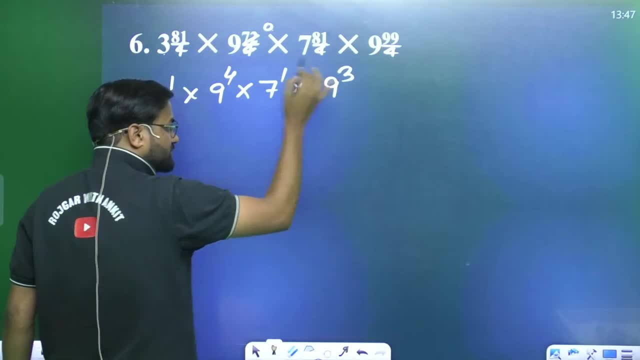 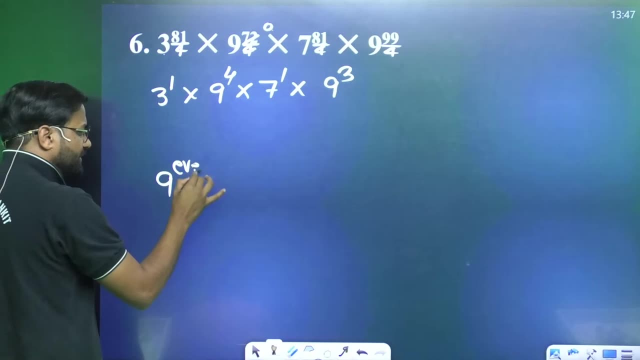 We will divide by 4.. 24 square is 96.. Final result is 3.. Now you see, Let me tell you a concept of 9.. Power of 9 is 1.. If the power of 9 is even, that is, if there is a sum number, then its unit digit is 1.. 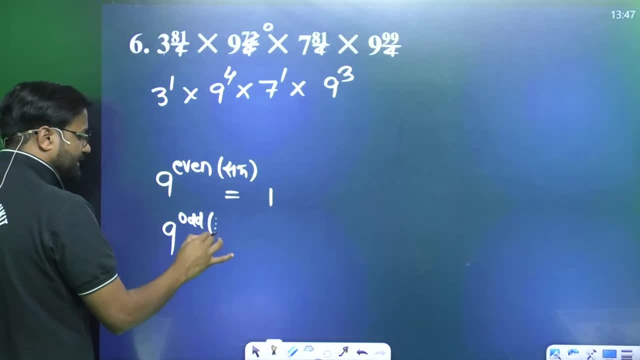 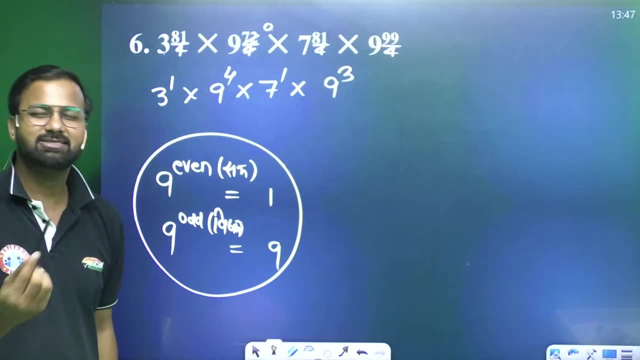 And if the power of 9 is an odd number, that is, if there is a divisible number, then its unit digit is 9.. In the case of 9, you can also remember it directly. If you do not remember even and odd, then consider the power of 9 as 2.. 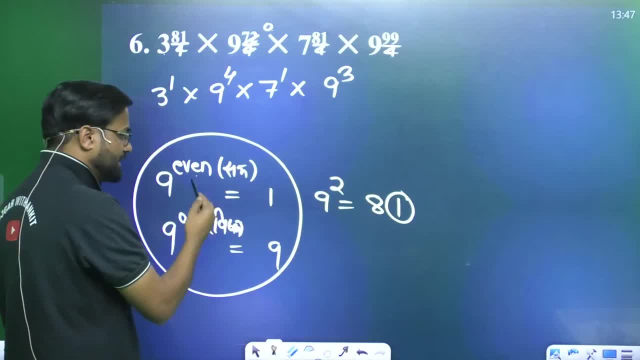 I remembered it the same way when I studied in the beginning. I did not study E1P1 earlier. I considered it as 2 numbers. The unit digit will always be 1.. Power of 9 is odd. Power of 9 is an odd number. 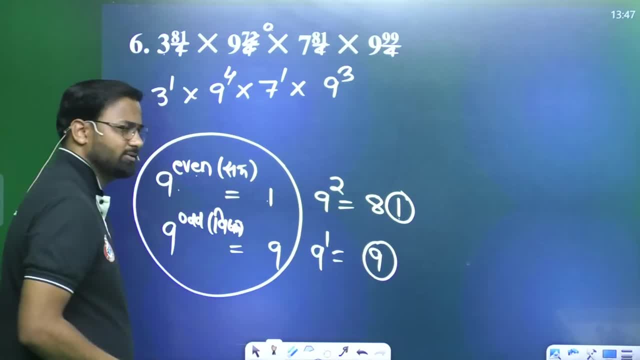 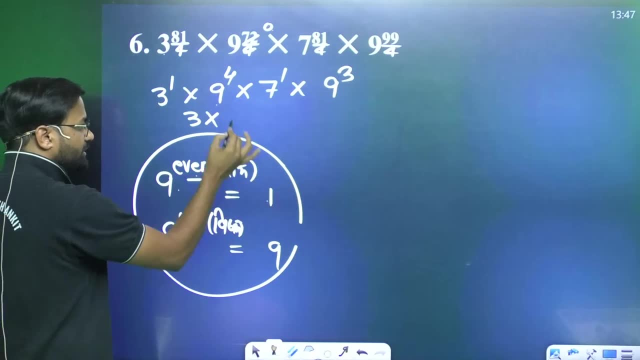 The smallest, power of 9 is only 1.. 9 will only be added. remember it as well. So here you saw that power of 9 is 4 and is an even number. so the unit digit will be 1.. The power of 9 is an divisible number. there is an odd number, 3.. 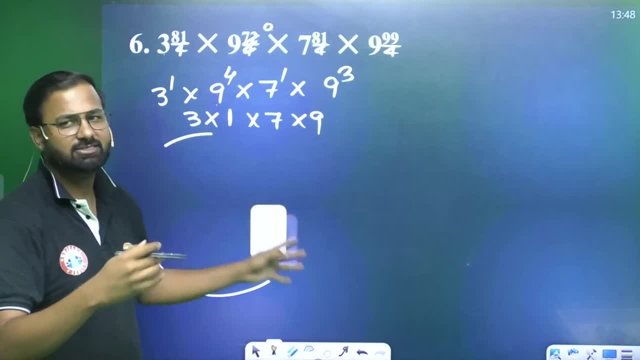 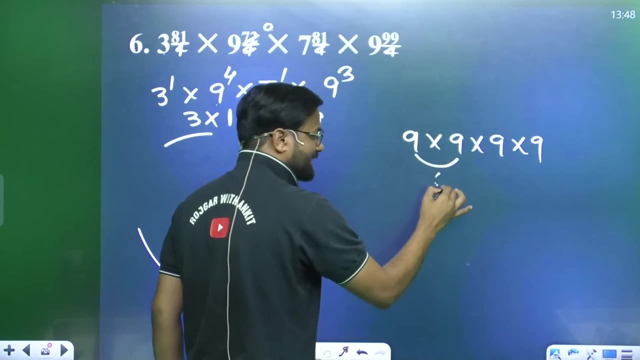 The unit digit will be 9.. You do not want to do this anyway. The power of 9 is 4.. Divide 9 by 4 times 4 times What was 9?? Take 1,. 1 is 9 and 9 is 81,. unit digit is 1.. 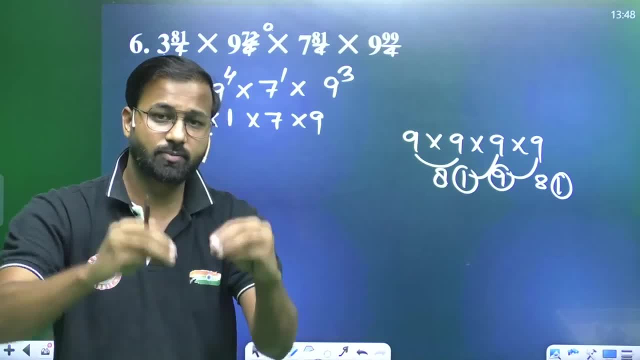 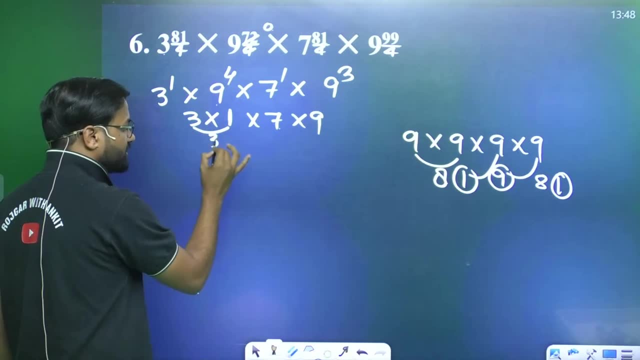 I have given you all the ways. even if you don't know the formula, you will get the answer. So here the answer will be 3x3, 3x7 is 21,. 3x3, 3x7 is 21,, 21 is 1 and 1 is 9.. 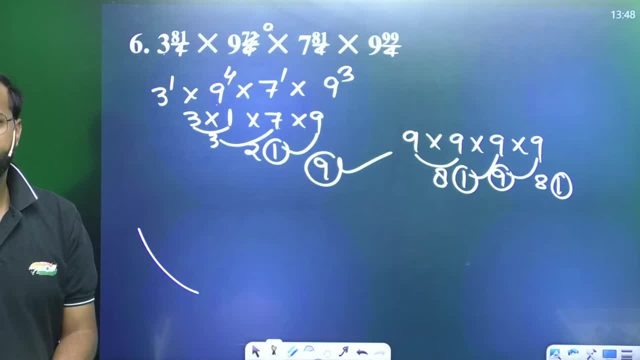 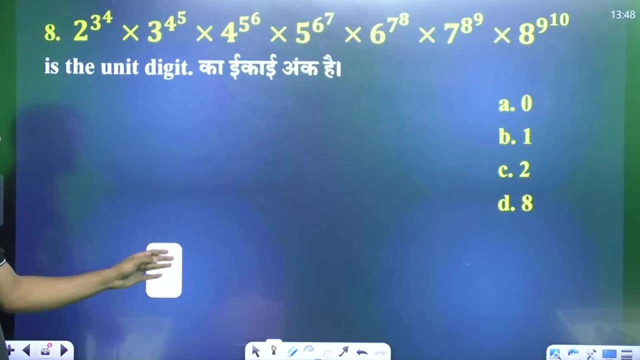 The answer is 9,, which is the correct answer. Okay, I have given you all the ways. Now let's move on to this question, Sir, what kind of question is this? You gave the power of power as well. What kind of question is this, sir? 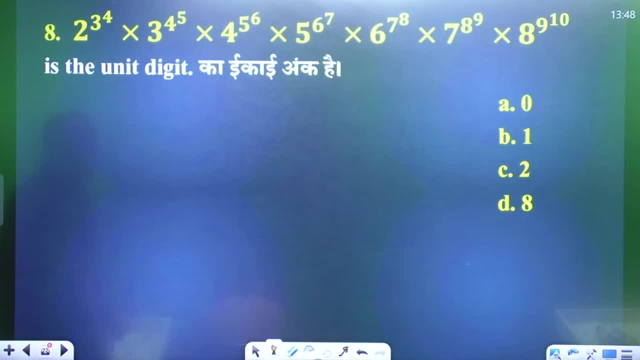 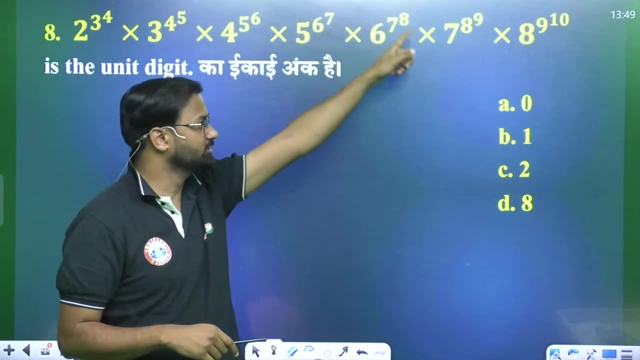 Power of power as well: Power of 2,, power of 3,, power of 4,, power of 3,, power of 4,, power of 5,, power of 5,, power of 6,, power of 5,, power of 6,, power of 7,, power of 8, power of 7,, power of 8,, power of 9,, power of 9,, power of 10.. 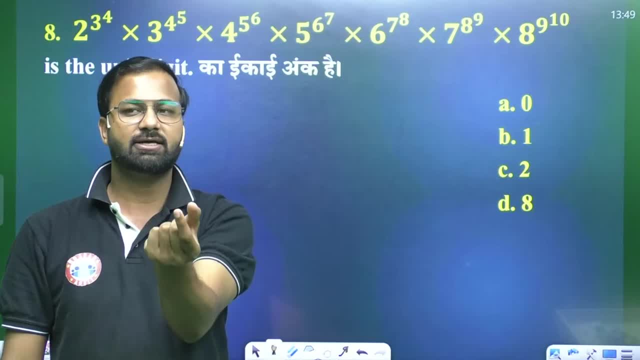 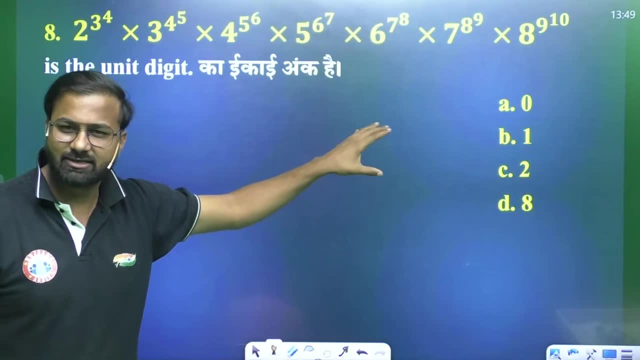 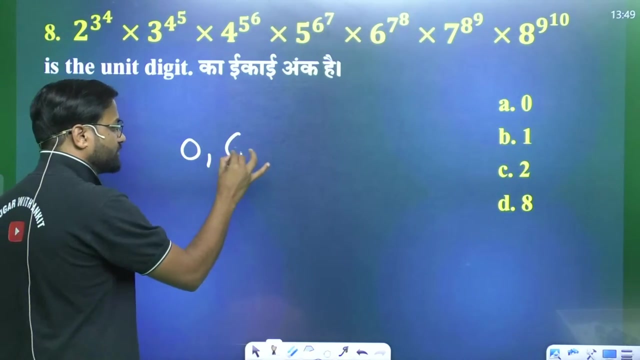 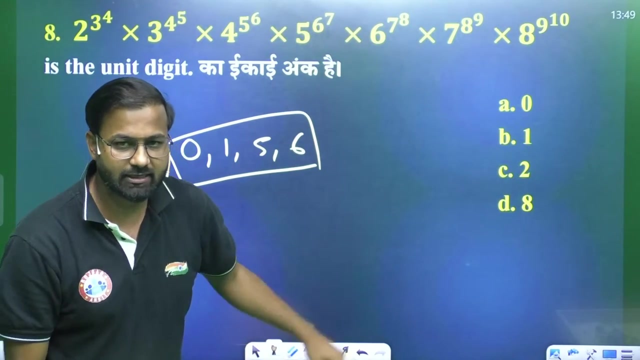 How did I start? I started with a small number, unit digit. And where? What did you think about this? This is the easiest question of the day. I told you that if the unit digit of any number is 0,, 1,, 5,, 6,, then any number of the world will be 0,, 1,, 5,, 6.. 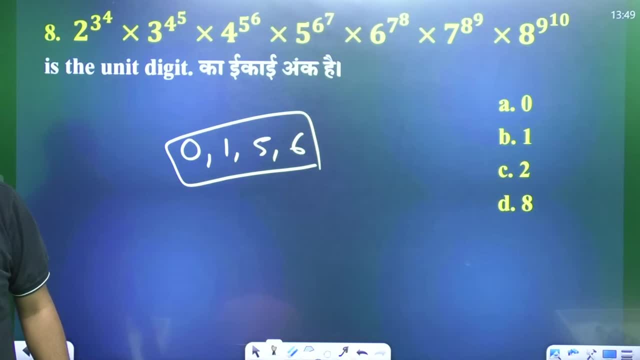 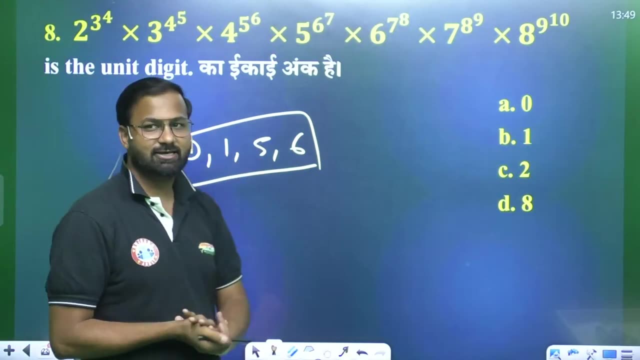 Tell me what will happen, Rajneesh, show me that M-table. So if 0,, 1,, 5, 6 are present, then any number of the world will be 0,, 1,, 5, 6.. 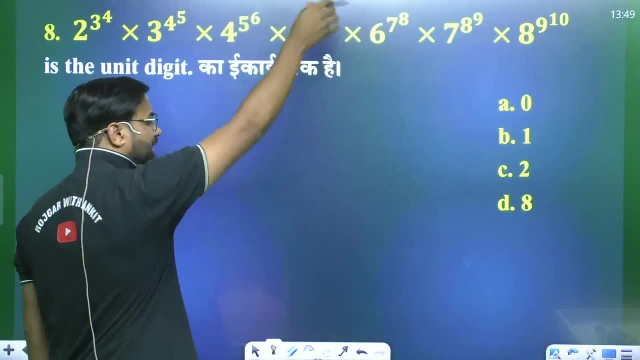 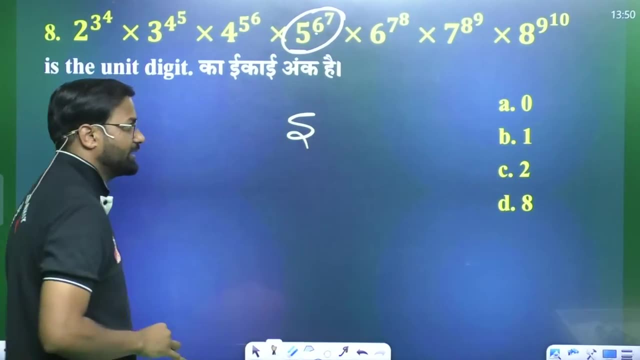 So you saw that this is 5, but the power of 5 is 7 and the power of 6 is 7.. So even if the number of the world is 0,, 1,, 5,, 6,, then any number of the world will be 5.. 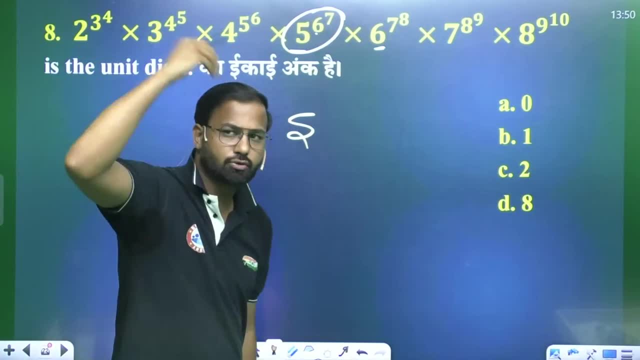 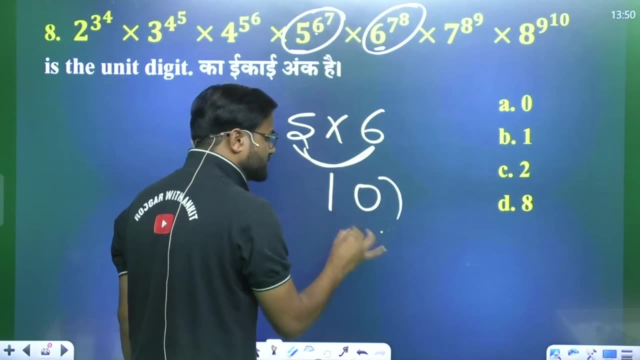 And then you saw that it is 6.. No matter what the power is, ie 6 is going to remain as i Yes, And when these two will be equal to each other, then we will create a zero. And if we make the zero equal to anyone, then what will be the answer? 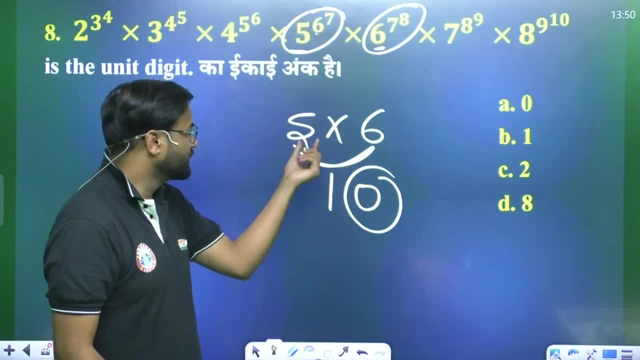 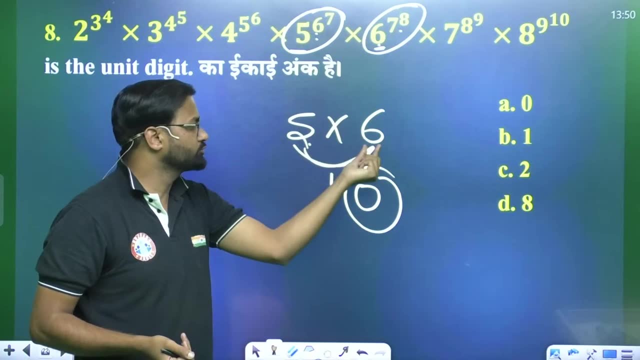 Zero will come. No, show me like this. Show me Okay. So what will be the answer? Your zero is going to come, Because I saw that the power of 5 is some 5,, the power of 6 is some 6, and when they are. 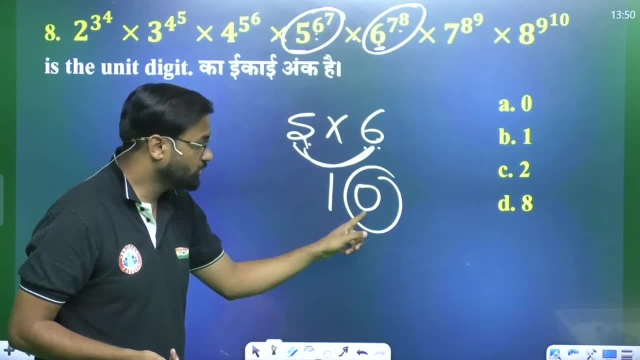 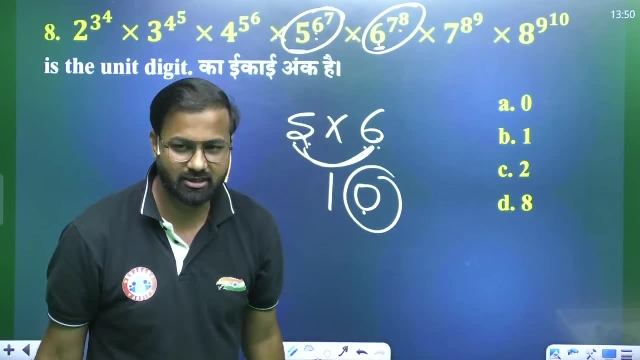 equal to each other, because there is a sign of equal in the middle. then the zero came. And when zero will be equal here as well as here, everything will be balanced. What will make everything balanced? The answer will be zero, Absolutely correct. 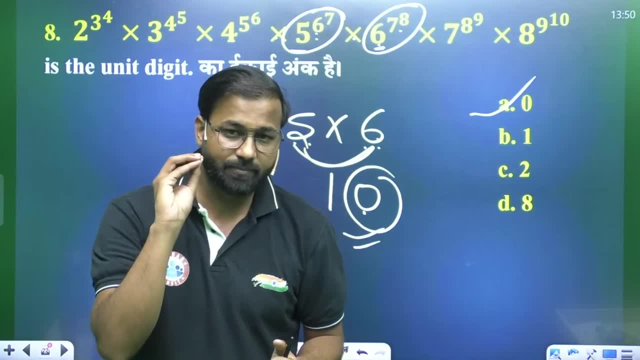 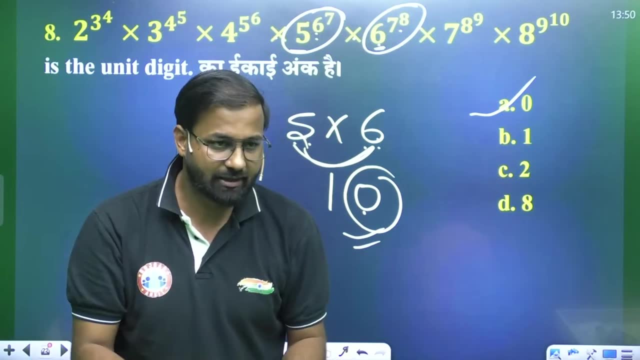 You have the answer. Let me tell you the timetable. Classes have been held since today. Reasoning has been done at 12 o'clock. A very exciting session has taken place. My class is going on at 1 o'clock. Math will go on regularly. 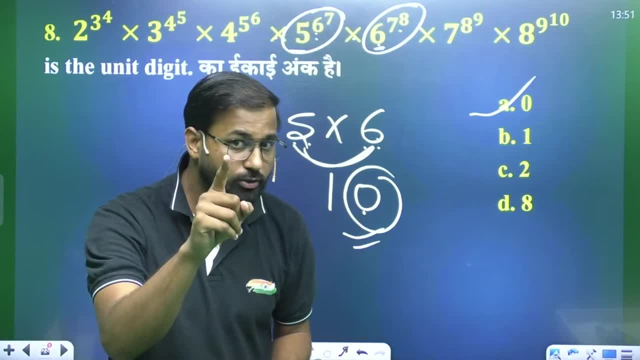 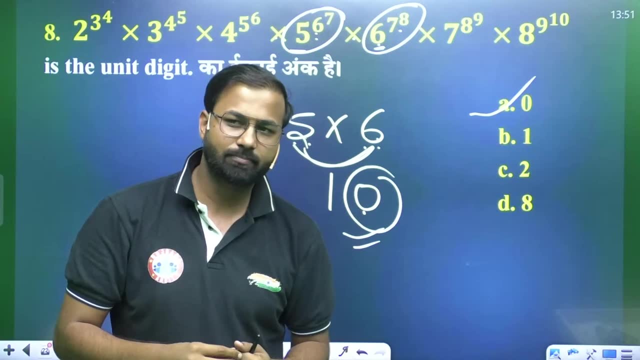 And after that Neeraj sir is coming in Hindi from 2 o'clock, So do not forget to join. Hindi is a very interesting topic And the energy of Neeraj sir, I bet, if you miss in any class and then at 5 o'clock, Ajit. 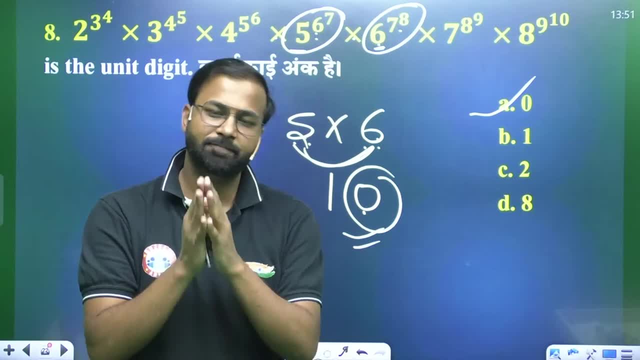 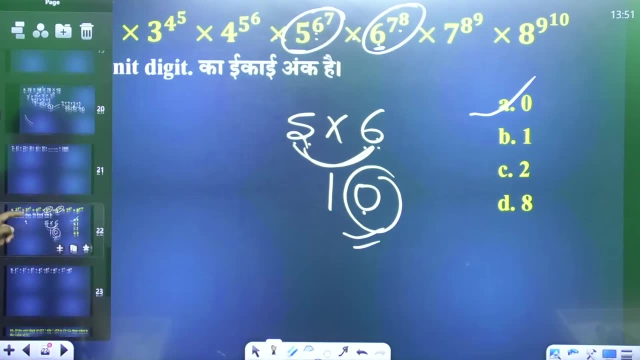 sir will start GS and at 6 o'clock Vipin sir will start English. So do not forget to join everyone today. So you have done this question. Come on now. I will tell you a little bit of the concept of factorial. 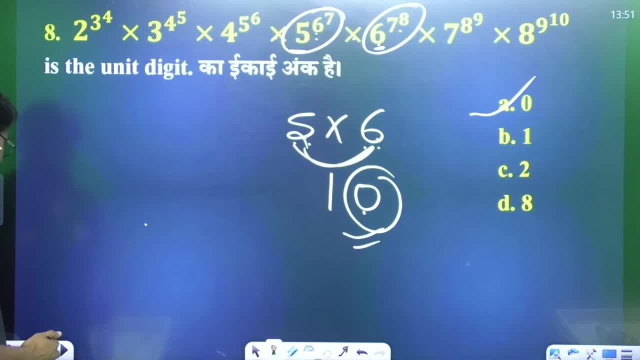 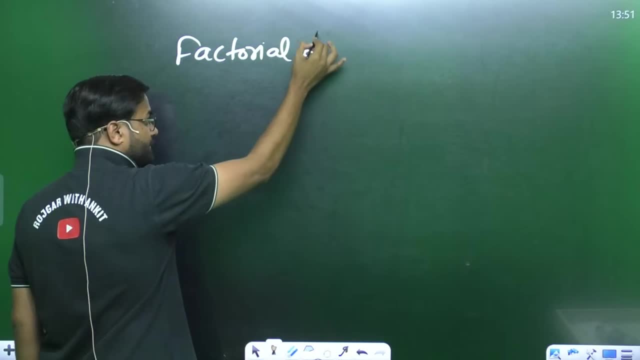 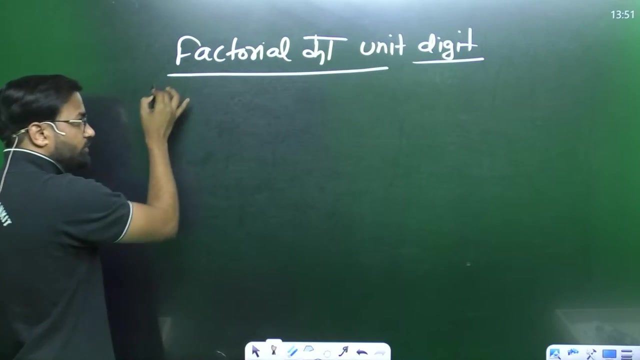 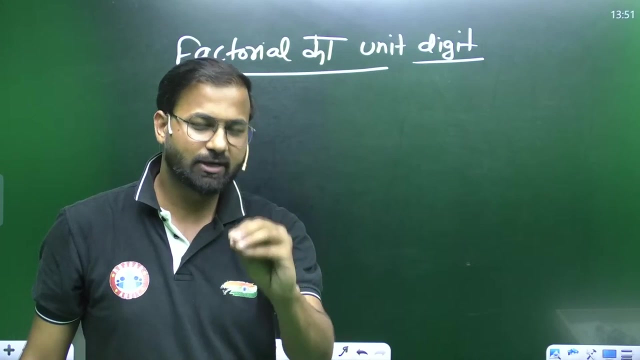 Let me tell you a little bit of the concept of factorial. This is what is left: Factorial, Factorial, The unit digit of factorial. Sir, how come factorial is now? How come factorial is now? That's the easiest topic, the one you have already studied. 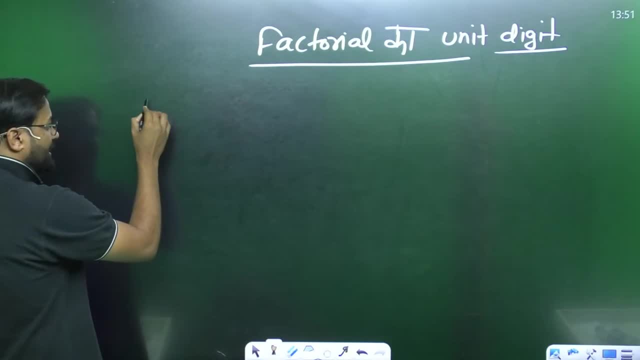 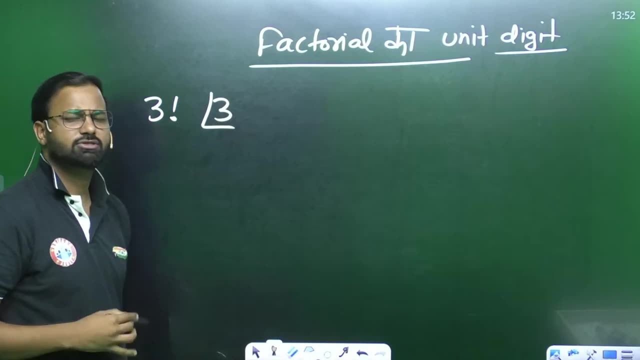 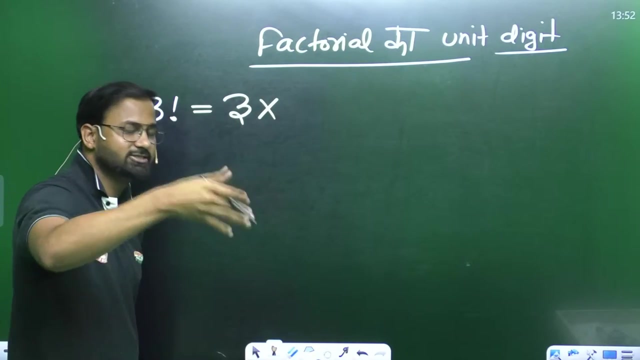 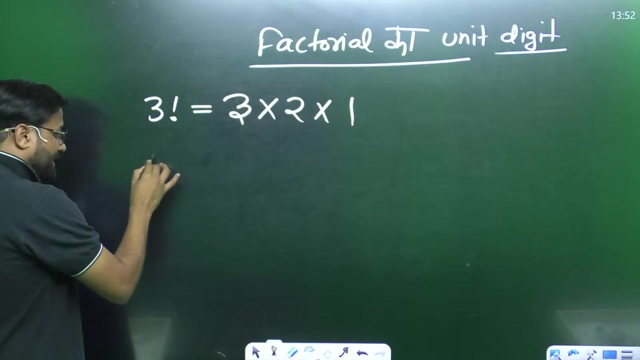 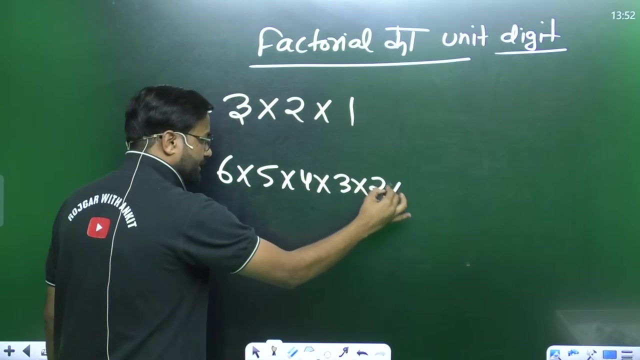 That's too easy. Factorial and factorial unit digits. All right, n factorial, 3 factorial is a sign of factorial in this way. you must have seen it written like this: 3 factorial in this way. so 3 factorial, just smaller than 3, natural number 2 and smaller than that natural number 1, let's multiply the number up to 1, I said 6 factorial, so 6 times 5 times 4 times, 3 times, 2 times 1,. 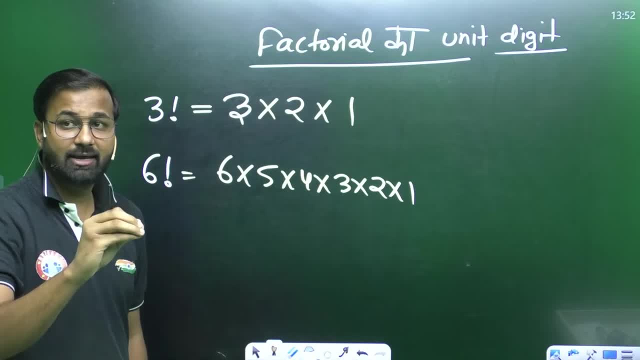 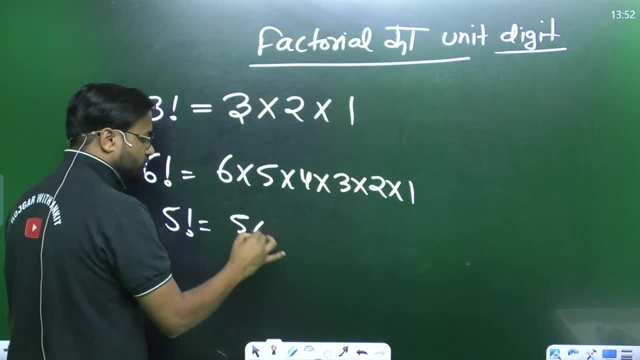 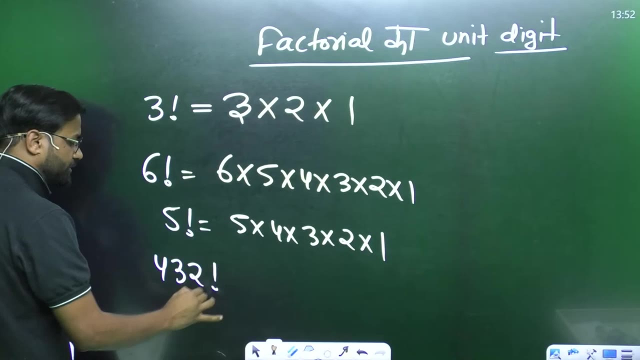 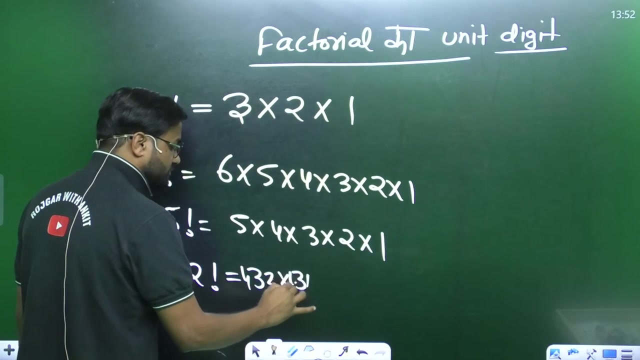 let's multiply the number up to 1, and I said 5 factorial, so you will say 5 times 4 times 3 times 2 times 1,. let's stop at 1,. I said 432 factorial, so what will you call 432 factorial, 432, 431, and this multiplied by 3, 2 and 1,. 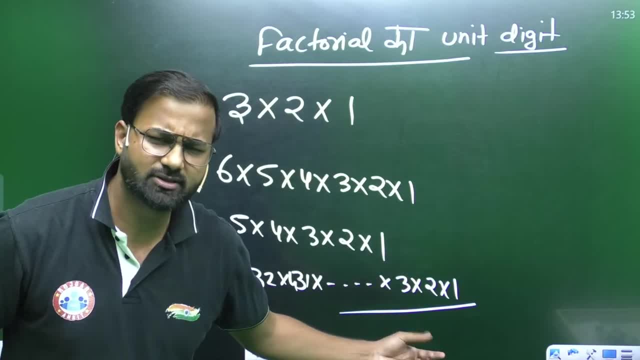 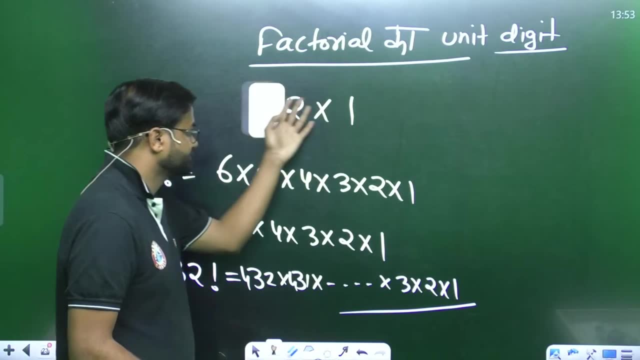 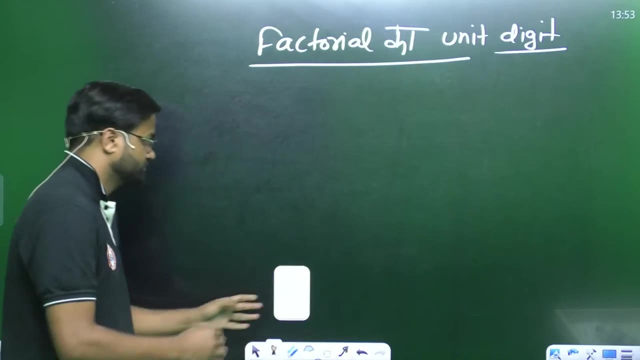 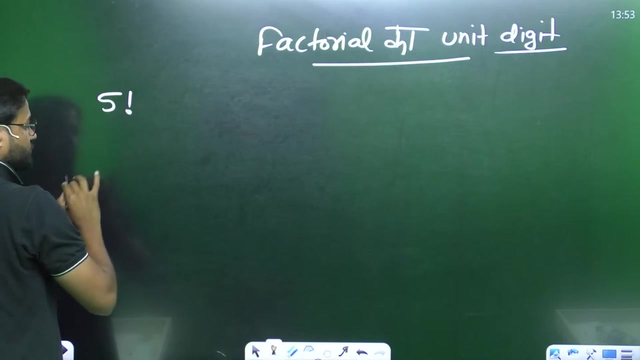 it will end at 3,, 2 and 1, factorial means it is clear. you understood now. you understood now as I now ask you a question. I ask you a question, I asked a question. 5, factorial. 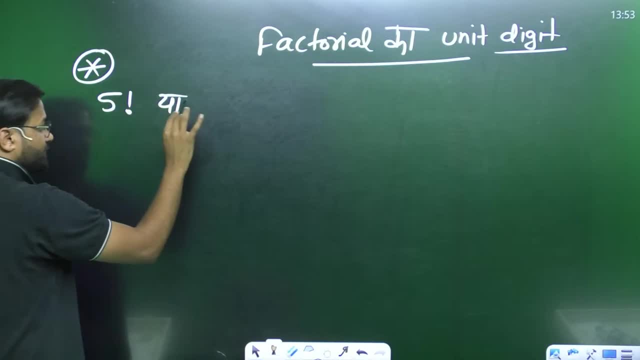 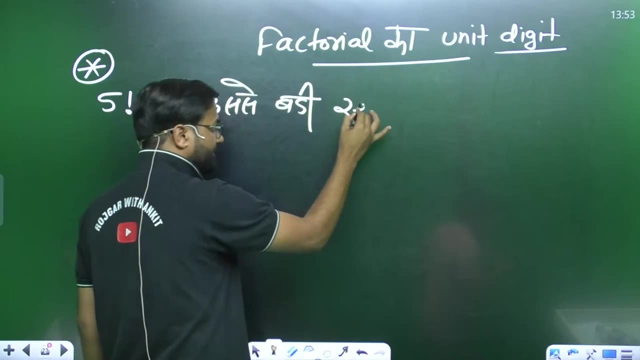 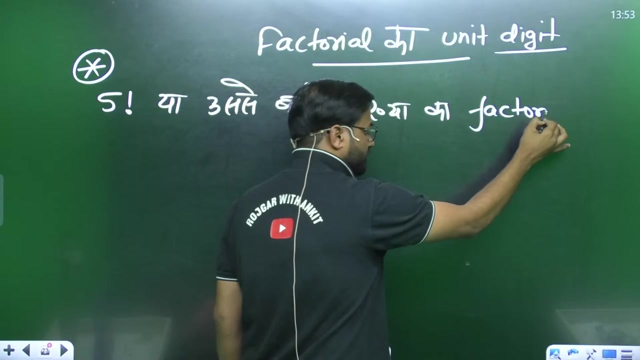 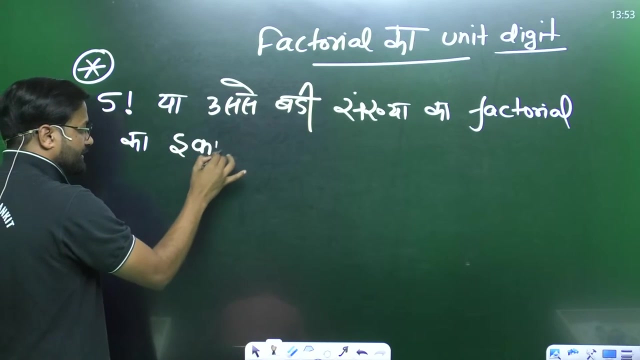 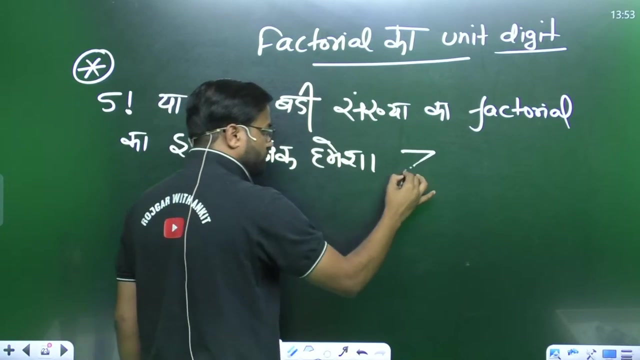 yeah, not a question. write it as a star: 5 factorial. 5- factorial or bigger than that factorial. 5- factorial or bigger than that factorial. 1 number: 1 number will always be 0, write it as big, it will be 0,. 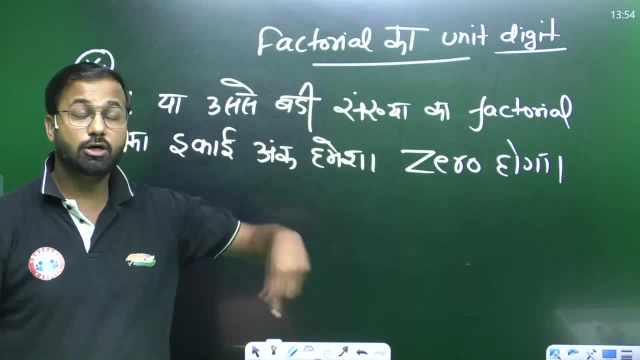 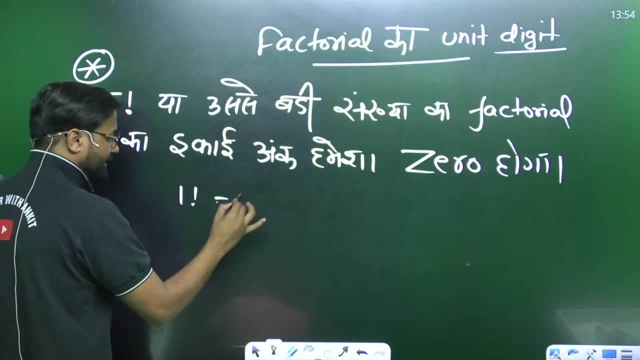 5. factorial starts with any number or greater than that factorial: See 5. factorial means: see 1. factorial means 1, 2. factorial means 2 times 1, ie 2,. 3. factorial means 3 times 2 times 1, ie 6,. 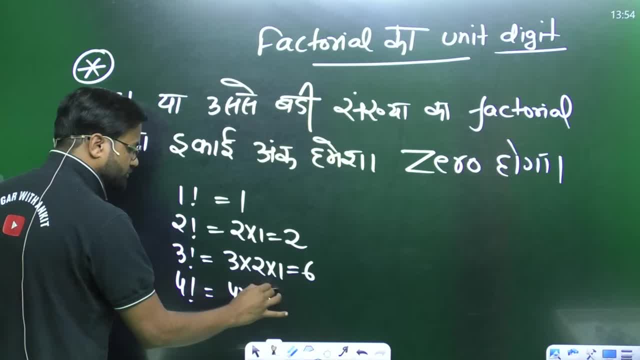 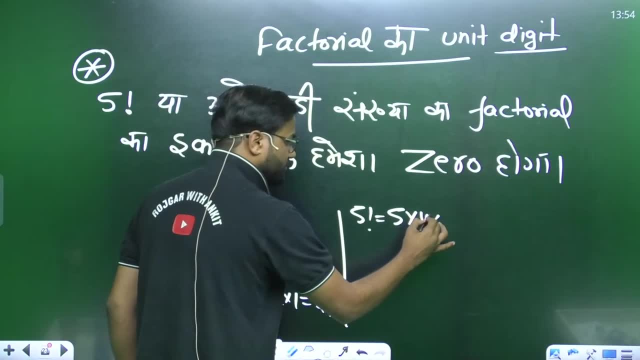 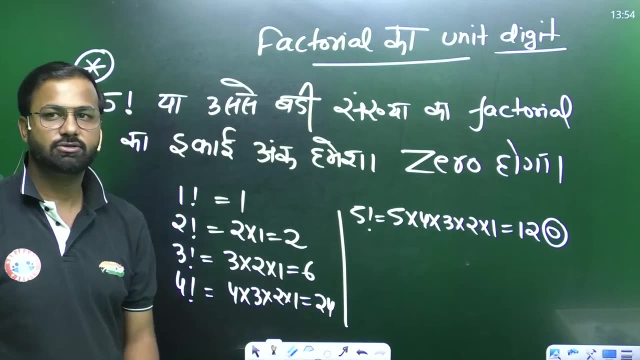 4 factorial means 4 times 3 times 2 times 1,, ie 24, and whenever 5 factorial mandated. 5 factorial means 5 factorial, x, 4 x, 3 x, 2 x 1 means 120 and the unit number of 120 is 0. and from here and from here, 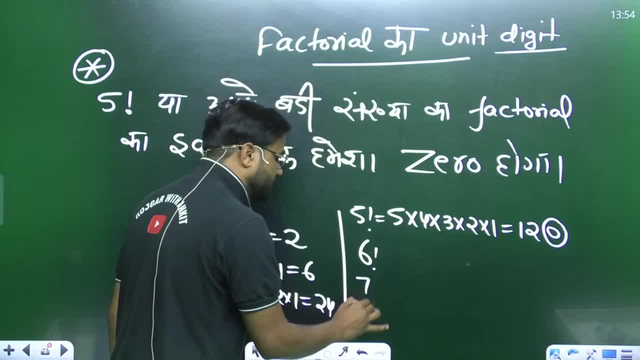 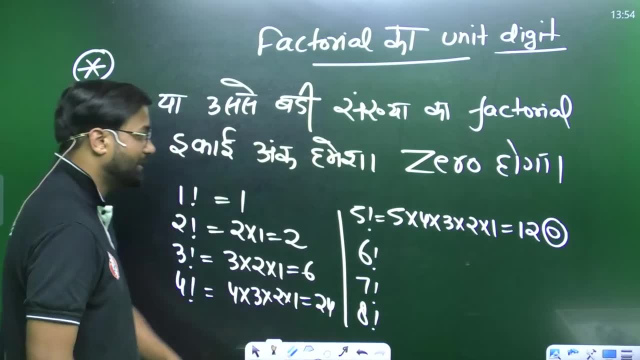 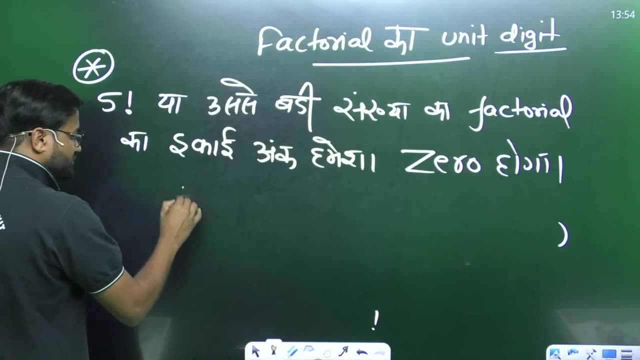 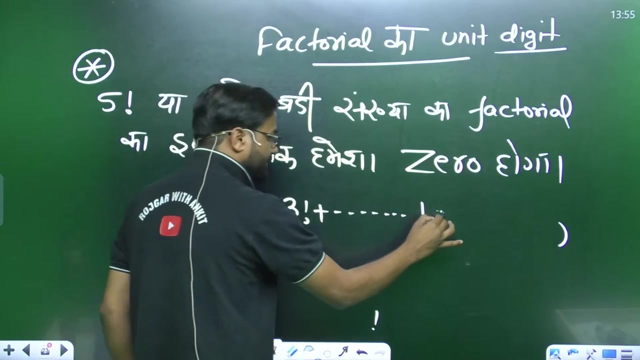 any factorial you take, 7, 8, any factorial you take, its unit number has to be 0, its unit number has to be 0, always ok. so now, as I gave you a question here, I gave you: tell me 1 factorial plus, 2 factorial plus, three factorial plus, and then go by 10 factorial. tell me. 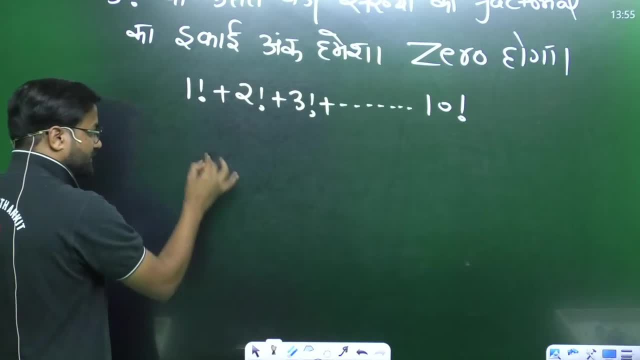 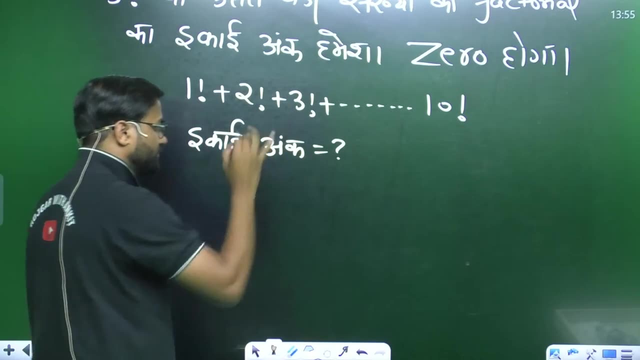 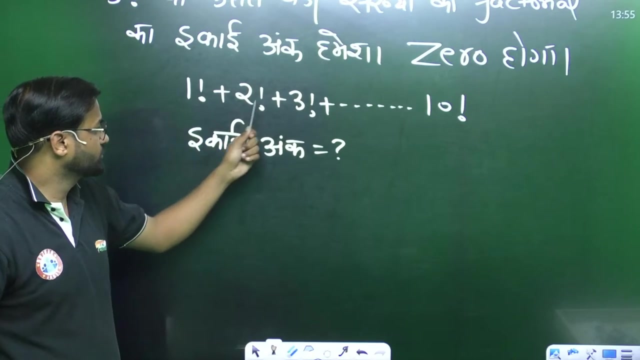 the number one What to do? tell me the number one. tell me the number one. tell me what will happen. Unit digit: what will happen? What will you do if you go by how you do this? if you have the question 1: factorial- 2 factorial, 3 factorial, And by doing that, the 10 factorial is 0 and the total x and PD is 30 on each side in its juncture. so this is 2 factorial, Let meűnủ it in this way- and then it is 21. so if you will come like this, that when you 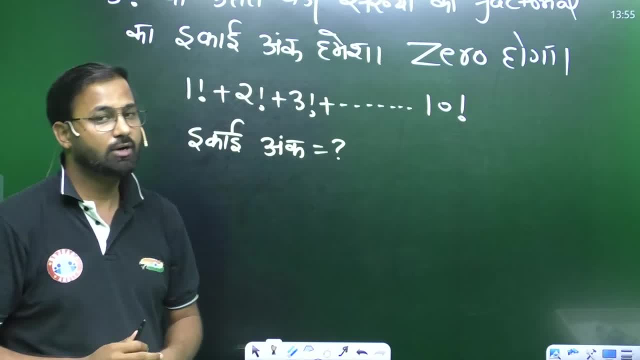 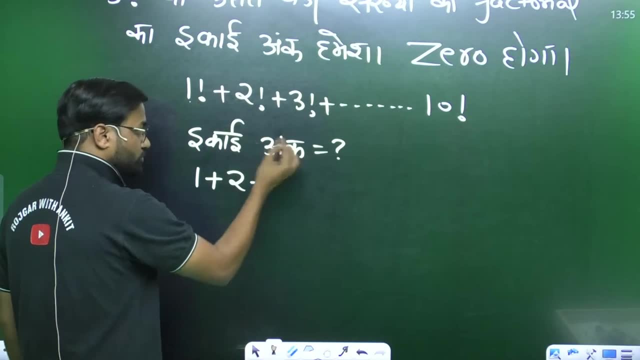 take zero and p and it will stay the volunt alert. the class number is 2 factorial and the number, If things go up to 10 factorial. then what will be your answer? 1 factorial means 1,. 2 factorial means 2, 2 times 1,. 3 factorial means 3 times 2 times 1,, 6,, 4 factorial means 24.. 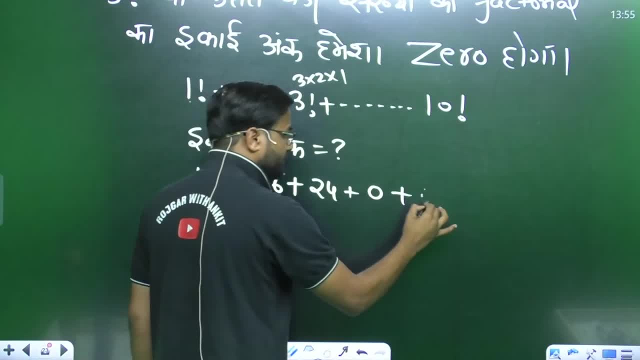 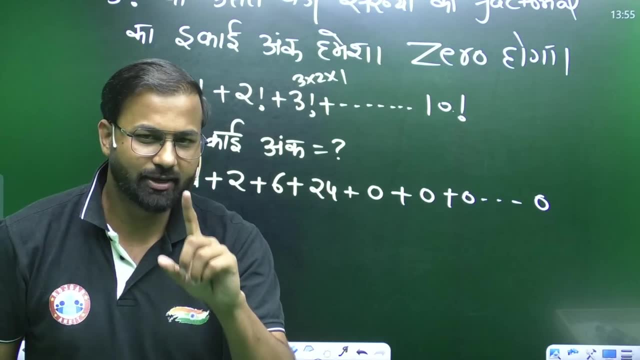 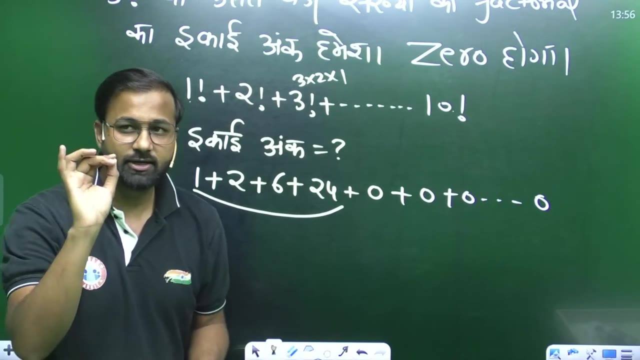 But as soon as 5 factorial comes, unit digit 0,, then 0,, then 0 and up to 10 factorial, unit digit 0 is going to be found. That means your work is only up to 4 factorial. How long? Only up to 4 factorial is your answer. 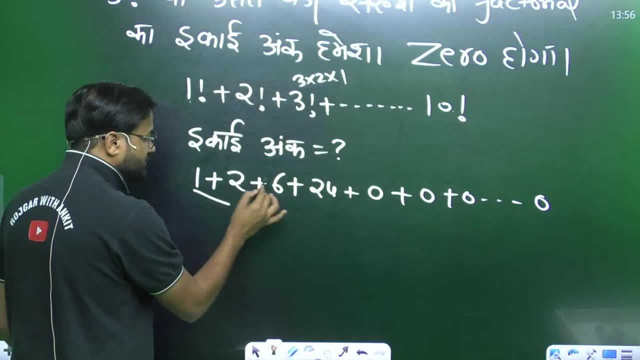 So when you add them, how much will it be? 2 and 1 is 3, 3 and 6 is 9, 9. is there right? Adding them is 9, 9 is added to 4, 13.. 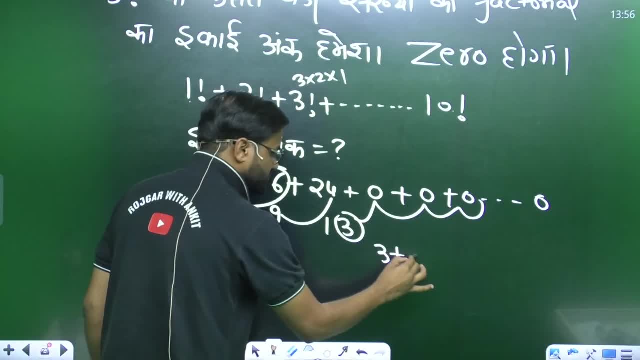 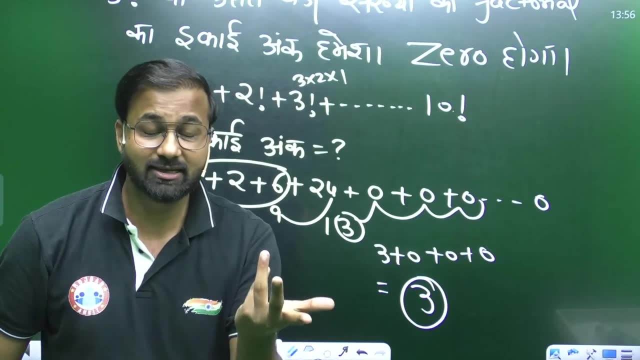 And then if you add 3 to any number- 3 plus 0 plus 0 plus 0, what will it make? It will make 3 only. Where are you getting the answer from 0?? There is no sign of quantity in between. 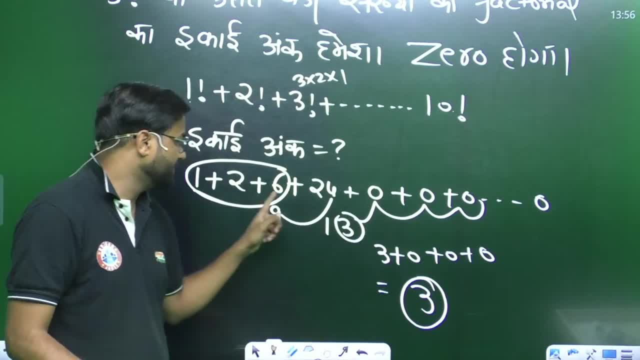 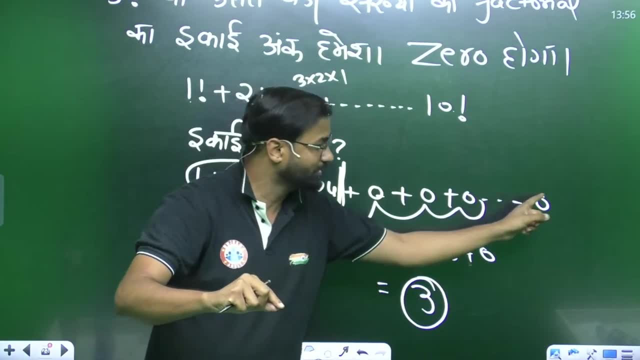 There is a sign of plus in between. So here you have added up to 4 factorial numbers. So unit digit is 3.. And then, in front of everyone, unit digit is 0, 0, 0, 0.. 5 factorial: is the number of factorial greater than that? 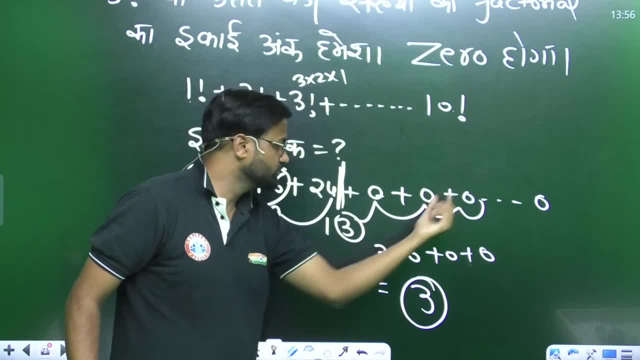 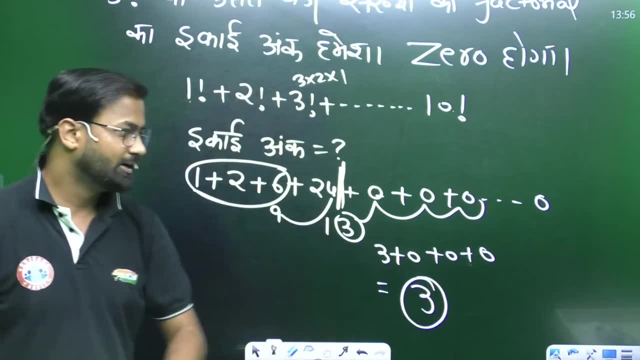 Unit digit is 0.. So, brother, 5 or greater than that 0, 0.. Add 0, 0, 0, 0 to 3, answer will be 3.. What will it be? You will get your answer. 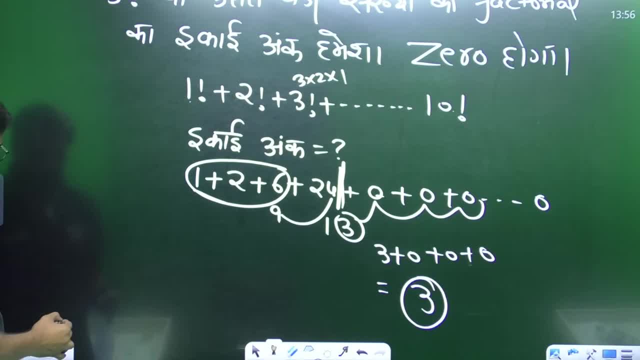 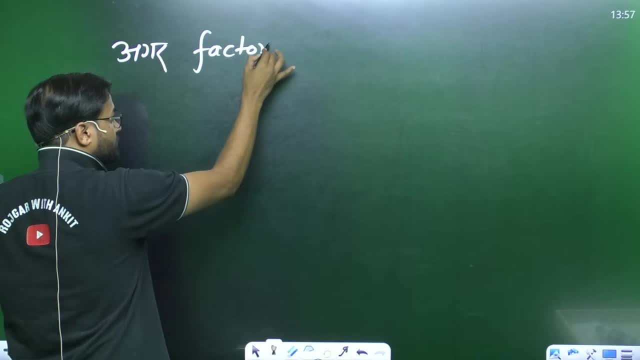 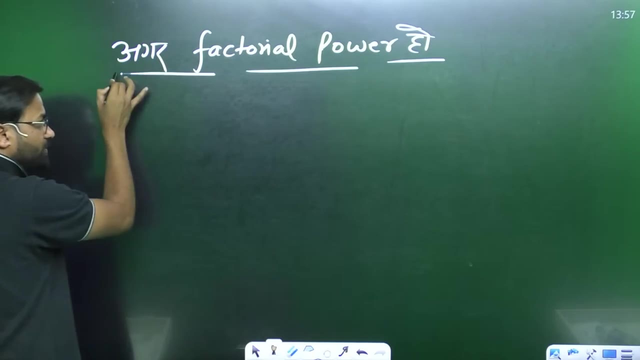 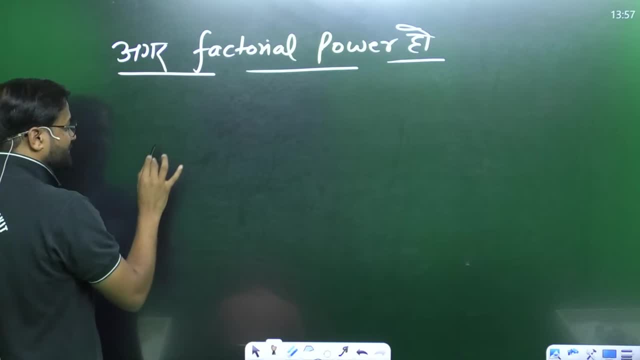 What to do. Just remember, As I said, Partial power is not factorial. I said 4 factorial. Power is of 3. power is 4 factorial. What is the unit digit of this? What will be its unit digit? Power of 3 is 4 factorial. 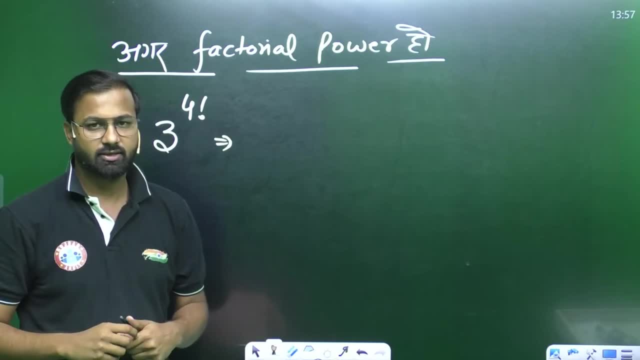 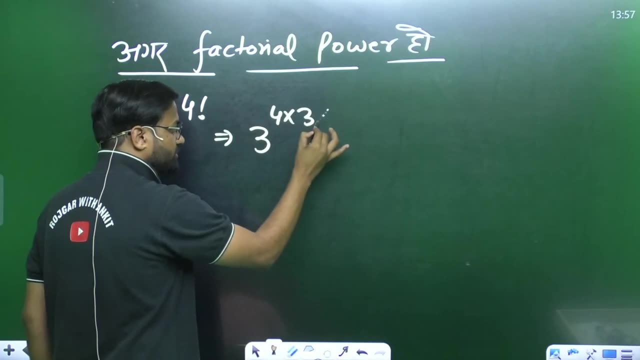 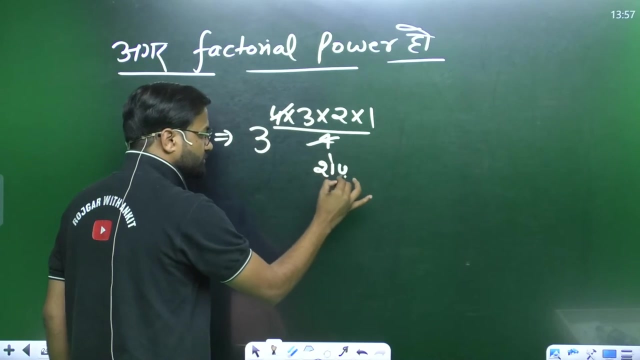 I said: let's divide the power by 4.. Let's divide the power by 4.. Don't want to divide it, but write it like this. I'm explaining: 3 x 2 x 1.. If you divide by 4, then the number will be completely cut off and the remainder will be 0.. 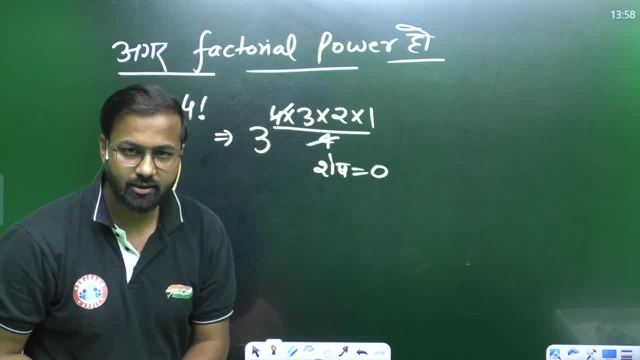 Brother, if the number below is completely cut off, then the final result is 0.. Isn't it? The final result is 0. And if 0 is the final result, then 3 to the power of 4 will be your answer. 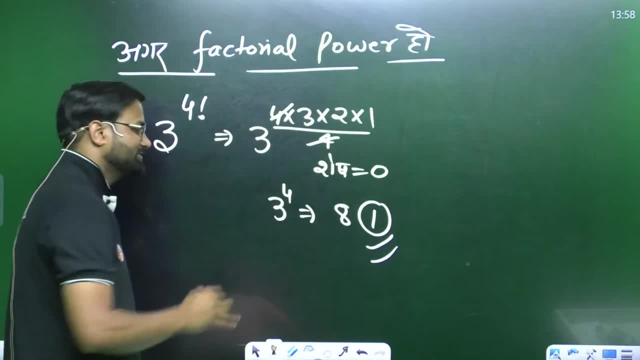 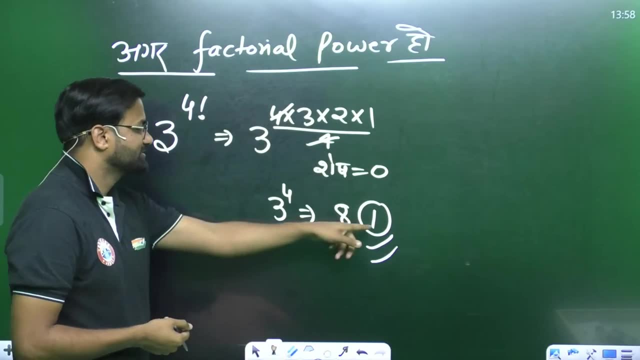 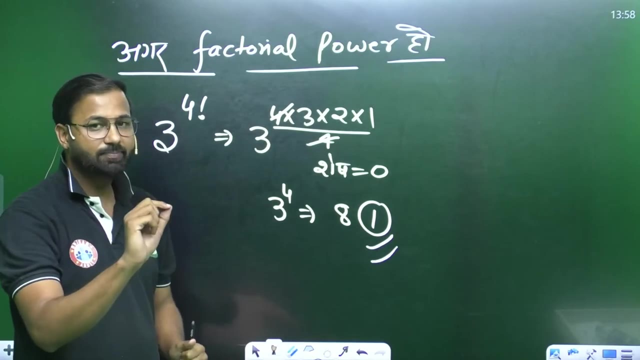 And 3 to the power of 4 is 81. So unit digit will be 1.. What will happen? Unit digit will be 1.. Absolutely correct answer. This is a very amazing concept. So here, what concept did I get? 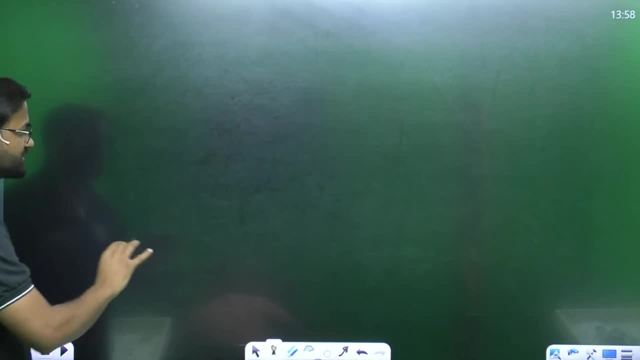 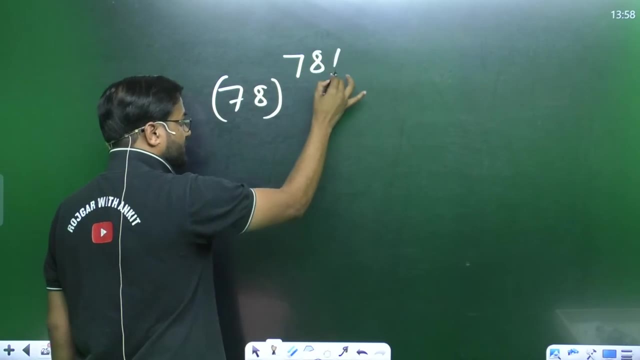 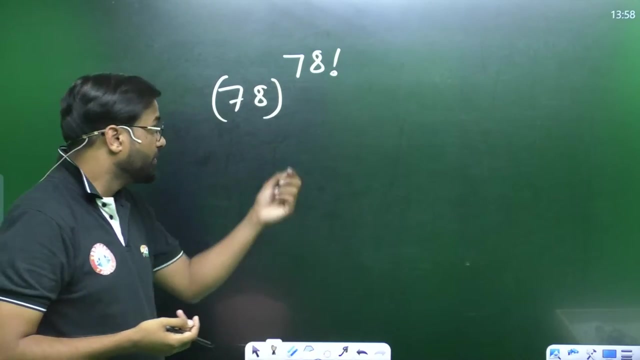 I will repeat it again with another example. I said that the power of 78 is 78 factorial. I said that the power of 78 is 78 factorial. Now, what should we do with this? I said that the power is divided by 4.. 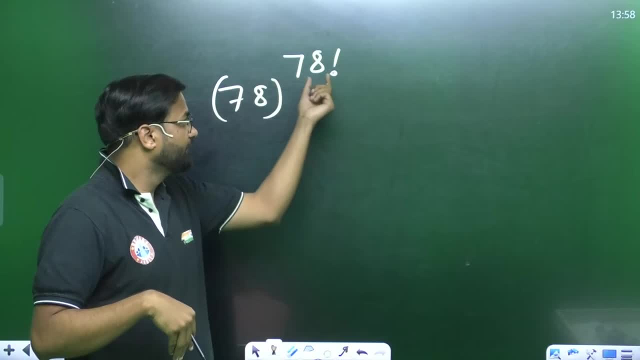 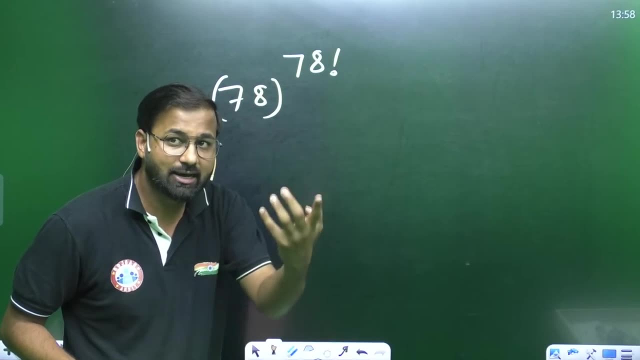 Don't worry, I will repeat it again. Don't worry at all. I said that the power is divided by 4.. The power is divided by 4.. But don't divide 78 by 4. Because it is factorial. So what will we do? 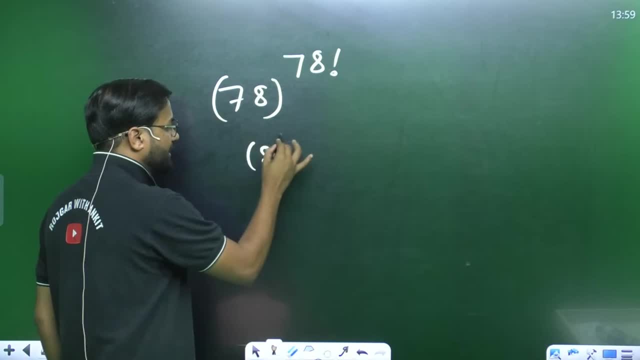 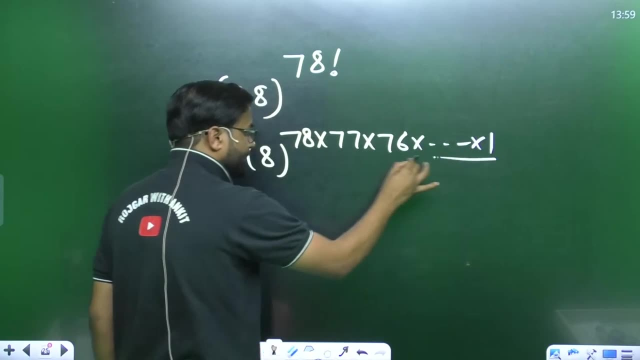 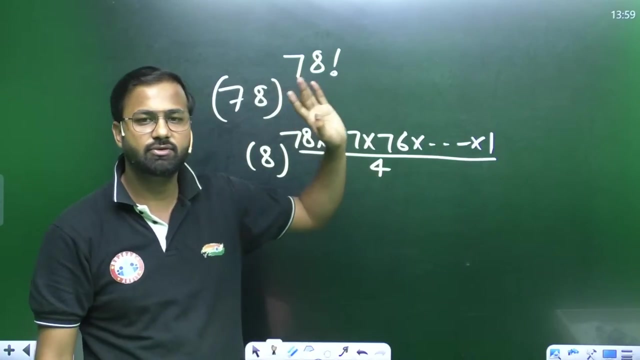 What is the power of 8?? 78 times, 77 times, 76 times, And by doing this it will come to 1.. Now, when you divide it by 4, then you will get a number which will be divided by 4.. 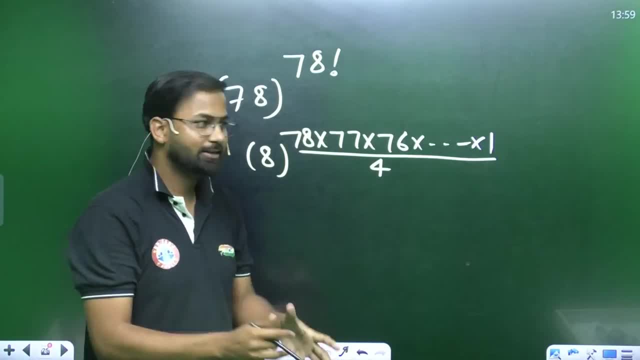 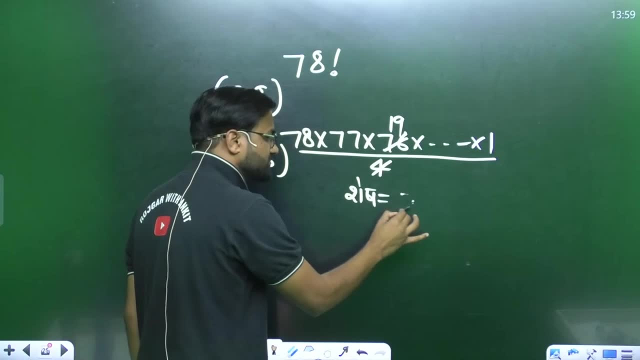 Now I will write the conclusion of this. What did the decision come out? If it is divided by 4, 19 times, then the final result is 0.. When the number below is cancelled, then the final result is 0.. So if the power of 8 is 0,, then it is 4.. 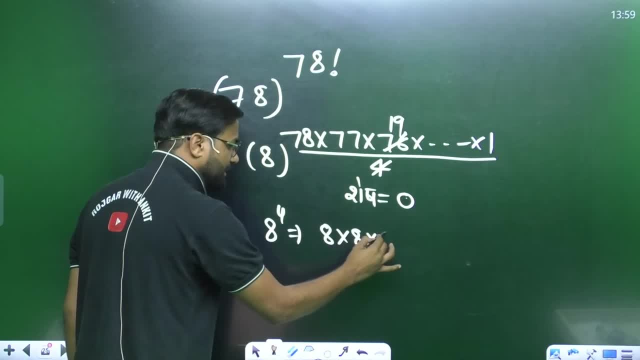 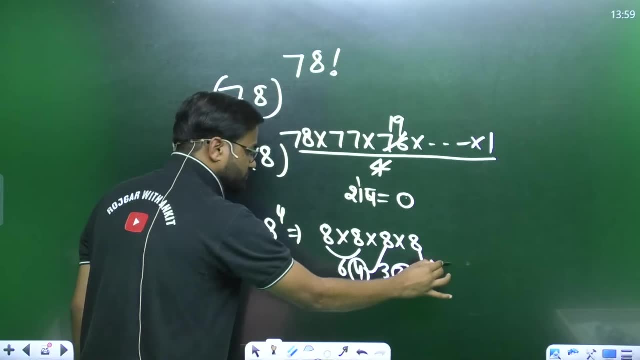 The power of 8 is 4 means 8 times 8 times 8 times 8.. 8 times 8 is 64.. Take 4.. 4 times 8 is 32.. Take 2.. 2 times 8 is 16.. 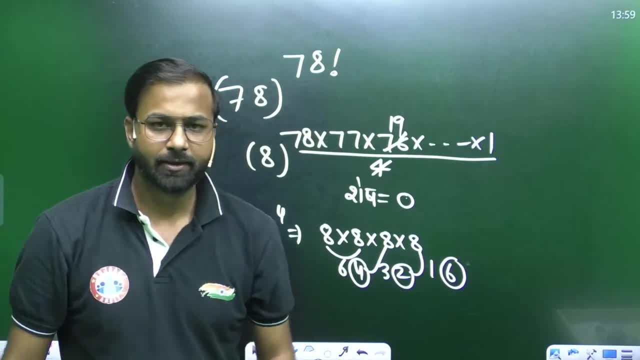 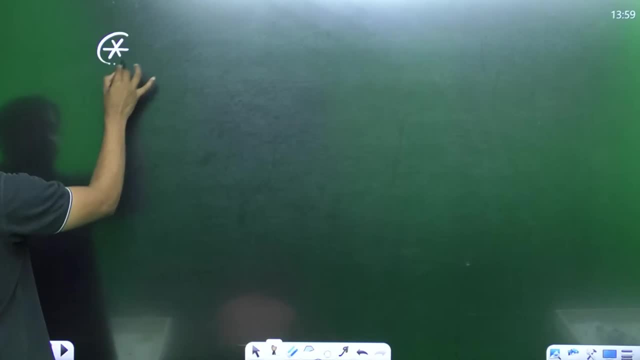 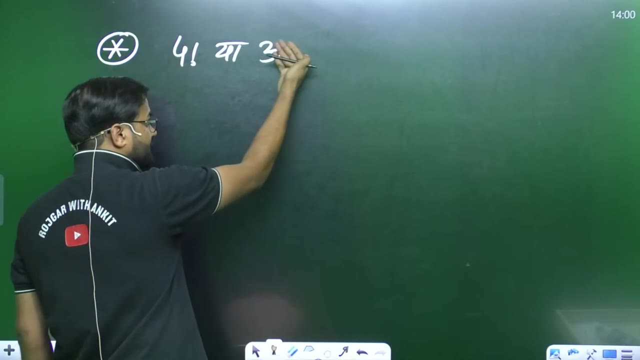 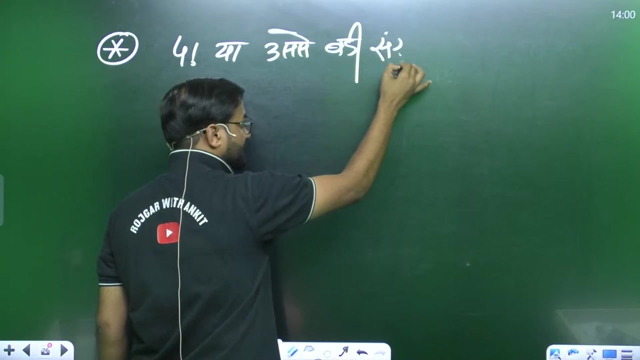 What is the unit digit? The unit digit is 6.. Now, what conclusion came out from here? The conclusion came out from here, The conclusion came out from here that factorial 4 factorial or greater than that, greater than that factorial greater than that. 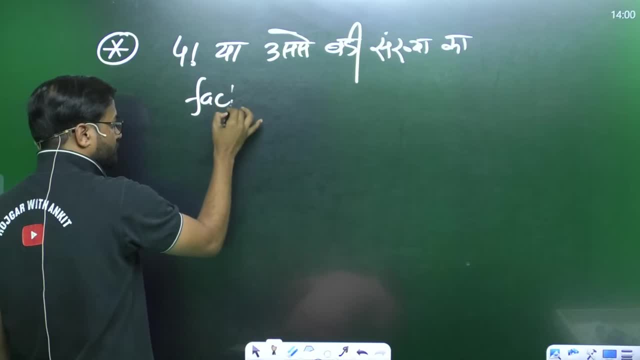 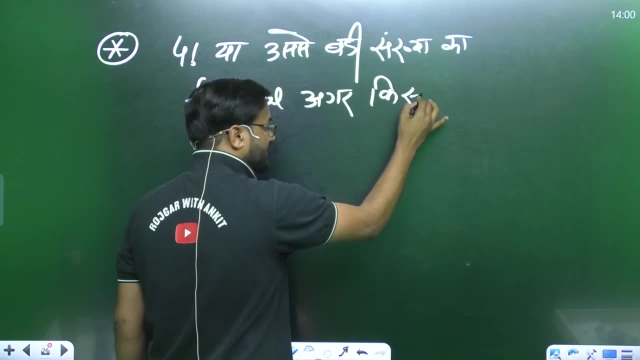 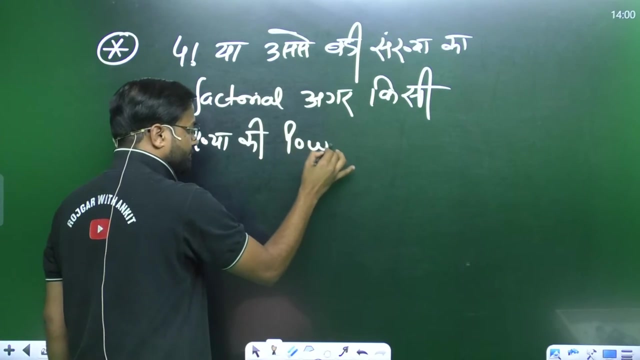 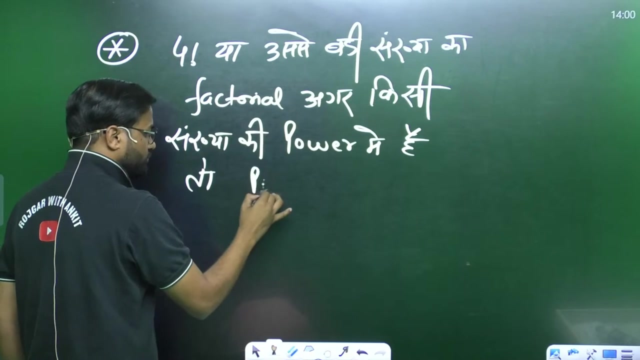 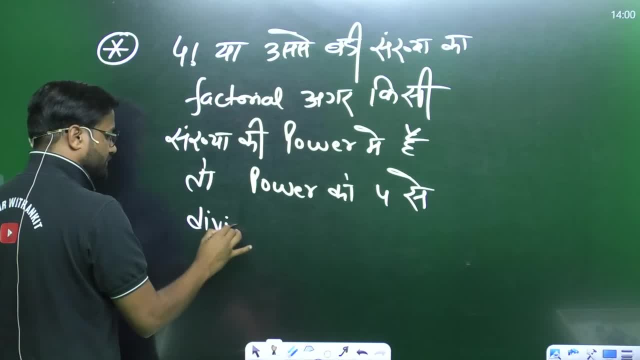 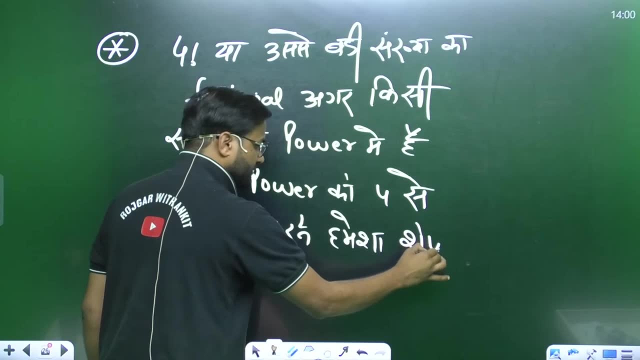 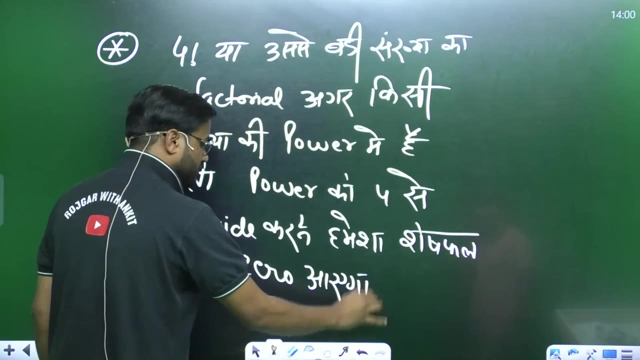 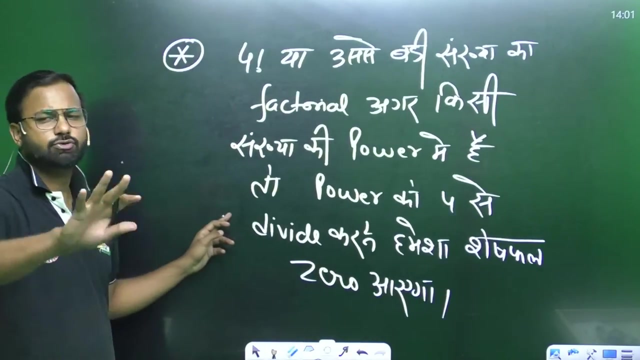 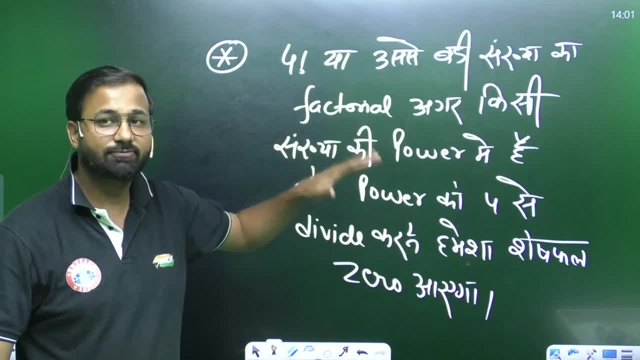 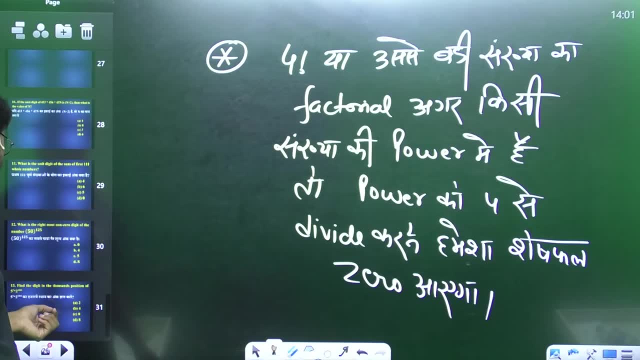 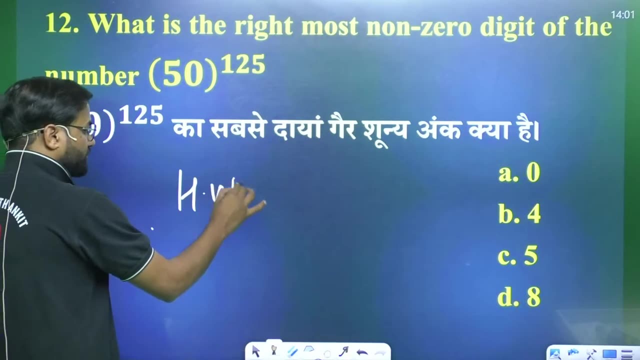